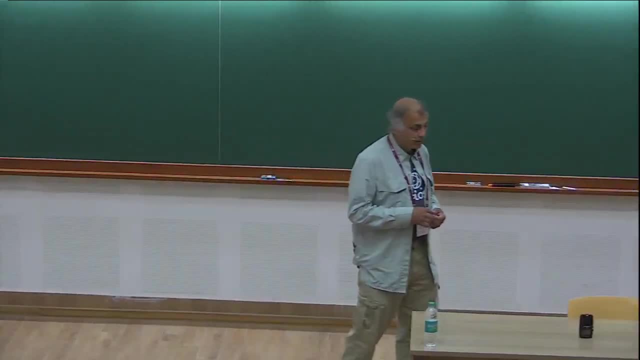 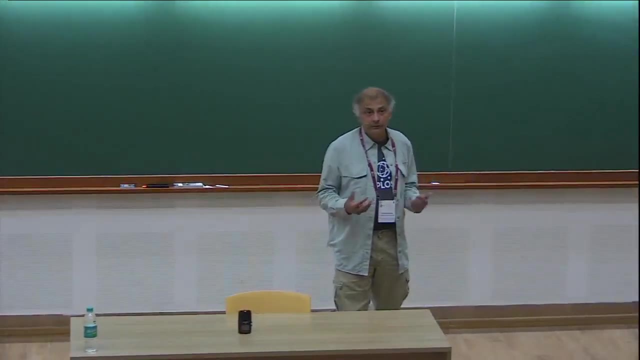 up to the individual who's giving it, But as for me, I would like to invite questions at any time. Just interrupt me with a question if you don't understand it, And I believe this should be the same for all the pedagogical talks. 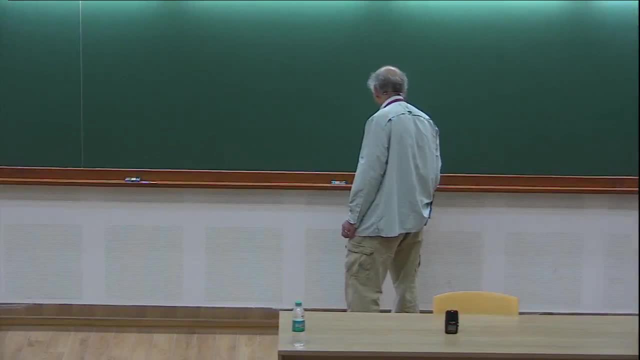 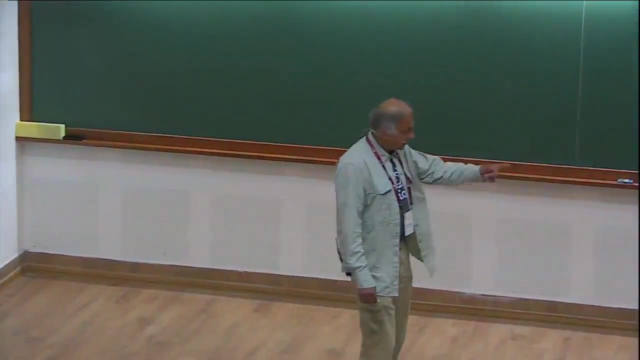 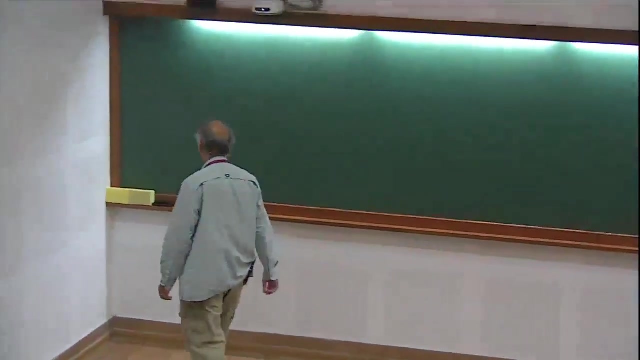 Okay, Good, Now I'm going to do this on the blackboard, So it's going to be recorded. I don't know if the – will the camera catch the blackboard completely? Okay, Good, All right, So I'll start with the classical Hall effect. 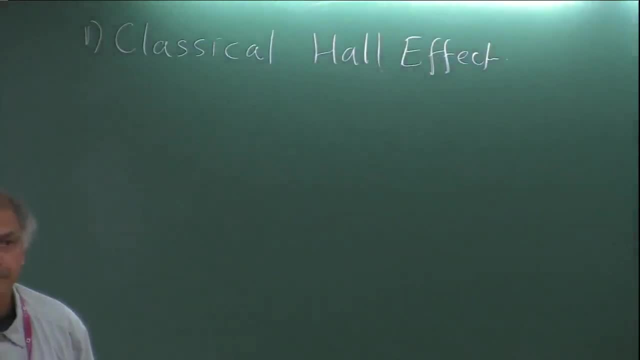 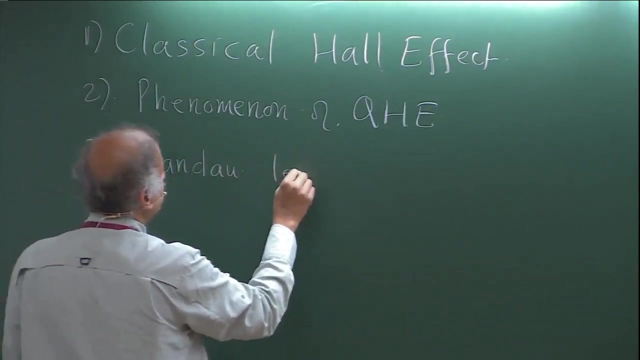 Is this big enough for people in the back to read? Yes, Okay. So then I will tell you what the phenomenon is of the quantum Hall effects. Then we'll talk about some elementary one-body Hamiltonian which will lead to Landau levels and their degeneracy, And then we'll 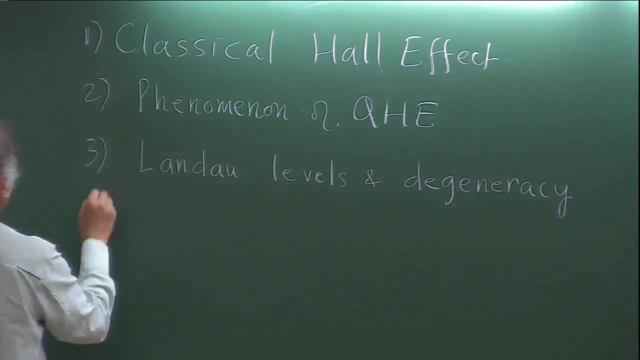 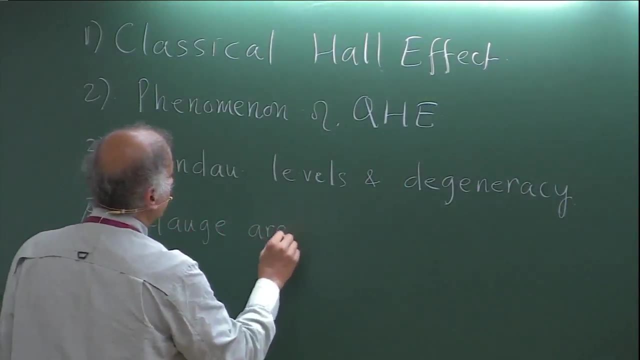 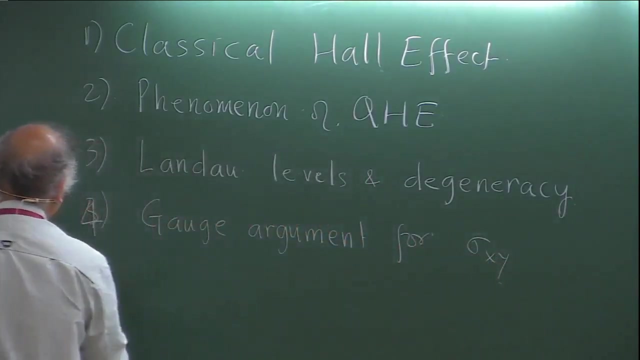 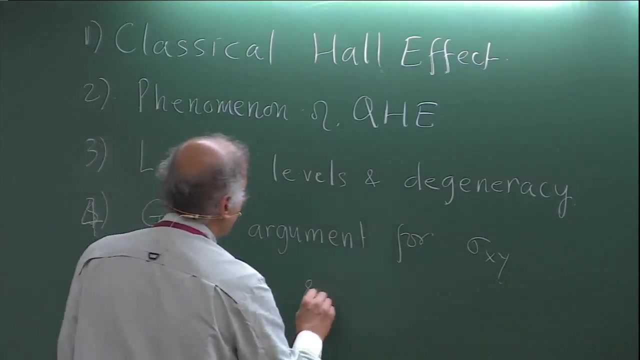 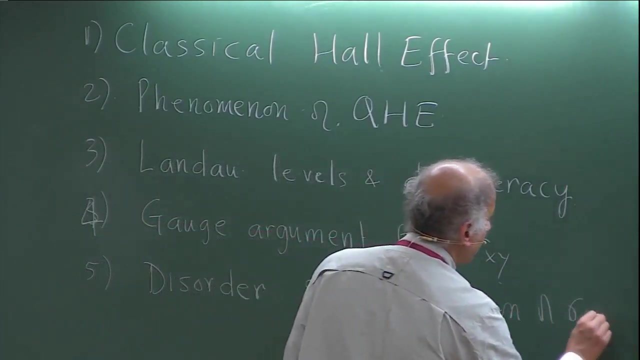 talk about what is known as the gauge argument, or sigma x- y, And then I'll talk about disorder, which actually plays a very crucial role, and how it actually quantizes. And then we'll talk about the sigma x- y And, since Shubhra has given me an extra five minutes, 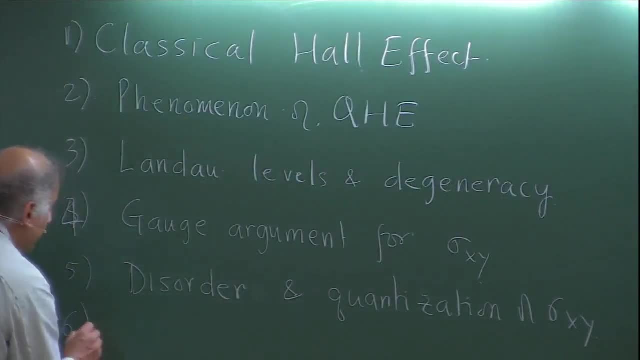 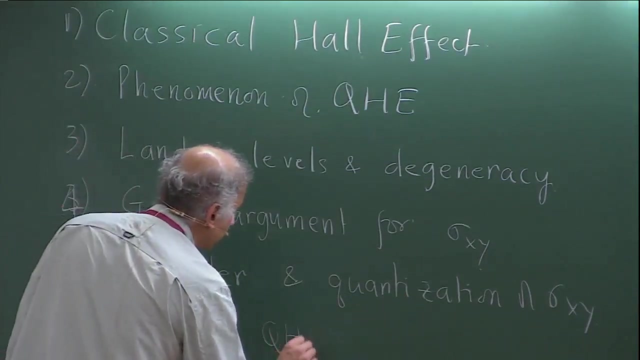 or ten minutes very kindly, if I have the time. there will be several talks on graphene. I believe in this conference And so, if I have the time towards the end, I will tell you a little bit about graphene, quantum Hall effect and how it differs from the standard. 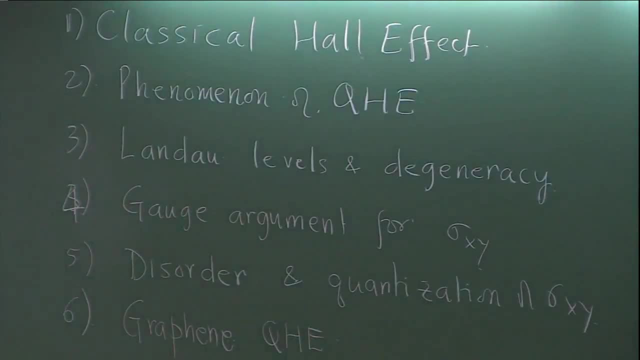 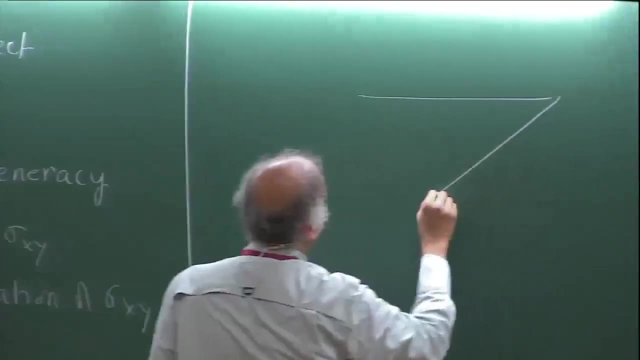 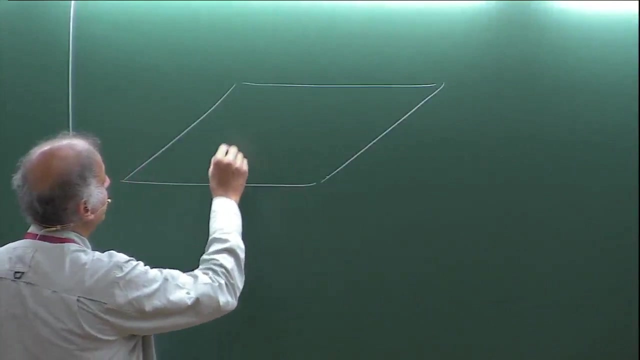 quantum Hall effect in semiconductors. Okay, So let's start with the classical Hall effect. Classical Hall effect was discovered around 1881 or something like that- 1880. And it consists of the following: So you have a perpendicular magnetic field. that's going. 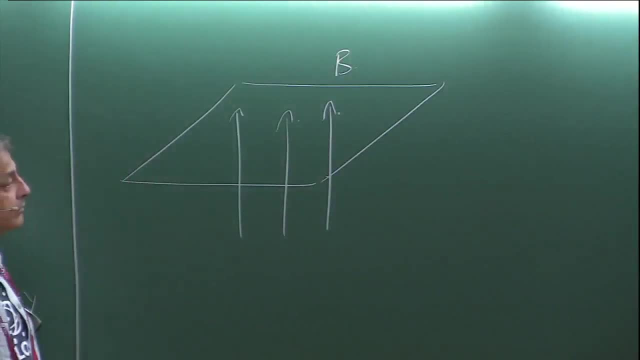 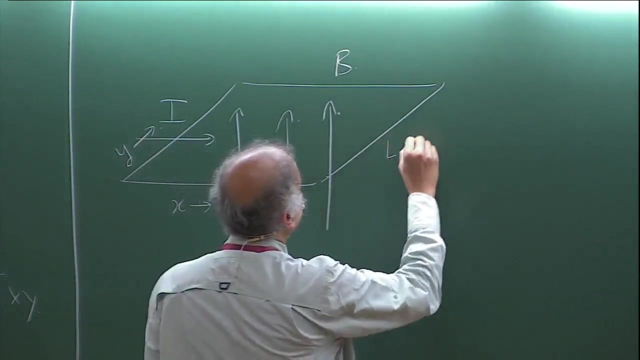 out of the plane. There's a two-dimensional plane or two-dimensional conductor. You push a current through it by using a current source that goes in this way. Let's call this direction Y. In the Y direction, the width of that sample is L sub Y And what is observed is: 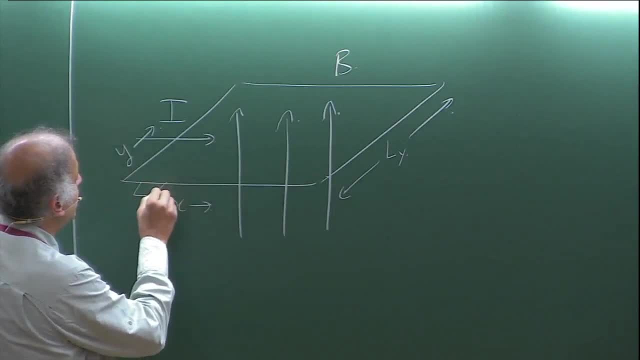 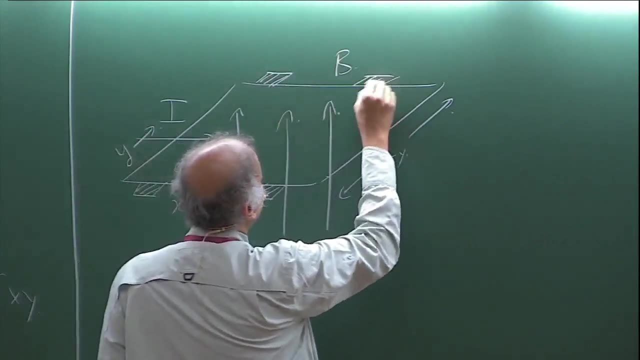 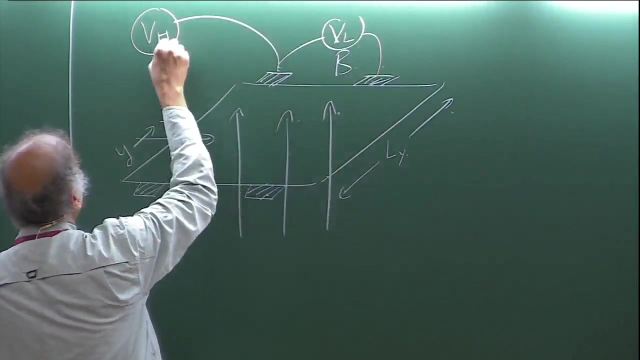 that, in addition to the usual longitudinal voltage that you would measure for any conductor, these are some contacts, So you can measure a longitudinal voltage here and you can measure a transverse, or nowadays what is called a Hall voltage over there across the sample. 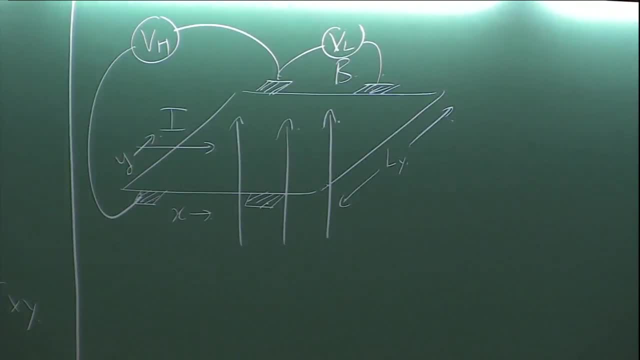 And so the current is in the x direction, the longitudinal voltage is also in the x direction and the Hall voltage is in the y direction. So let's imagine that this current is being carried out, carried by carriers of charge Q. So what is going to happen? 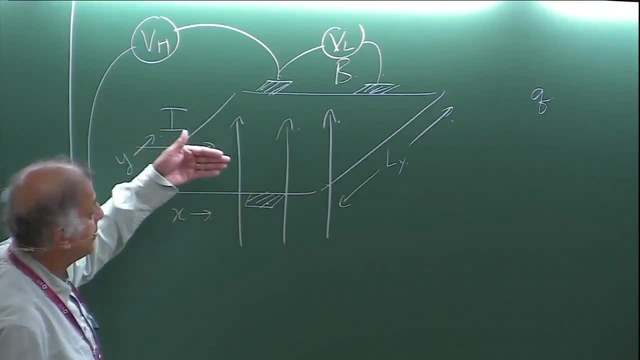 If Q is positive, then of course the charges are going to be moving in the same direction as the current. If Q is negative, they're going to be moving in the opposite direction. All right, So imagine that you have a positive charge here. 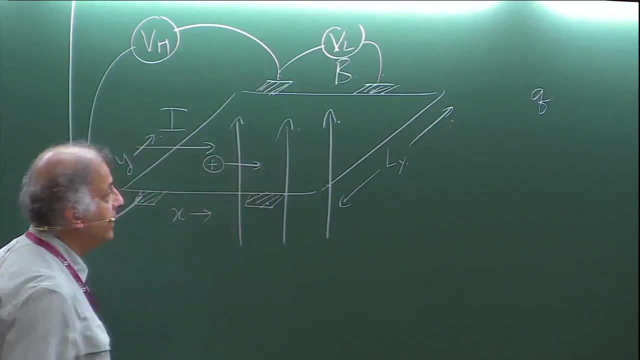 carrying this current. It's going this way and as it enters the field region, then it's going to get bent by the Lorentz force due to the magnetic field. Okay, And as it is bent, so let us see what happens. 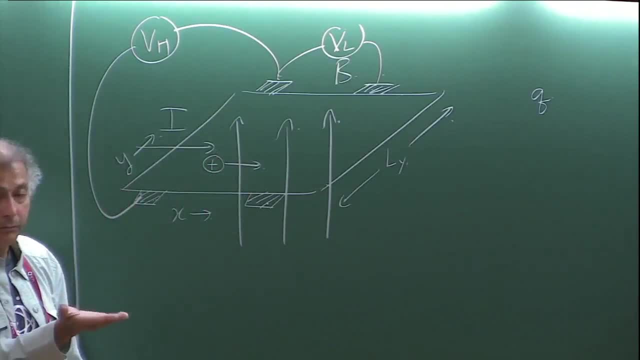 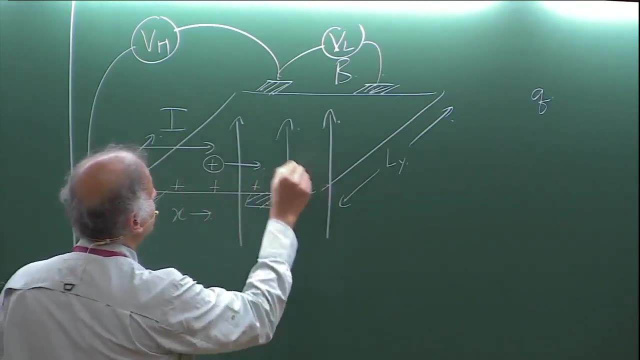 So there's Q, there's V. V is in this direction, B is in that direction, so it's going to get pushed towards my side of the sample, So it's going to accumulate over here. There are positive charges here. there are opposite, negative charges on the other side. 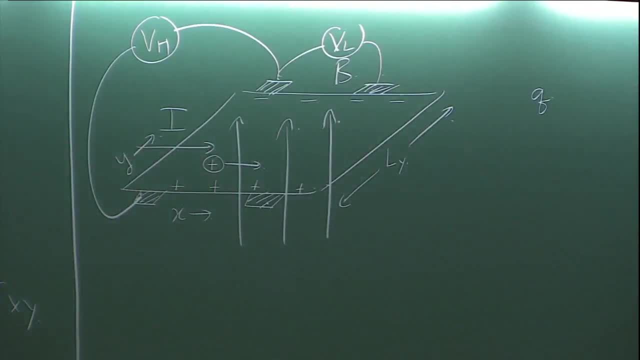 and that means there's an electric field that is being set up in the direction. thus, Okay, So there's going to be some E field here that's in the Y direction, And, of course, now that there's an E field, the charges that are moving through the sample will feed both the magnetic field. 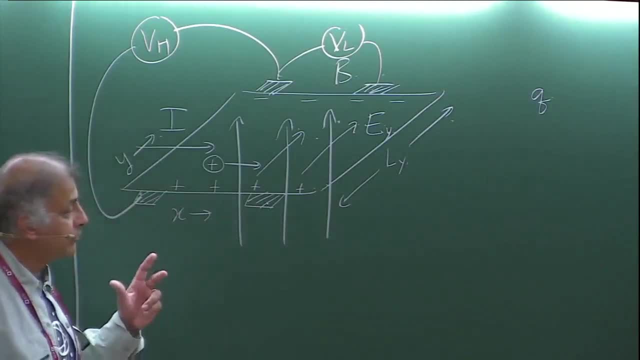 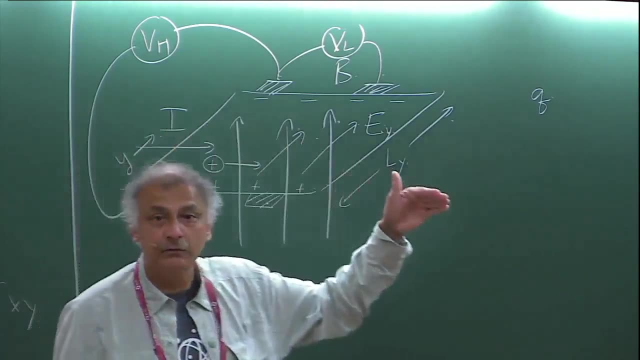 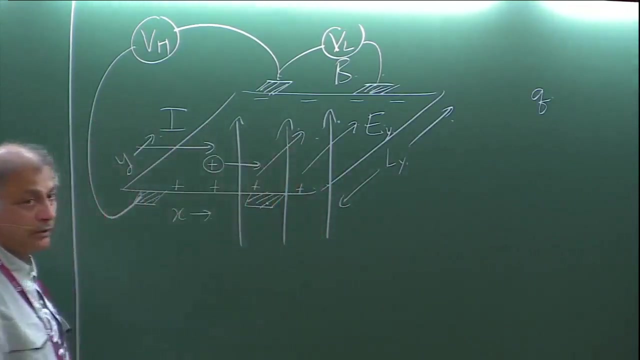 and the force due to the electric field, And this will continue to occur until there's a self-consistent solution such that the electrons can propagate- or sorry, the charges can propagate straight through without being deflected. All right. When that happens, the condition should be that whatever charge is moving through here, 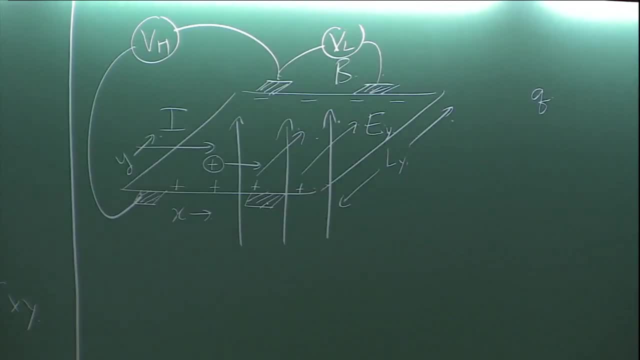 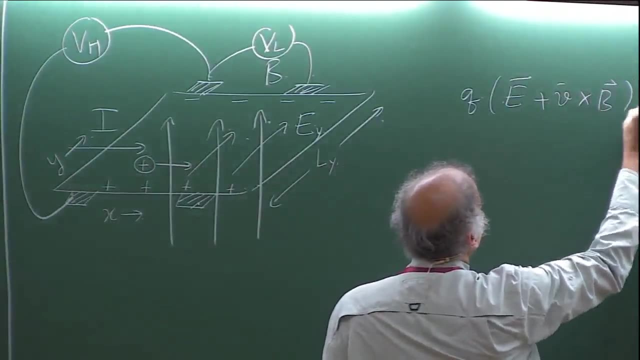 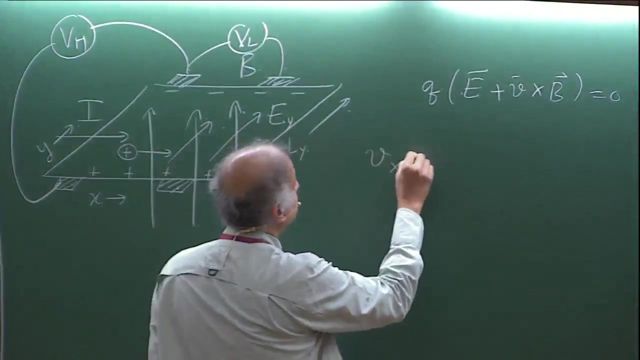 the electric and magnetic forces on it should cancel. And so that just says that Q times E plus V cross B should be zero Right. And that tells you that in this case the velocity in the X direction should be equal to E over B. 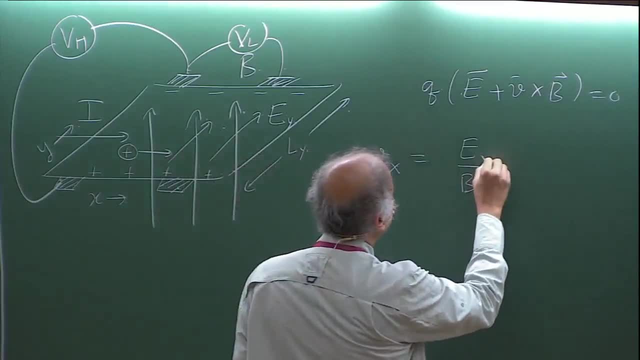 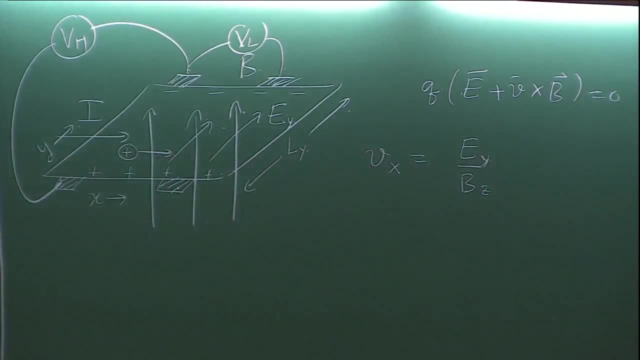 Right, So rather EY Over BZ in this particular case, Right, That is the condition under which those forces will cancel each other to some sign. Okay, So now let's try to figure out what this Hall voltage is actually going to be. 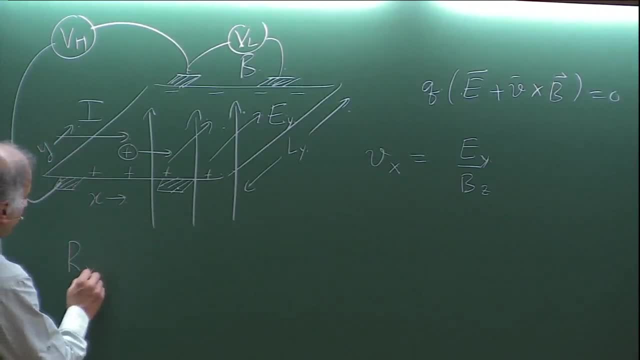 Okay, So what we want to measure, or what the experimentalists measure, is something called the Hall resistance. Okay, So it's the V Hall divided by the current. Okay, So this current, what is the current? Let's try to figure it out. 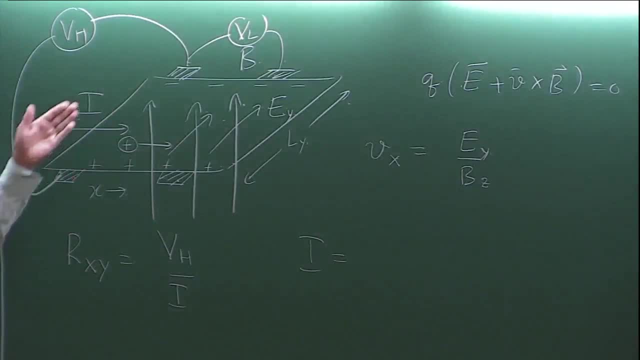 The current is the current density times the length in this direction. Right. This is a two-dimensional sheet current. So the total current is the current times the cross-sectional length in this two-dimensional sample. Okay, So that's going to be equal to JX times LY. 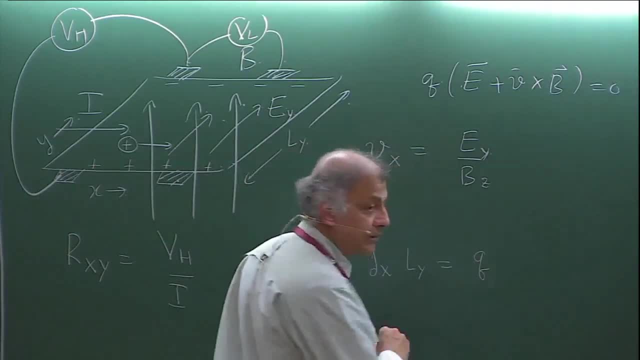 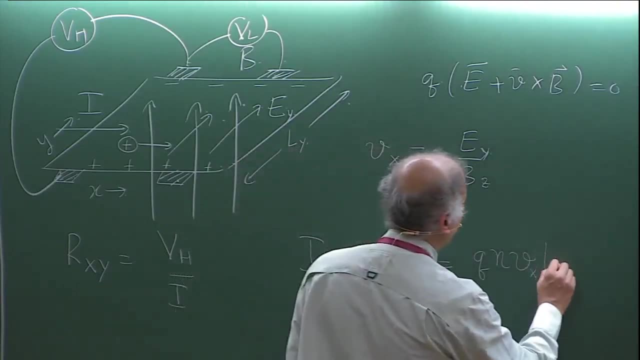 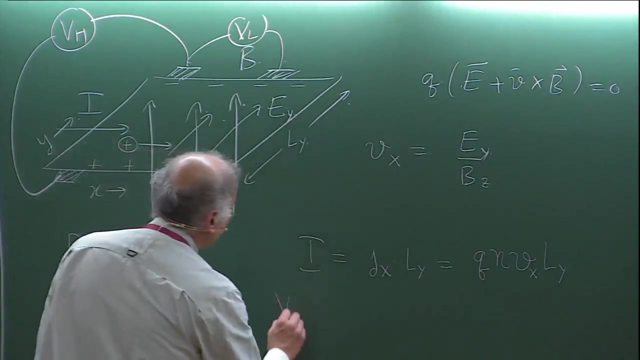 Right, And what is JX? It's the charge of the charge carriers times their density, times their drift velocity. Let me just call it VX times LY. Okay, Good, And then the Hall voltage is going to be equal to whatever is the electric field times LY. 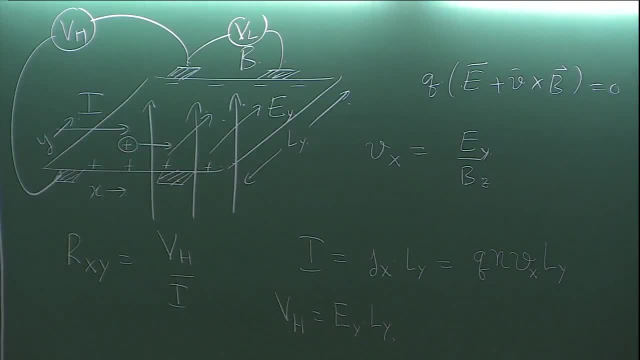 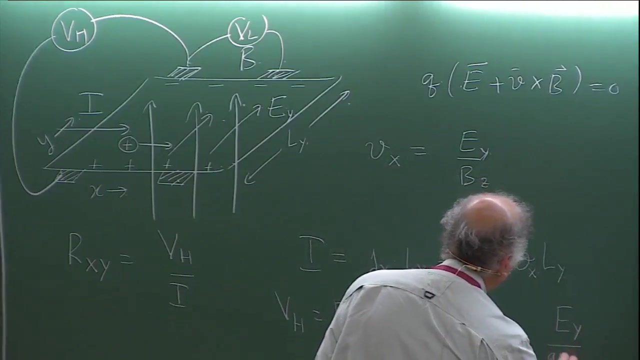 Right, All right. So therefore, the Hall resistance is going to come out as EY. The LY will cancel Right And then it will have QN, VX And, if I use the fact that VX is equal to EY over B. 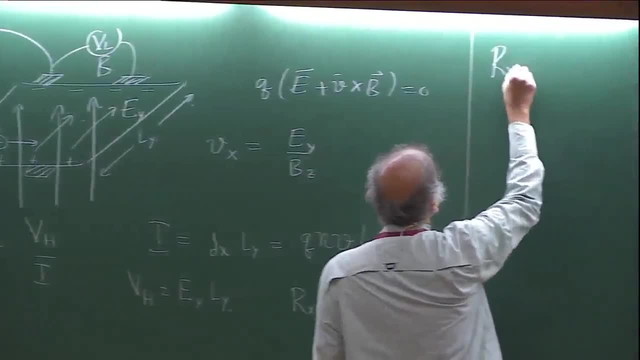 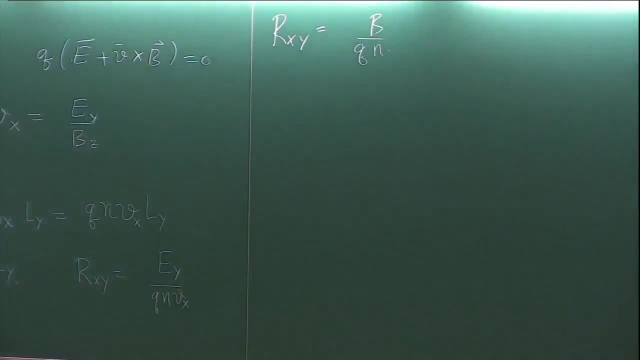 I find that RXY. Okay, That's what it is. So that is the Hall resistance. Now this, as I said, was observed already in the 1880s And even today it's actually used in any materials lab to characterize samples. 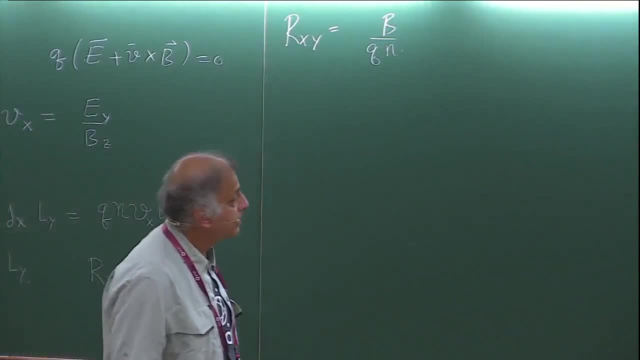 Okay, Okay, Okay, Okay. So one of the things you can do by measuring the Hall effect is to figure out what is the density of the carriers and what is the sign of the charge carriers. As you all probably know, sometimes in some materials it's not the electrons that are. 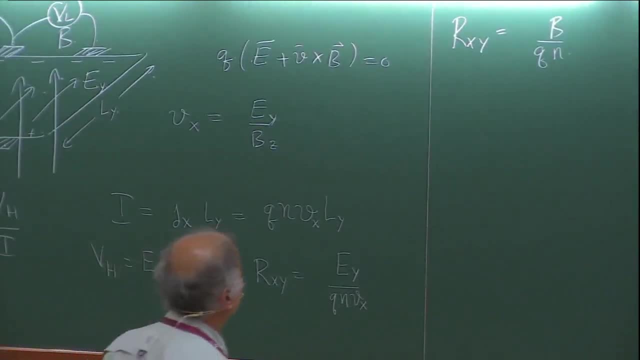 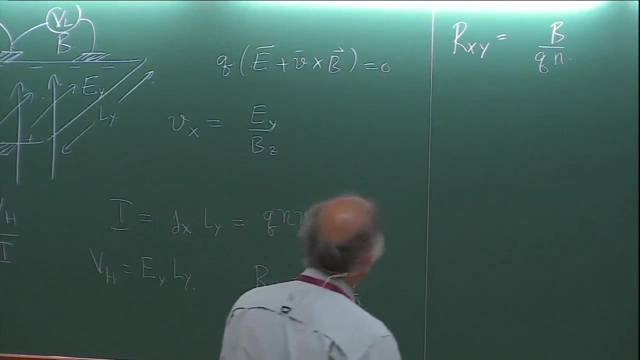 carrying charge, but it's the holes And they would come with a positive charge. So the sign of the Hall resistance indicates the sign of the charge carriers And the magnitude. from the magnitude you can actually extract what is the density of charge carriers. 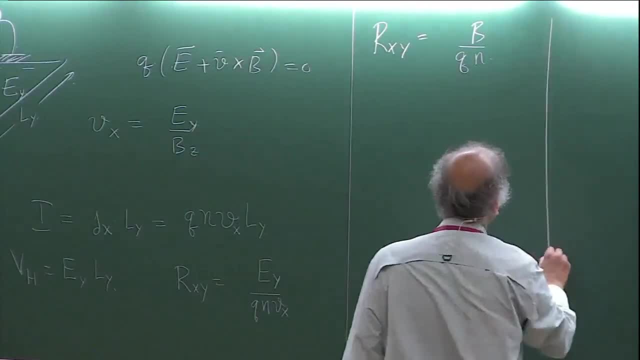 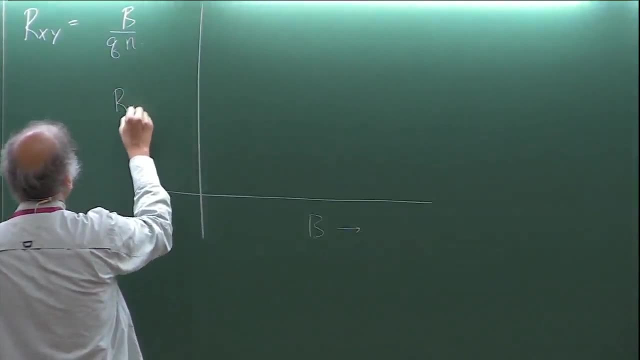 Okay So let me plot a graph. Let me plot a graph of what it ought to look like. Okay So, this is B in that direction and this is RXY. So what you should observe is something that looks like that, something that looks like: 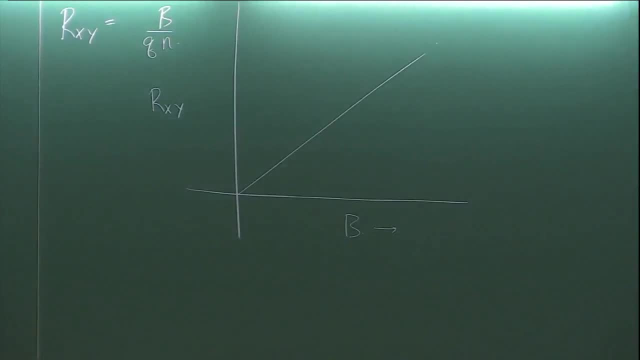 a straight line And the slope of that straight line will tell you the density of the charge carriers. Okay, Good, This is the classical Hall effect. Any questions? Okay, Is this all too elementary? Yes, You should say something, Otherwise, I've been known to ask, I've been known to point to particular people and ask: 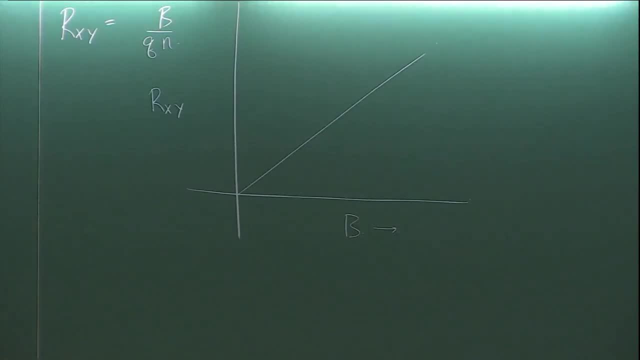 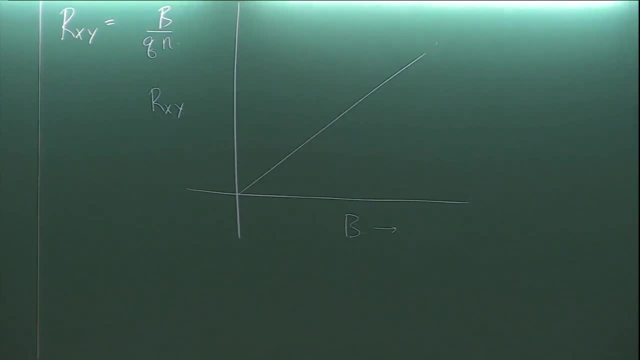 So even if the magnetic field were not present, there would still be an RXX that would come from scattering due to impurities inside this two-dimensional sheet. Okay, So any sample always has some impurities, some defects, some lattice defects and the 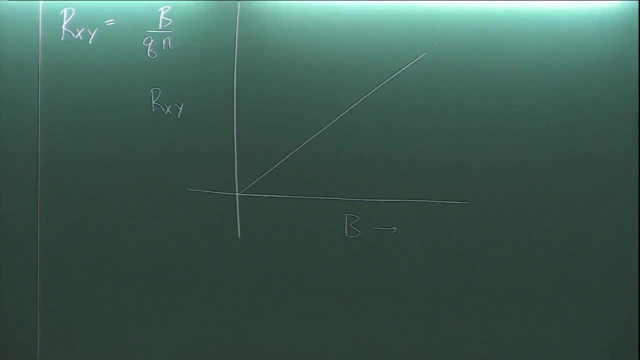 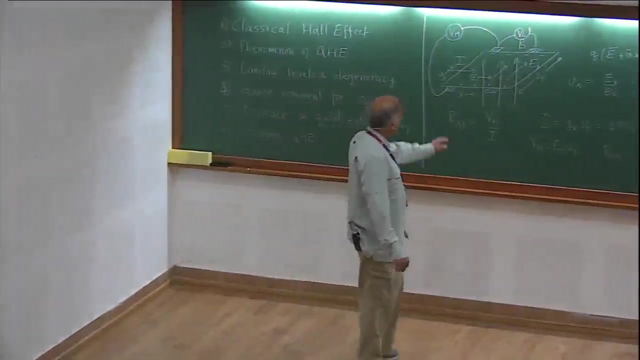 electrons as they're entering will scatter off of them And in addition to that, if you're at not a very low temperature, there will be photons and other things that can scatter electrons. Okay, So RXX comes from that, RXX in the presence of magnetic field, at the magnetic fields we are talking about. 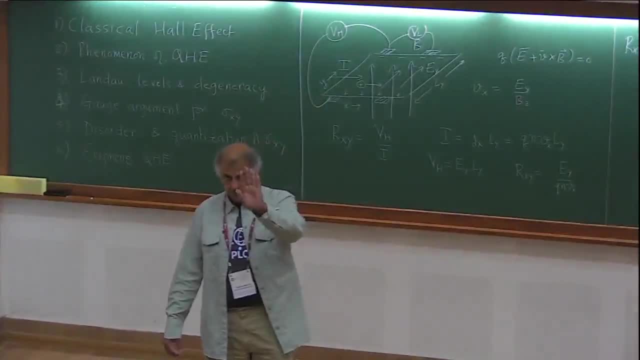 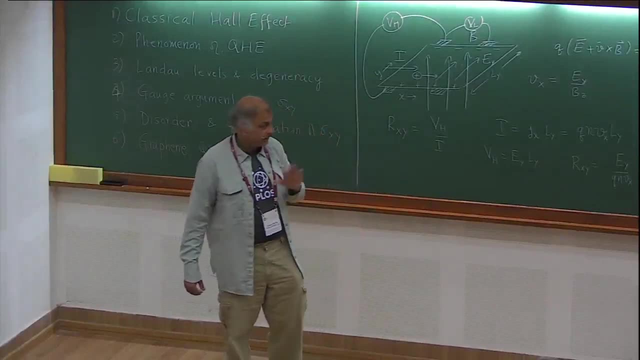 doesn't change very much. Okay, We will come shortly to the actual quantum Hall effects. So in the classical Hall effect RXX doesn't change very much The quantum Hall effect, it will change dramatically. We will see that shortly, Okay. 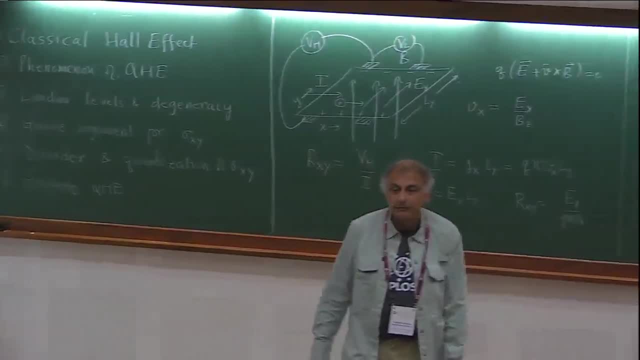 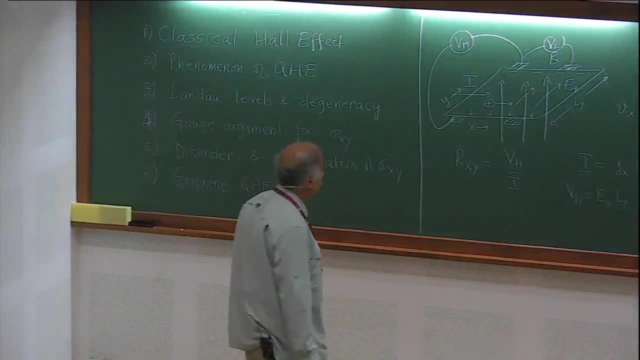 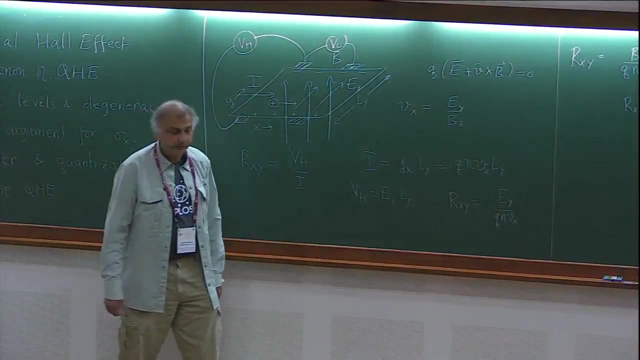 Other questions. Yeah, Yeah, I have a question. Very good, Very good. So the Galilean invariance argument basically says that if you have an electric field and a magnetic field, if the electric field is smaller than the magnetic field, you can boost. 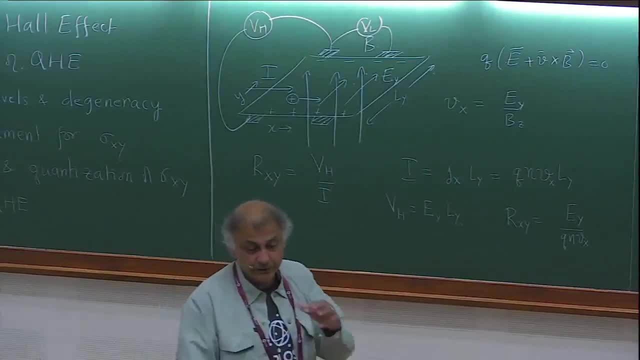 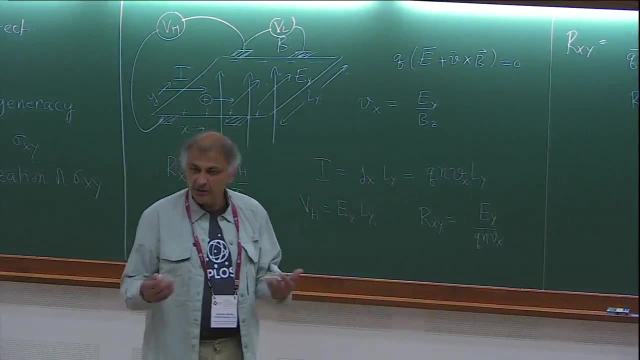 yourself into a frame in which, due to the transformation of electric and magnetic fields into each other, you can actually cancel the electric field completely, Right? So that is the- It's actually Lorentz invariance, but at very low velocities it becomes Galilean. 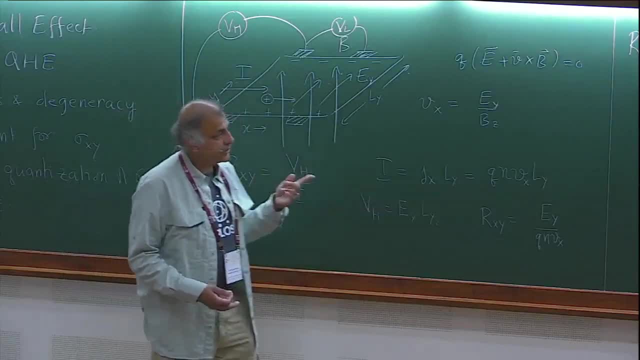 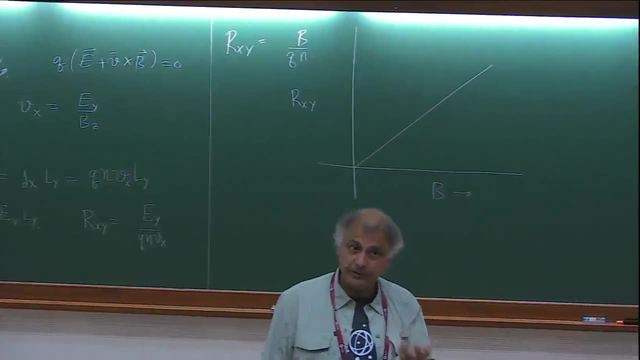 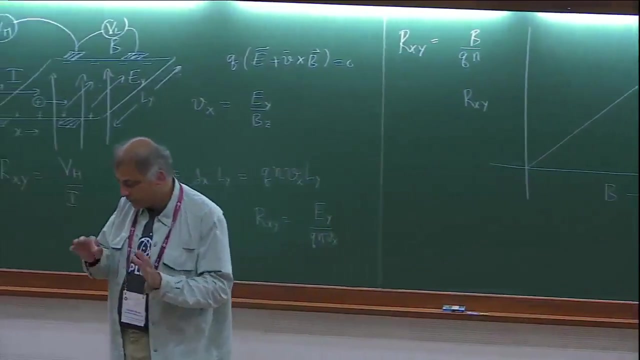 invariance. So that will basically say that this curve should hold at all temperatures As long as there is no disorder in the sample. Okay, But there is always disorder in the sample, So that situation is never realized, Okay, So it's a very theoretical argument which, however, will play some role. 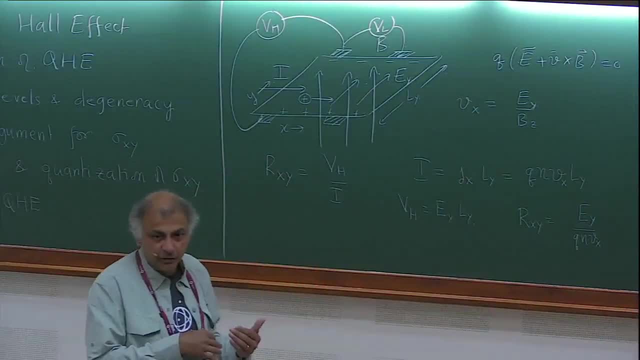 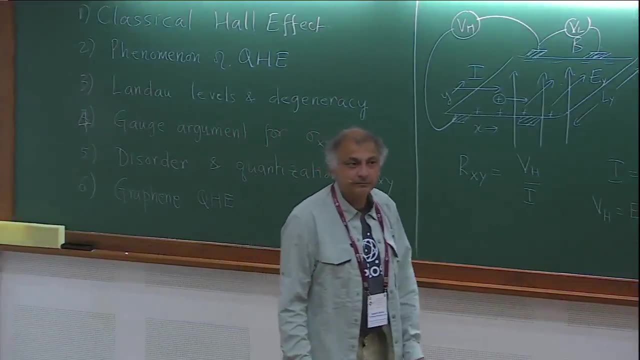 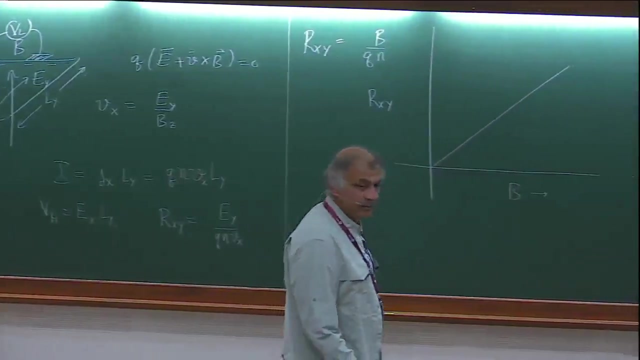 So it shows you that if you didn't have disorder, you would actually not have the quantum Hall effects. Okay, You would not have the quantization of the Hall resistance. Okay, Other questions? Yeah, Sorry, speak up, speak up. 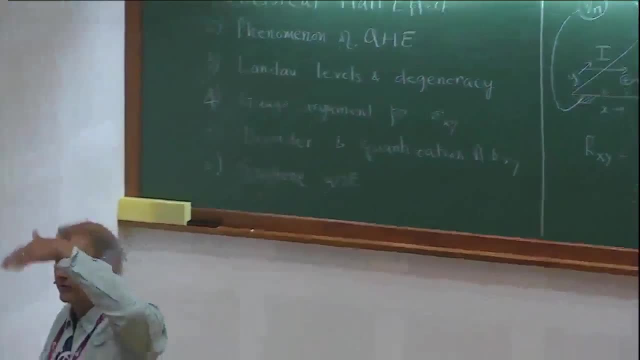 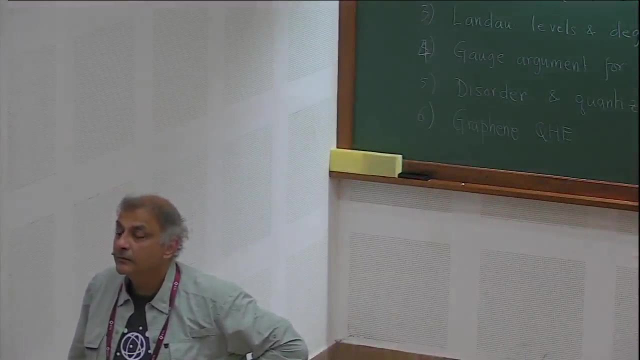 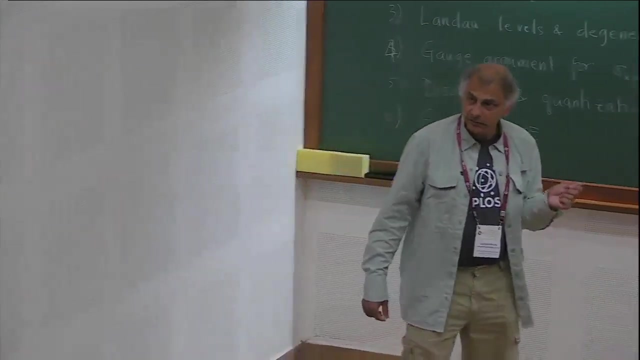 I can't hear very well, okay, So, especially if you're in the back, you should speak a little louder. Yeah Right, That is the steady state. Yeah, So when you switch on the current, there will be a transient. 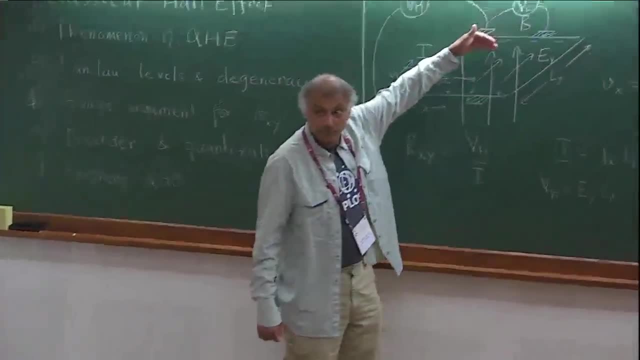 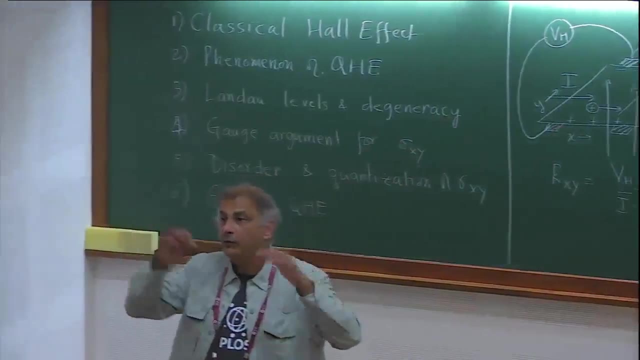 So before there was any current, of course there's no electric field. So when you switch on the current For I don't know some picoseconds, there will be some transient where the electric field will grow from zero to whatever value it will have in the steady state. 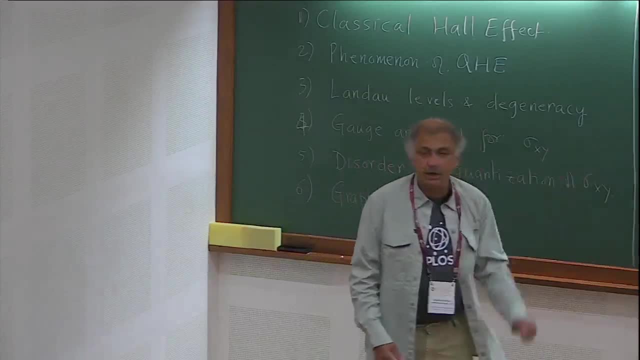 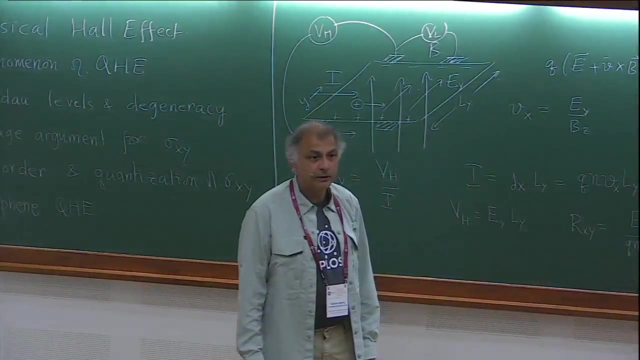 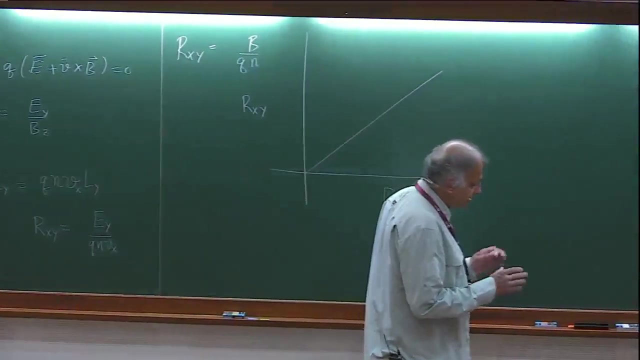 Okay, So after that transient, there will be a steady state, and this is the electric field in the steady state. All right, Good Shall we proceed. Okay, So now what happens is that this is indeed what's observed in almost any material at 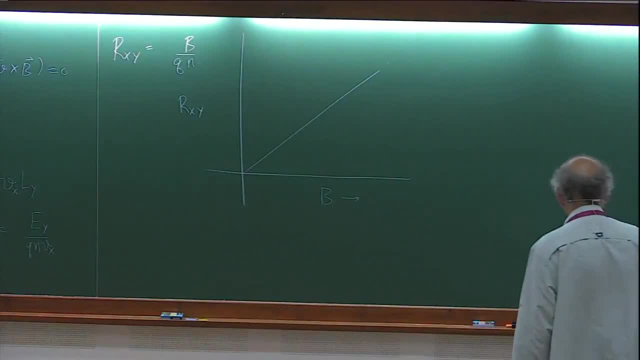 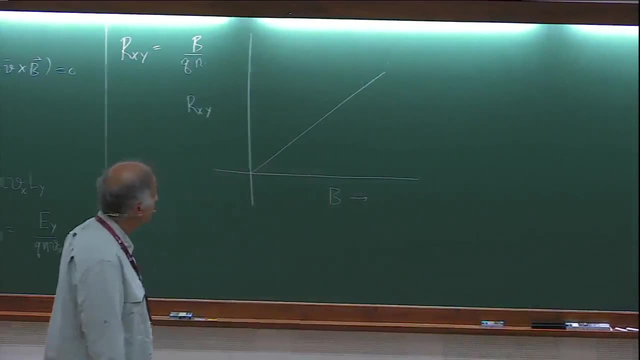 room temperature As you start cooling it and if the material is very clean. of course, no matter how clean you make it, there is always some disorder there, and that's essential. As you make the material very clean, it turns out that you start seeing the appearance of 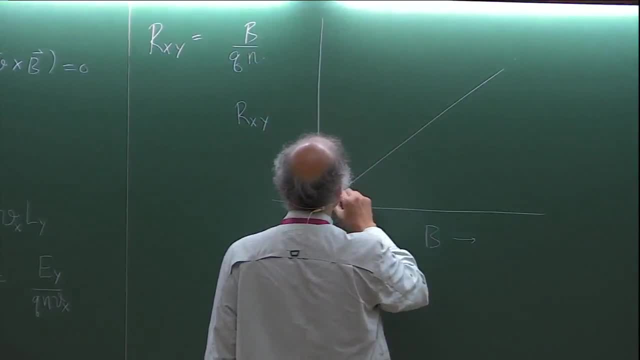 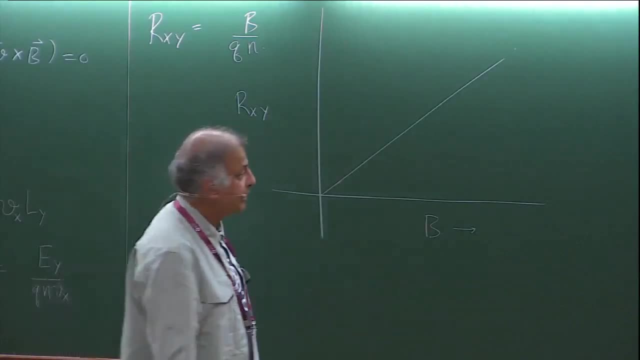 certain steps. Okay, So it first starts looking sort of like this. So it follows this line for a while, And now I'm going to draw a sequence of graphs at lower and lower temperatures. Okay, So this white graph was at room temperature. 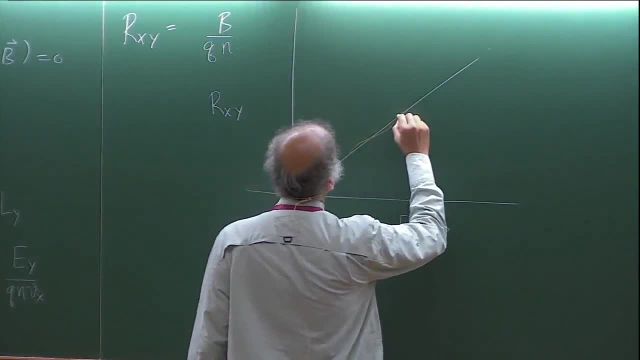 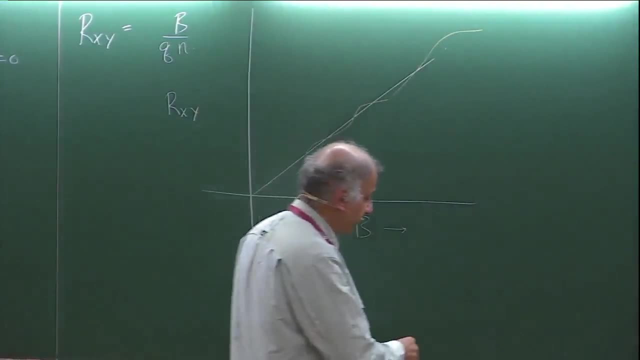 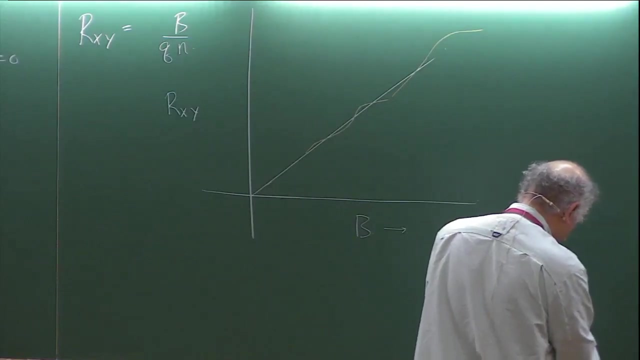 Okay, Then here comes another graph. This graph that's sort of at some other temperature, slightly lower, and so on. So it looks like this: At an even lower temperature, at an even lower temperature. what will happen is that this? 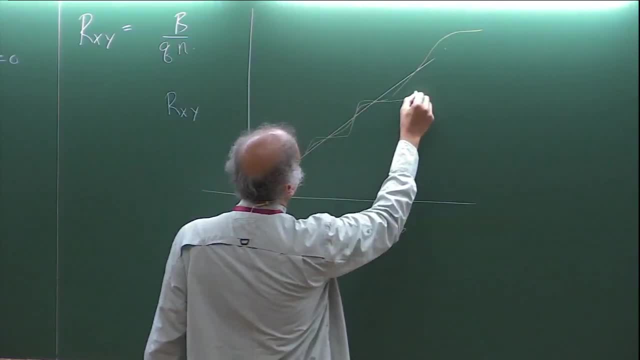 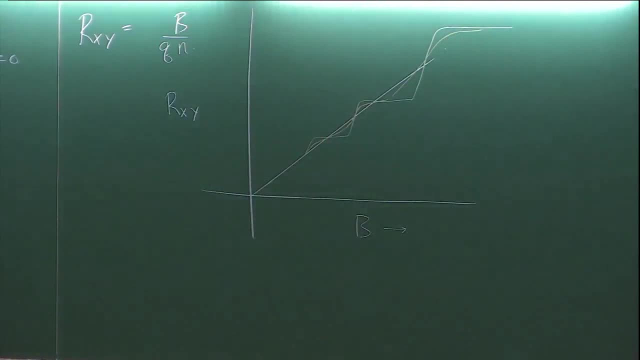 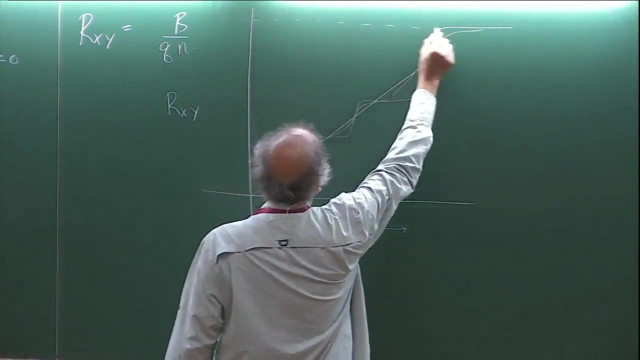 guy will sharpen, It will sharpen. And as the temperature keeps getting lower and lower, These steps, these plateaus, get sharper and sharper. Okay, Not only that, the value of the Hall resistance at these plateaus is always found to be or. 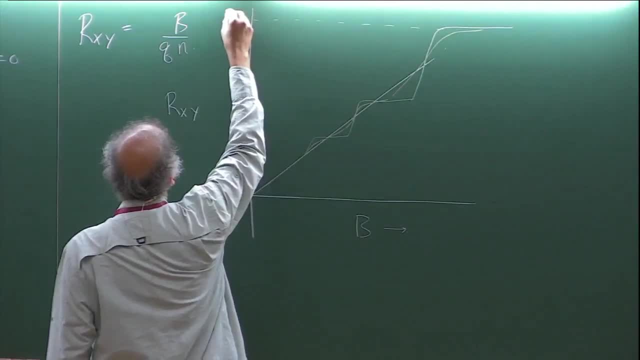 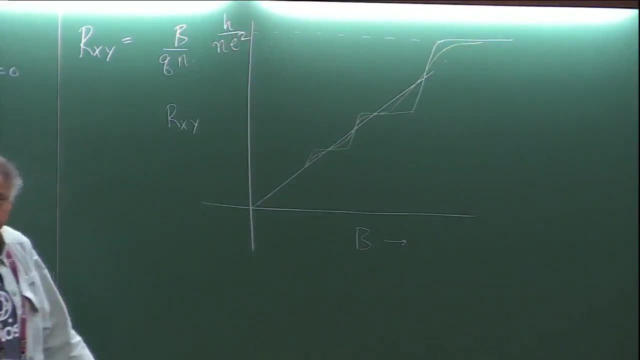 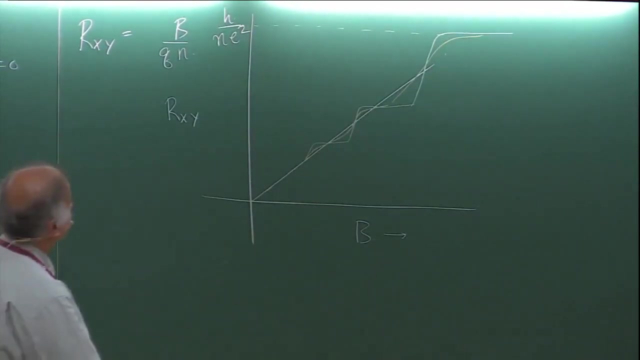 almost always, is found to be some. So H is Planck's constant, N is some integer, and then E is, of course, the electric charge. Okay, It's found to be this value. So let's say this is, I don't know- H over 1E squared. 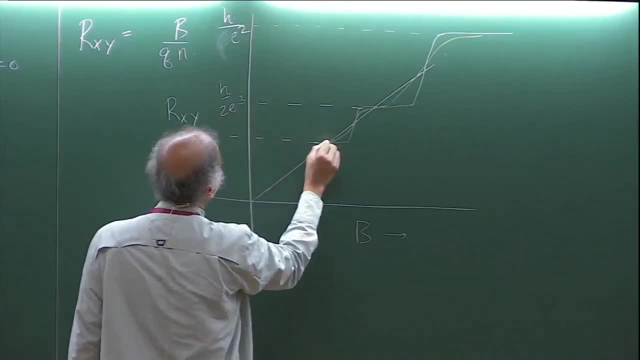 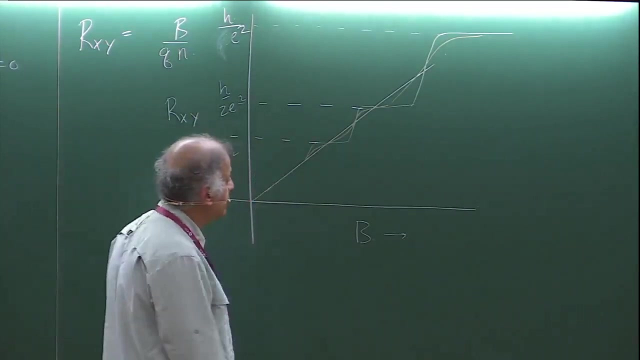 Maybe this is H over 2E squared, This is H over 3E squared, and so on. Okay, So this is the phenomenon. So now somebody asked me about Rxx. So Rxx also does a weird thing. So what happens is that as you start developing these plateaus, you also start seeing oscillations. 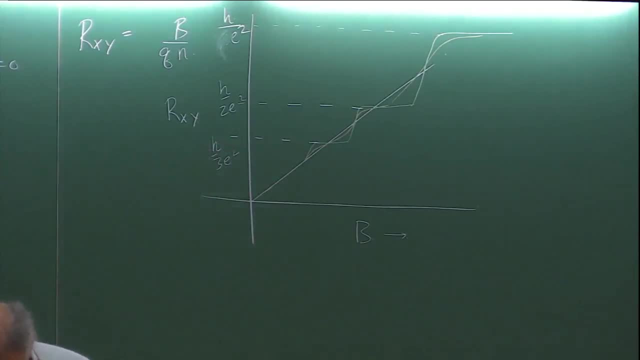 in Rxx. Okay, Now, some of you may have heard of Schublikov-Dehaas oscillations or Dehaas-Van Alphen oscillations or something like that, So this is something that's used to measure the area of the Fermi surface in any material. 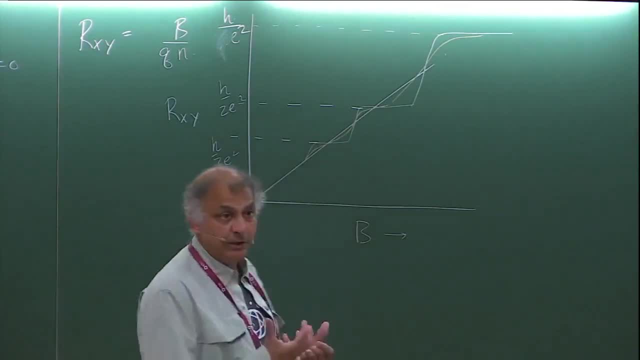 in normal material slabs. So you do expect oscillations as a function of the magnetic field in any physically measurable quantity, in particular the resistance. Okay, So they're all oscillations, but these oscillations, So let me draw them in a blue. 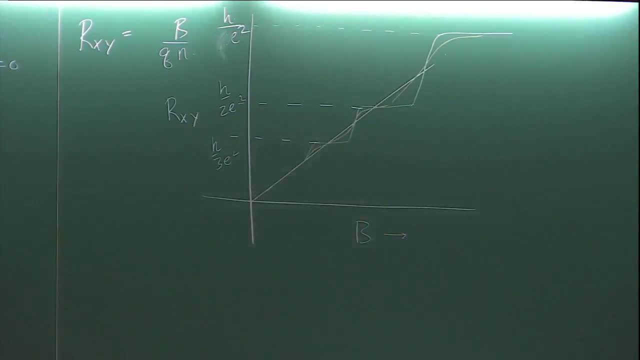 With a blue chalk. Okay, So these oscillations, Rxx will start out somewhere here and then there'll be some oscillations And then, as these plateaus, as you lower the temperature, these plateaus are getting sharper and sharper. 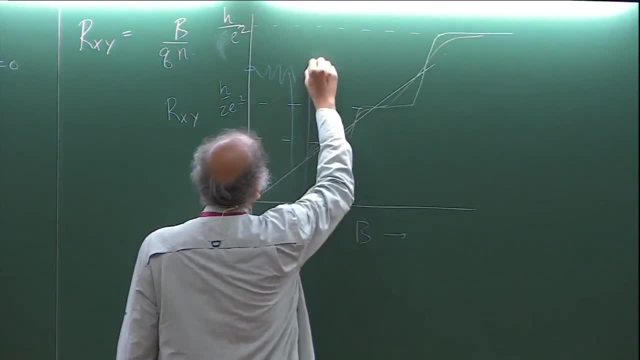 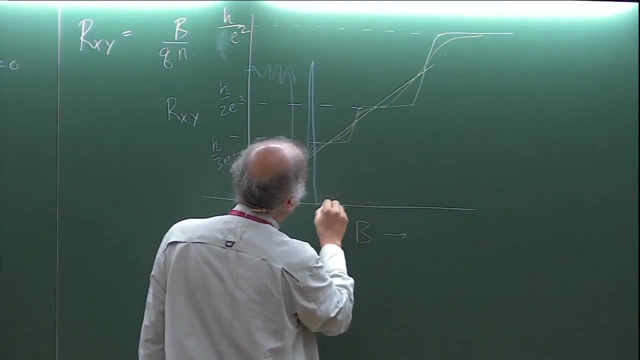 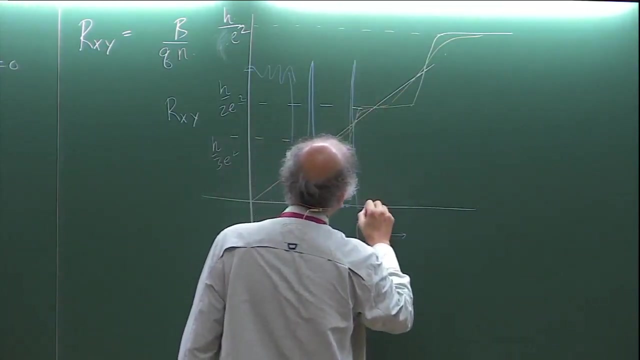 It turns out that when the plateaus are changing, this Rxx becomes very high, and during the plateaus, or in the region of B, where there are plateaus, this Rxx is very close to zero, And then again it spikes whenever the plateaus change, and it seems to do this. 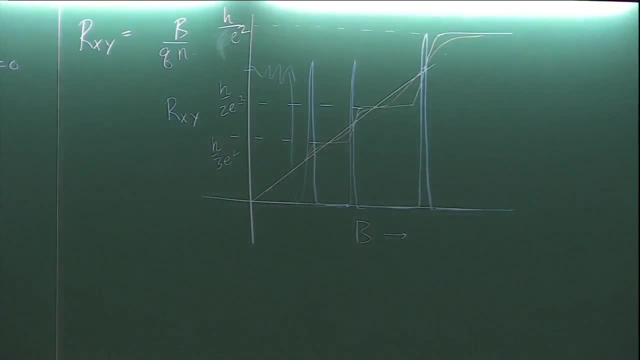 So this is what Rxx does? Yeah, Yeah, The amplitude of the oscillations, the Rxx, probably depends upon the material. Yeah, I think the idea is that as the temperature goes to zero, these oscillations are going to get sharper and sharper and the peak is going to rise. 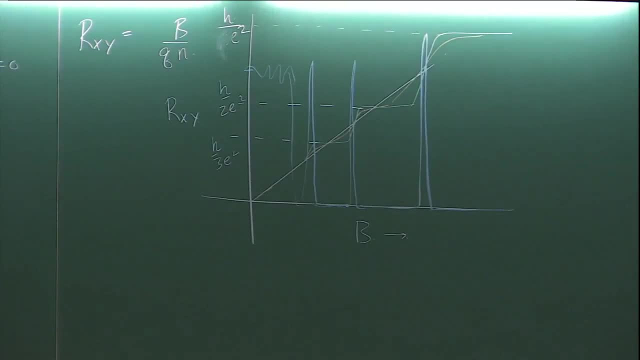 So it depends on the temperature and the material's properties. Okay, So this is what Rxx does. So what this is basically telling you is that in here, whatever electrons or particles are responsible for this Hall conductance, they're not able to scatter. 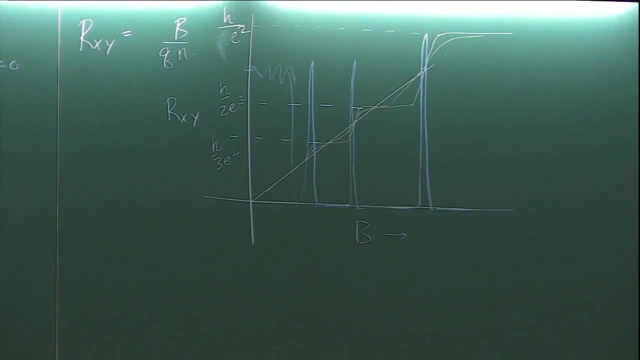 Okay, So there's no Rxx. That's what it's trying to tell you. Yeah, Yeah, That's not completely true, right? That's true classically. Okay, I'm not sure what you mean by the motion stops, but 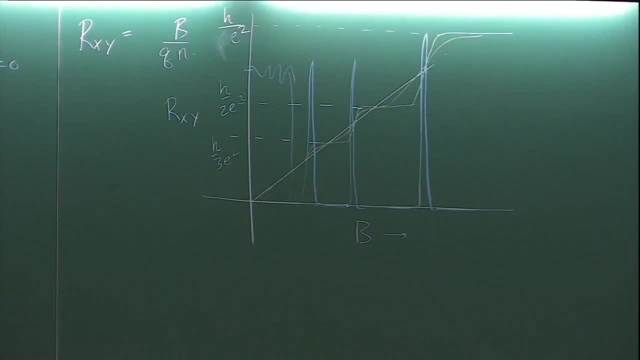 Okay, Go ahead Ask the question. Yeah, Why is the Rxx? Why is it not zero at certain points? Why it is not zero? Why it is not zero, Zero, Okay, In fact, Rxx. if you take a normal material, Rxx is almost always not zero. 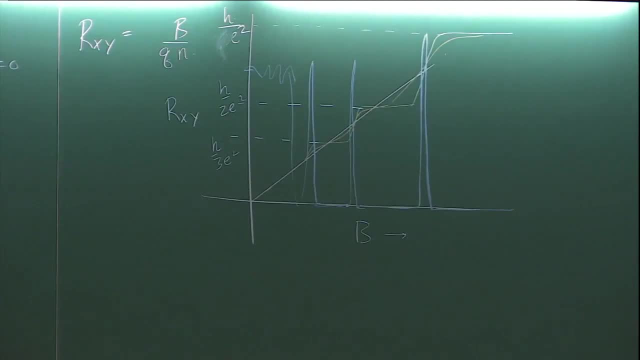 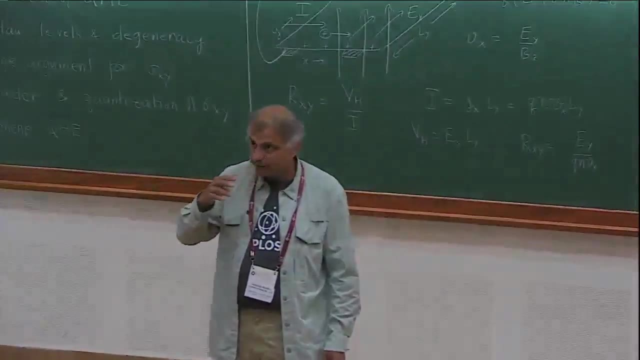 Right, If you take a metallic wire, something like copper, that does not superconduct, and you reduce the temperature of the wire, you will find that Rxx decreases as a function of temperature until it eventually saturates to some constant. Yeah. 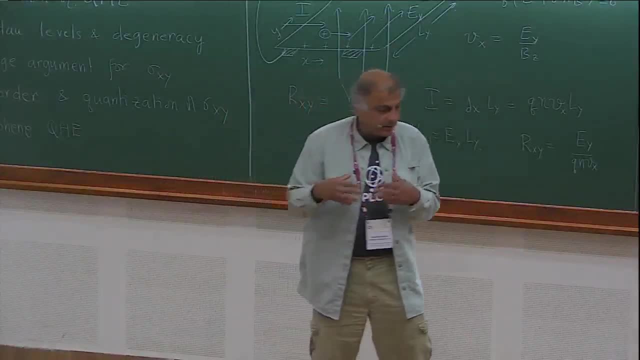 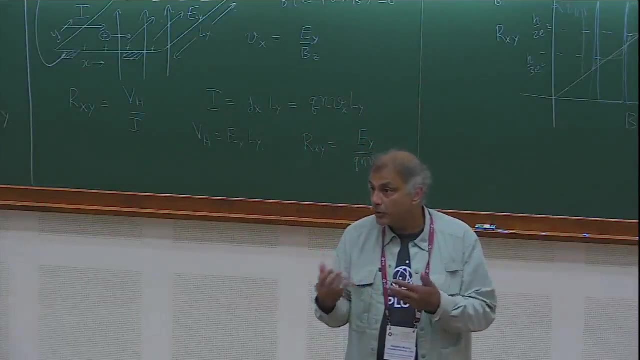 Okay, So it's not zero. Okay, So the reason for that? The reason for that is that even at zero temperature, or even at very close to zero temperature, the electrons can scatter off of impurities and therefore their momentum is not conserved. 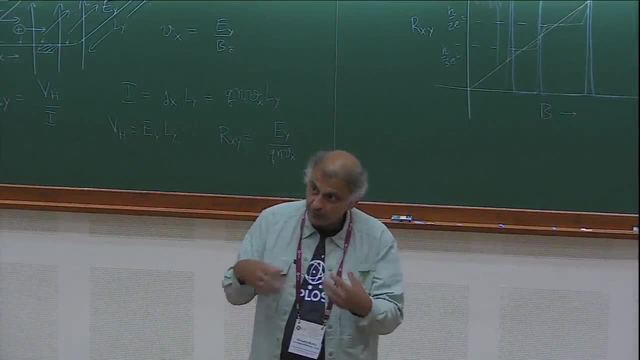 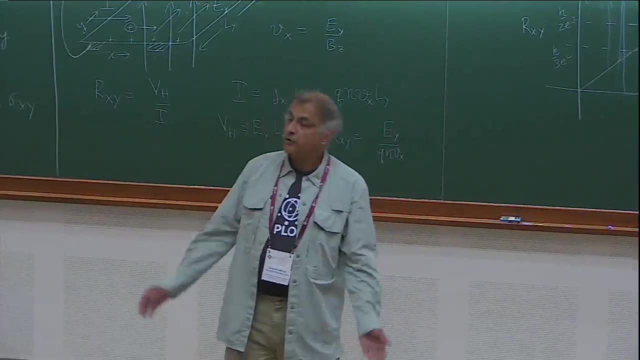 So whatever current you push through there, the electrons they're scattering off of the impurities and the current is getting degraded. So you have to impose a voltage in order to keep accelerating the electrons. Right, Okay, So Rxx not being zero is a normal situation. 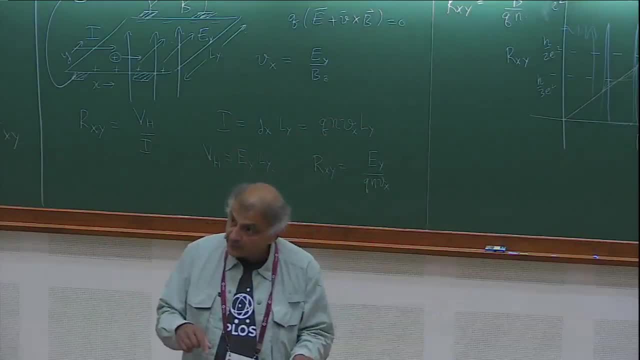 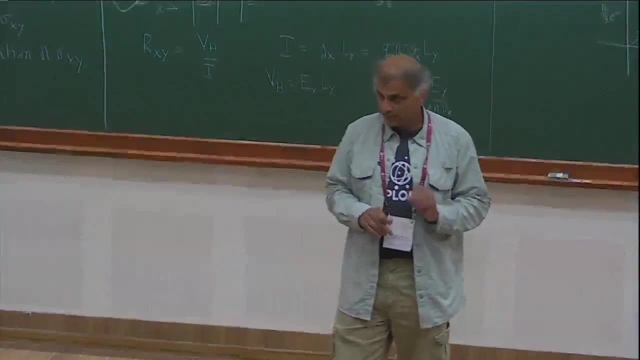 You shouldn't be surprised by that, Okay Okay, You should be surprised if Rxx is zero. That's much more surprising. You should be surprised if Rxx is not being zero than Rxx not being zero. Right, Okay, Yeah. 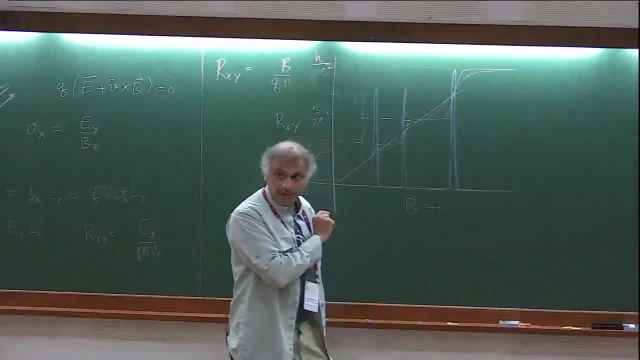 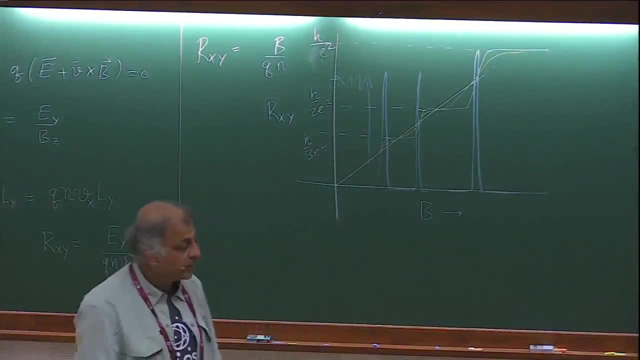 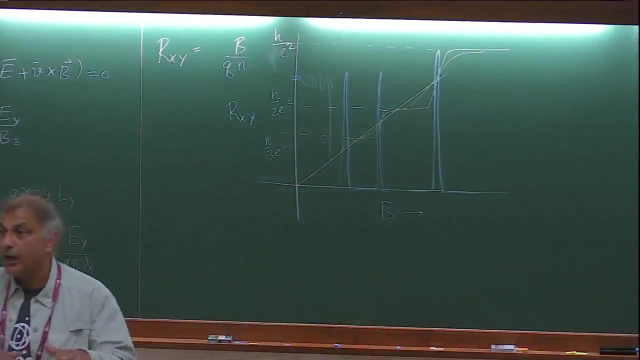 So in these spikes somehow it's behaving more normally, which means that during these spikes the electrons are able to scatter. But when you're not in these spikes, when you're inside the plateaus, whatever extender states there are that's allowing this transport of the Hall current, the electrons are not. 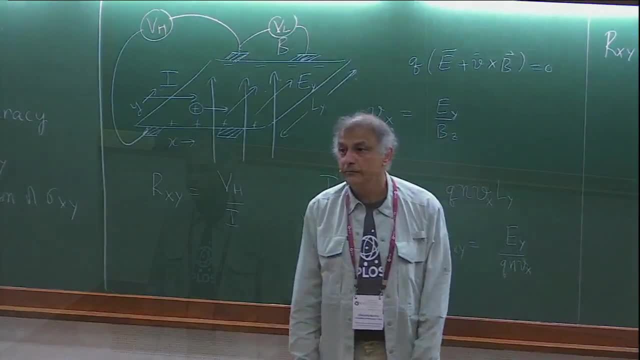 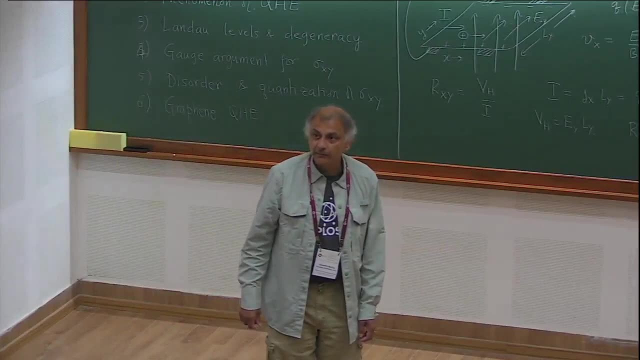 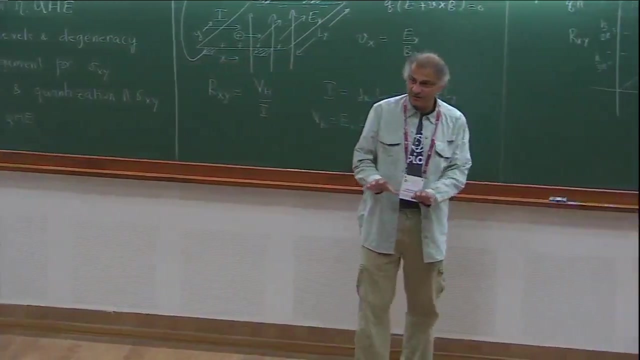 able to scatter. That's what it's telling you- That Rxx is zero. There's no scattering in the sample. How to understand that in a physical picture? I will show you, Okay, Okay. That's what this talk is going to end with. 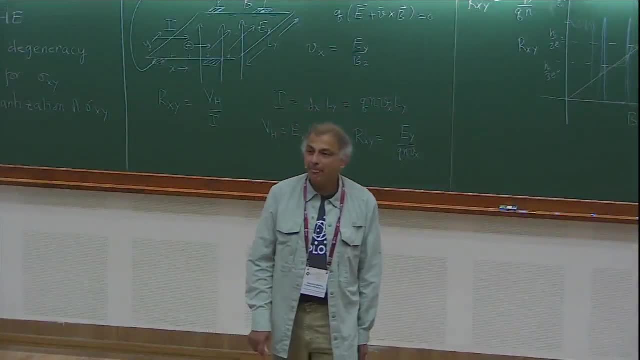 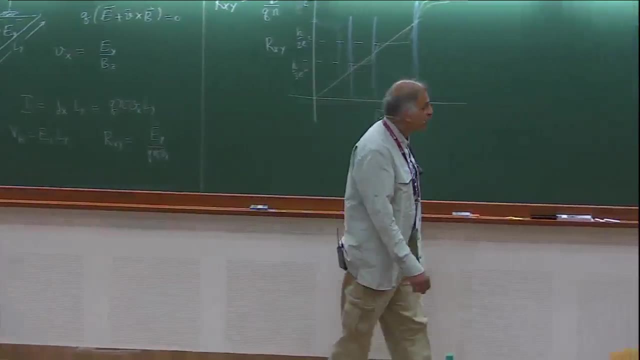 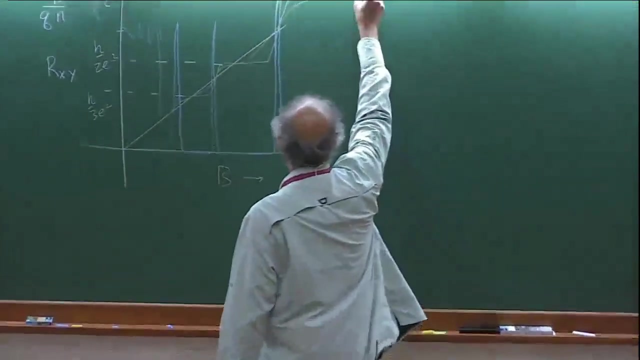 Okay, You will understand the physical picture of how that happens. Okay, Other questions? All right. So this is the phenomenon, So let's see how to understand it. So let's start with something very basic. We will start with a clean, non-interacting system. 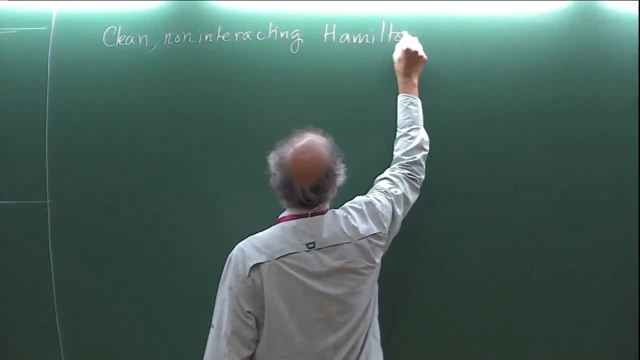 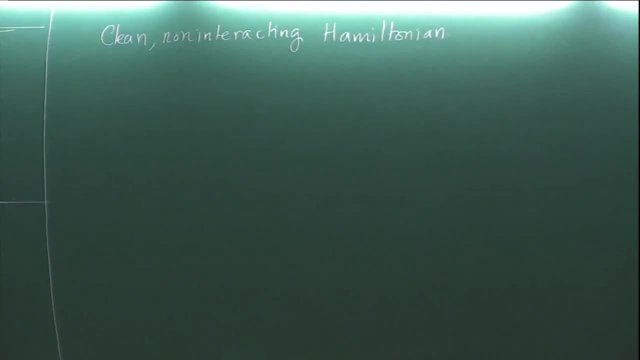 And we'll write down a Hamiltonian. Okay, So, this is extremely idealized, but this will let us actually at least start making some steps towards understanding what is going on, Okay, Okay, So what is such a Hamiltonian? Well, you have some quadratic band inside a semiconductor. 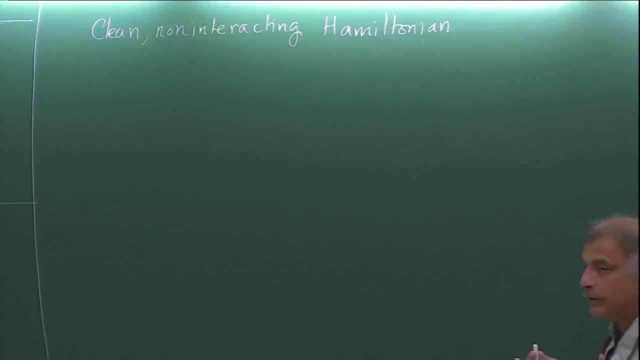 There's some charge carriers and they're subject to an external magnetic field. That's it. That's all there is. Right. If there were no magnetic field, then you would basically write down p squared over 2m. Right? That's what you would write down for your Hamiltonian in a quadratic band, assuming. 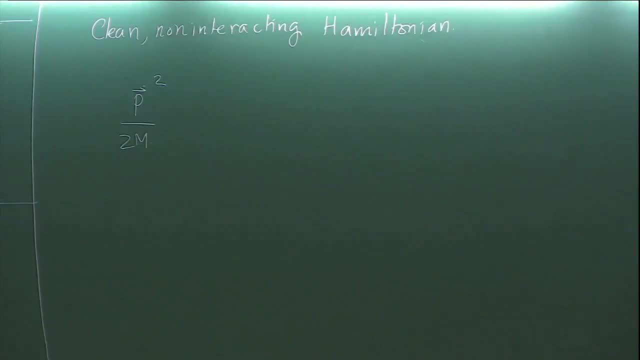 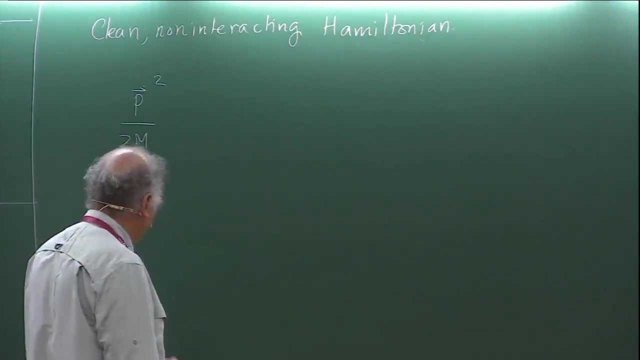 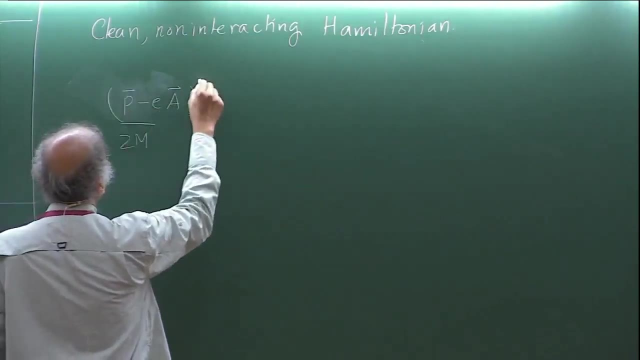 and bring it into this form. When there is a magnetic field, what happens is that this p gets replaced by p minus ea. Right, Where a is the vector potential that gives rise to the magnetic field. Right. So this is the Hamiltonian of electrons in a magnetic field. 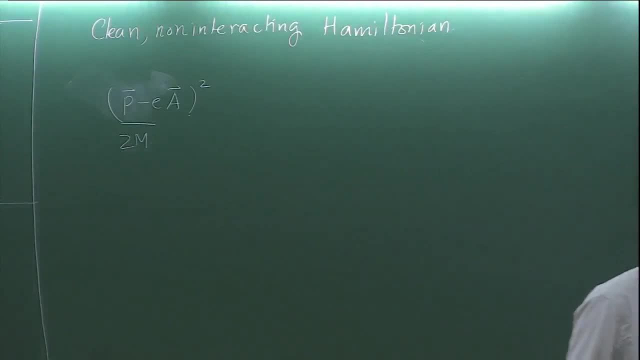 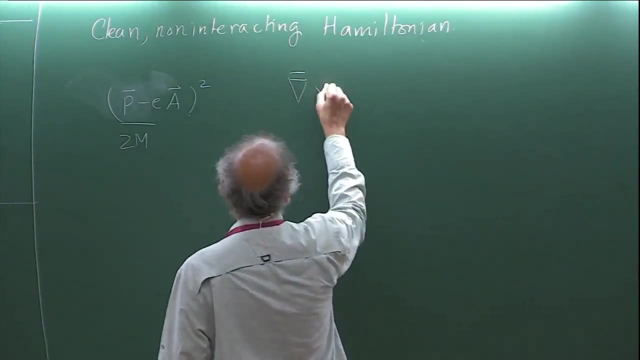 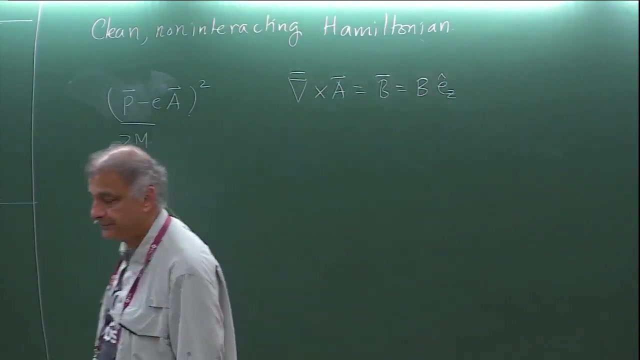 All right, This a is some vector potential. You can choose whatever gauge you want, as long as the curl of that a satisfies. our magnetic field is equal to our magnetic field, which is just b in the z direction. Okay, Now it it turns out that of course the Hamiltonian is always gauge dependent, because 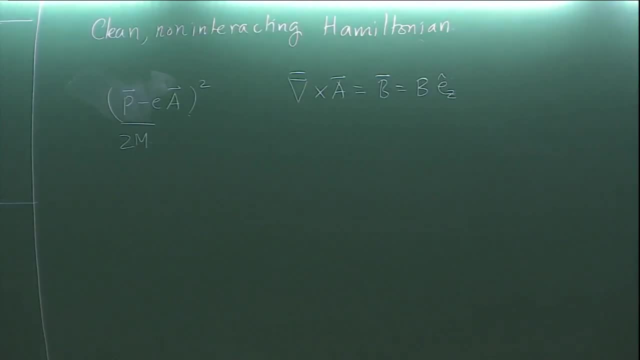 quantum Hamiltonians often come with, always come with the vector potential And the wave functions are also gauge dependent. but anything that's measurable, like a spectrum or like the expectation value of some physical operator, those things will not be gauge dependent. Okay, 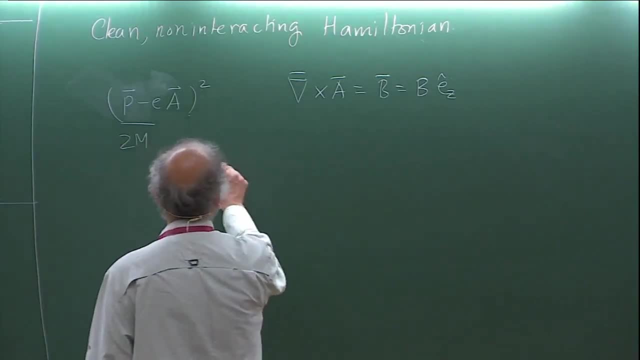 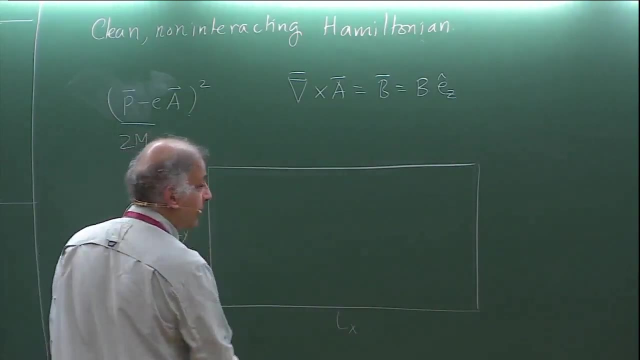 So let's choose a very simple geometry. Let's choose a geometry like this, where this length here is lx, this length here is ly. Okay, So it's as though I took that sheet over there and I laid it flat on the board. 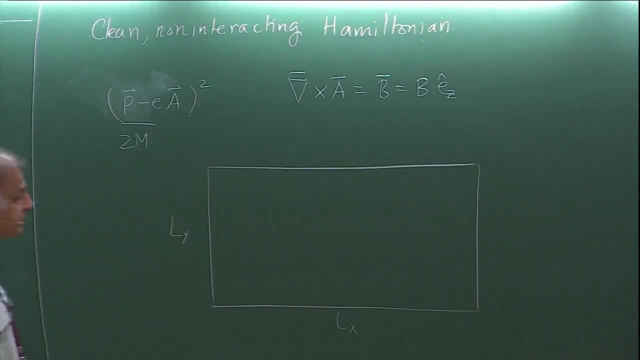 Okay, Now I'm also going to do something else. I'm going to make periodic boundary conditions, So this thing is really the same as that thing. So really, you should imagine this sheet being rolled up into a cylinder, Okay. 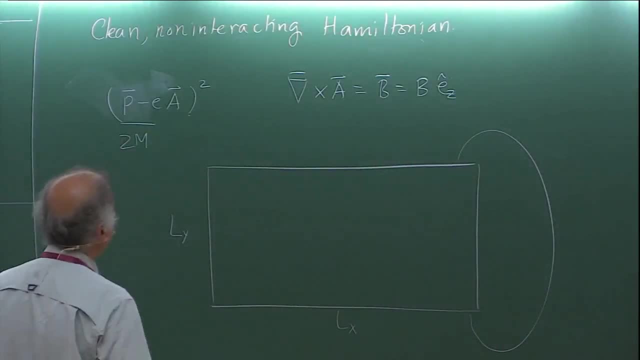 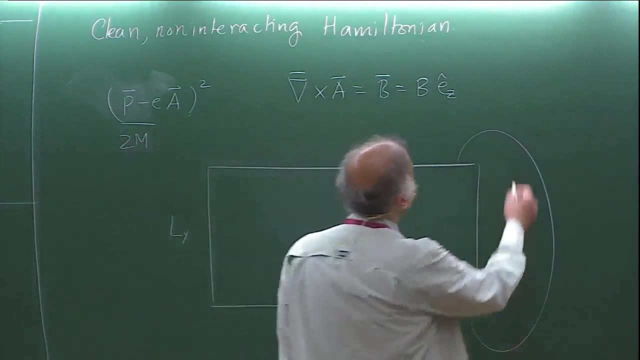 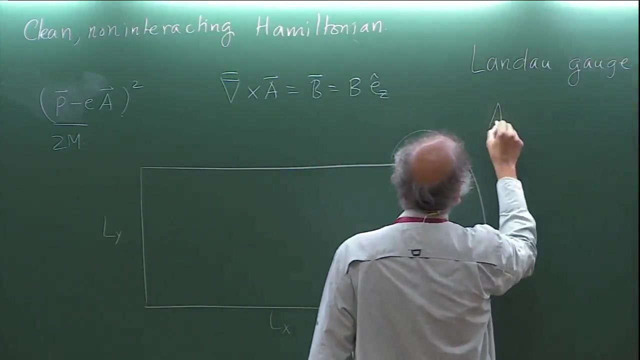 And that's the geometry that I'm going to be considering. Okay, So, for this particular geometry, it's very convenient to choose a gauge called Landau gauge. Okay, So Landau gauge is the following: You say that the vector a is equal to just ey times bx. 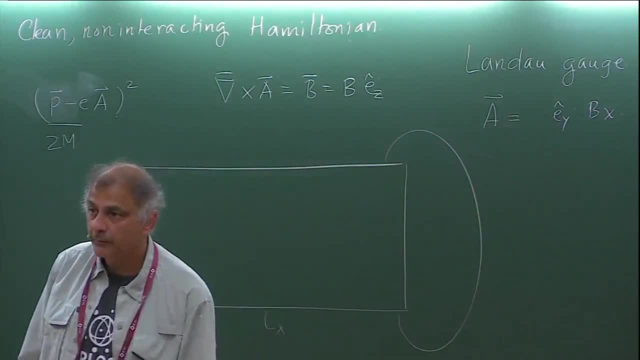 Okay, So x is the x coordinate, And then ey is the unit, And then y is the unit vector in the y direction. Okay, So you can easily see that the curl of this thing, the curl of a, will be, of course, dx. 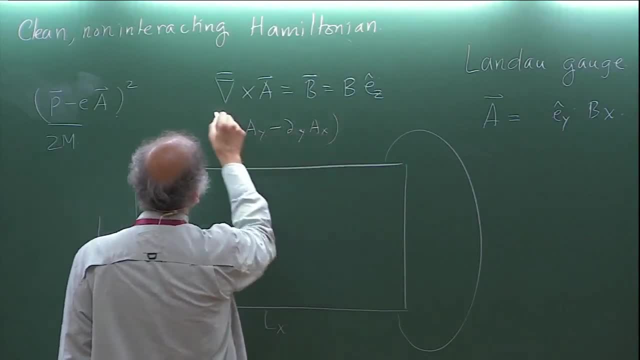 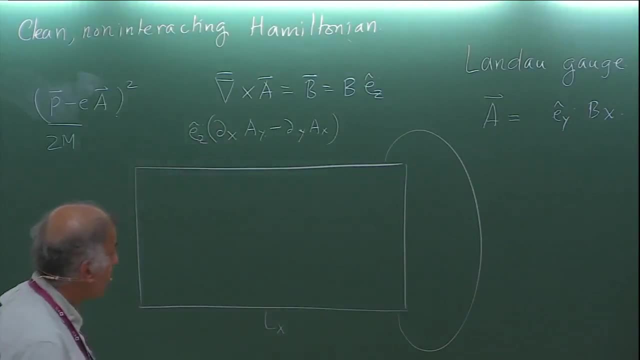 ay minus dy ax times, ez right, And that is equal to, in fact, b in the z direction. Okay, So now that I have it, let me write down my Hamiltonian. What does it look like? So it looks like px squared. 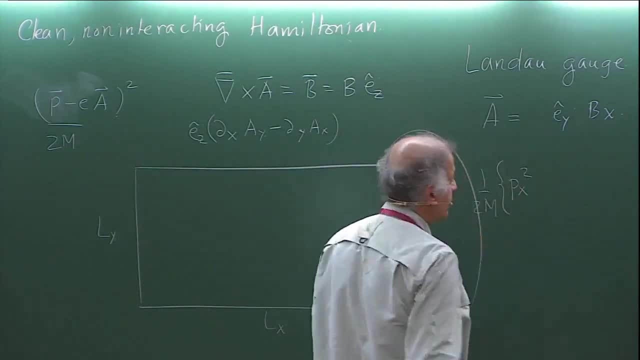 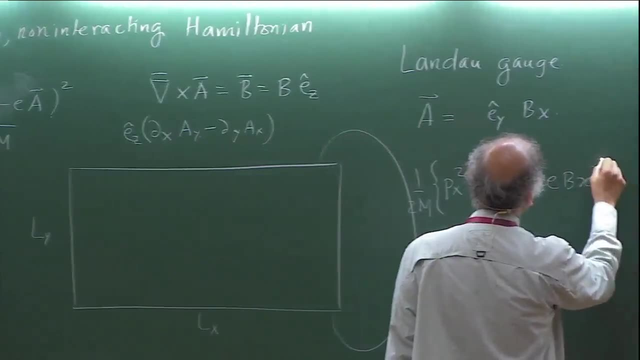 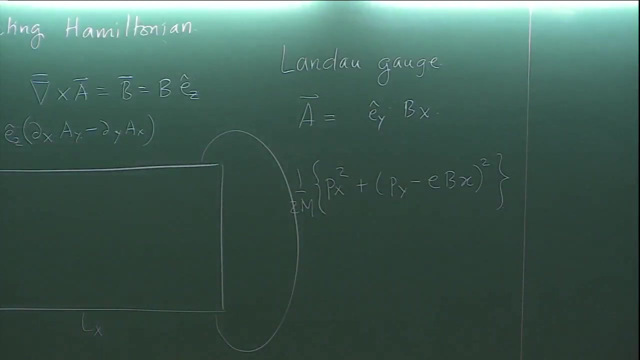 So there's a 1 over 2m sitting outside. There's a px squared. So there's a px squared plus ey, minus e, bx, whole squared. okay, That's my Hamiltonian. All right, You realize, of course you stare at it. whenever you see a Hamiltonian, you want to first identify. 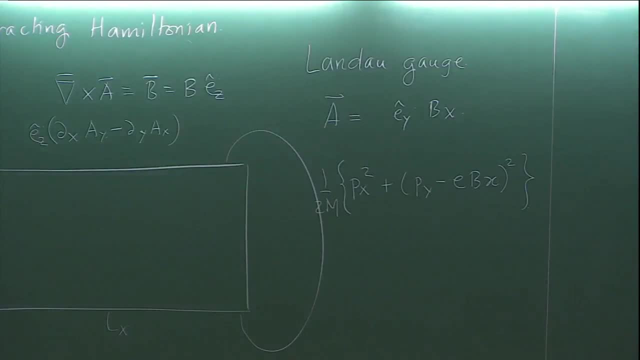 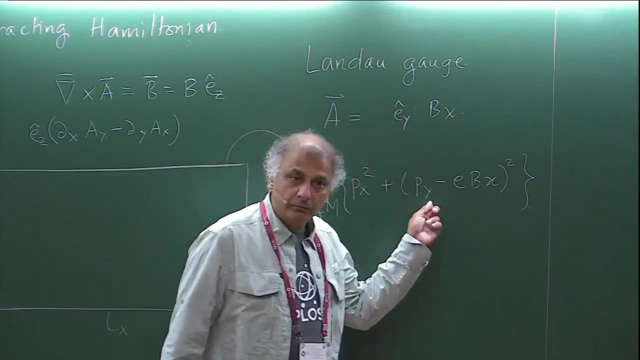 all the conserved quantities, because the conserved quantities of this Hamiltonian, of any Hamiltonian, will give you the quantum numbers of the states. So all right. So what is it that commutes with the Hamiltonian? Certainly x doesn't commute, px doesn't commute, y doesn't commute, but py does commute with. 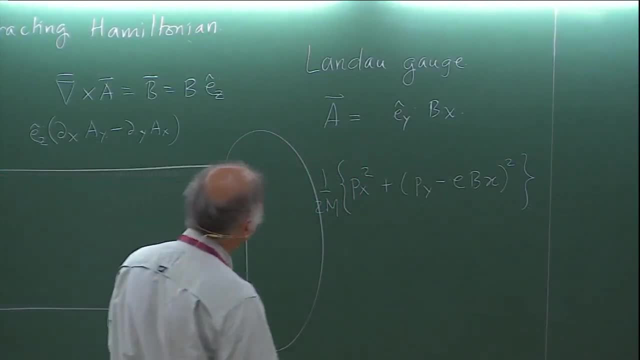 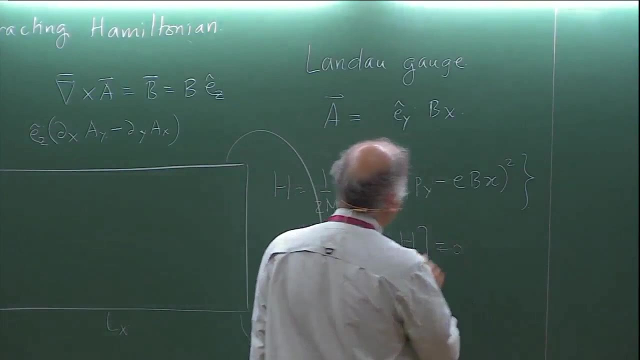 this Hamiltonian. Okay, So py is a conserved quantity, So I can say my Hamiltonian is this: So py commutes with h And therefore I can label my states by the quantum number, which is the eigenvalue of. 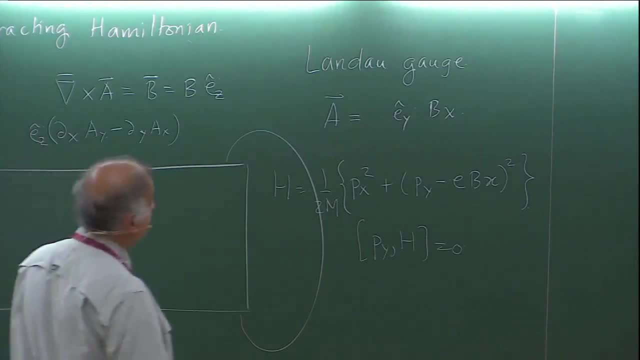 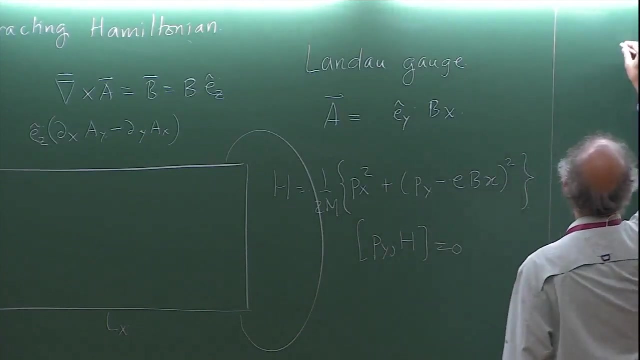 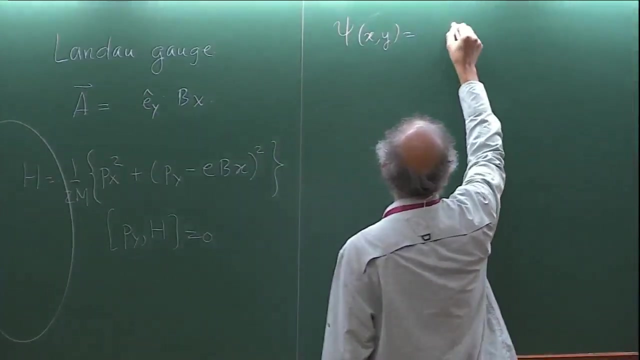 py. All right. So therefore, what is the conserved quantity? Okay, So what are the eigenstates of py? Eigenstates of py are Okay, Very good. They're plane waves in the y direction. So therefore, I can say that my wave function, psi of x and y is going to be equal to sum. 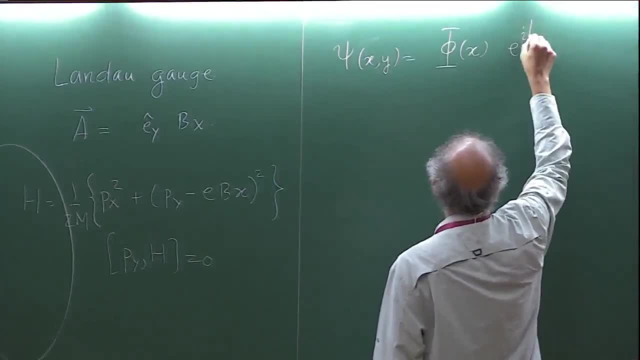 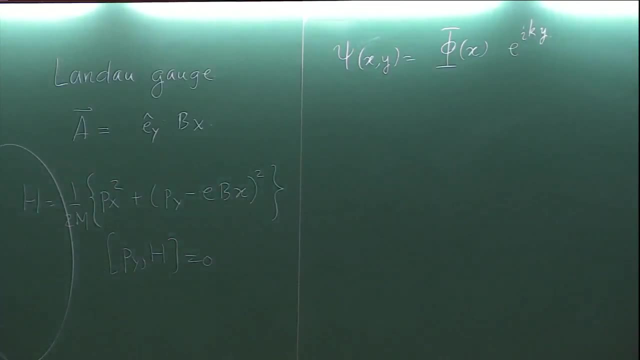 phi of x times e to the power i ky. Right Here is going to be the momentum. Okay, Here is going to be the momentum in the y direction. And because I have chosen this particular periodic boundary condition- and I'll tell you why in a second, why I chose that. 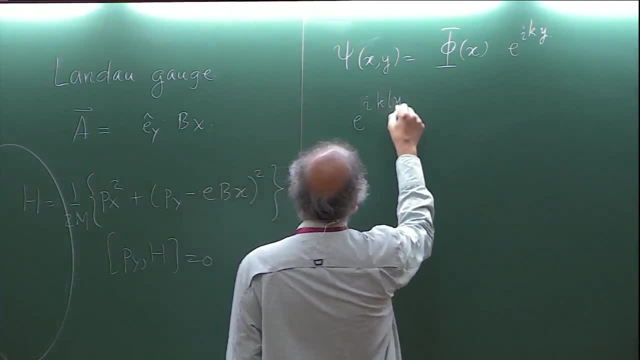 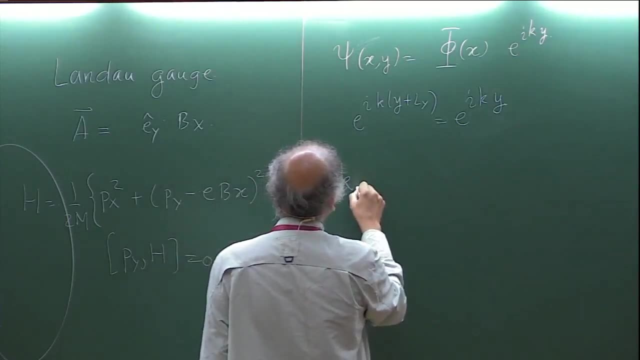 Because I chose that. I realized that e to the i ky plus ly must be e to the i ky, And this tells me that the values of k should actually be labeled by an integer and they should look like this: Okay, So stare at that for a second and convince yourself that it's correct. 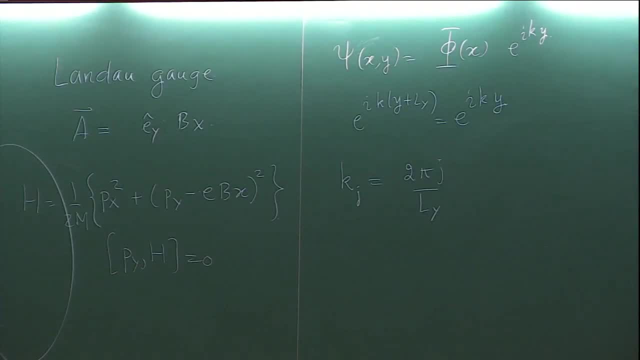 Okay, Fine, All right. So now that I have this, I plug it in here and I ask myself what is the differential equation for phi of x? And I want to solve it. Okay, So let me write that down here. 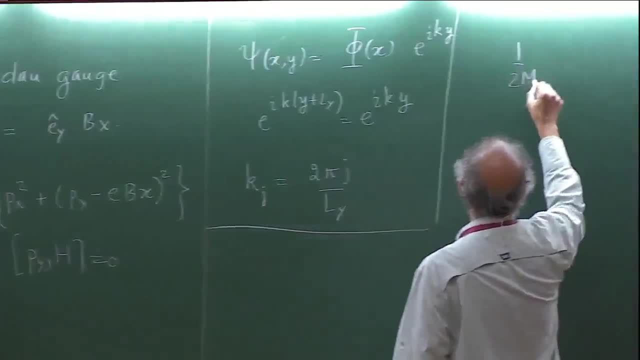 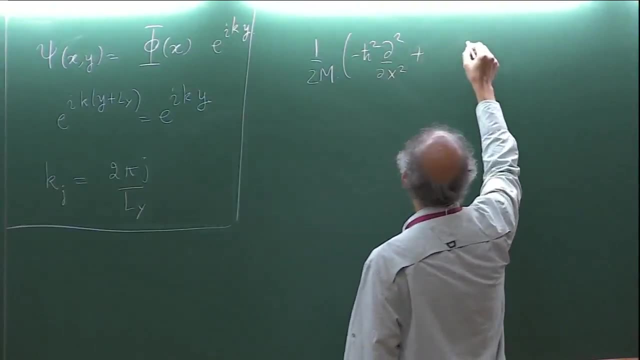 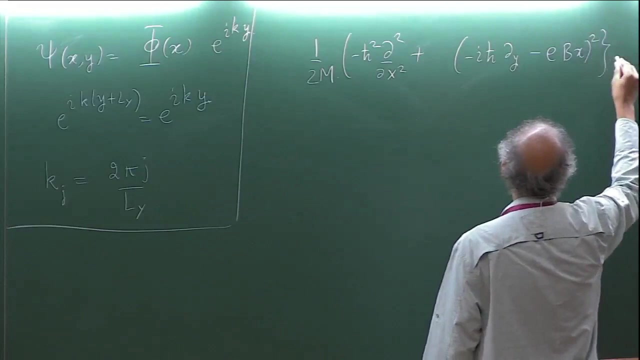 Okay, So I find that 1 over 2m have minus h bar squared, d squared by dx squared, plus minus i h bar, d by dy e b x squared. sorry, I should be consistent in my brackets: e to the i ky. 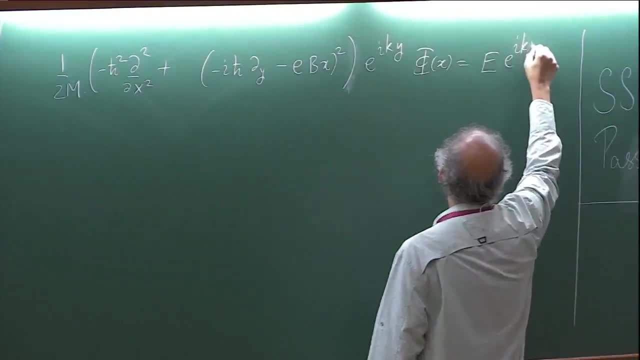 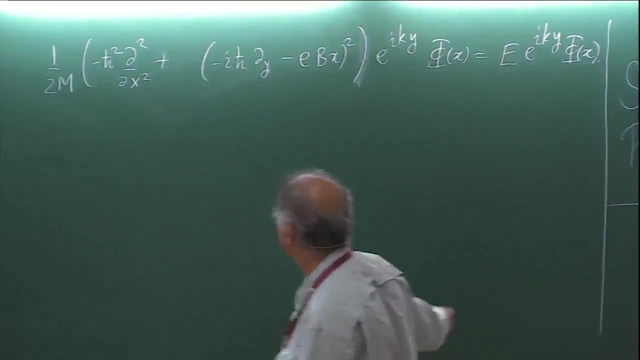 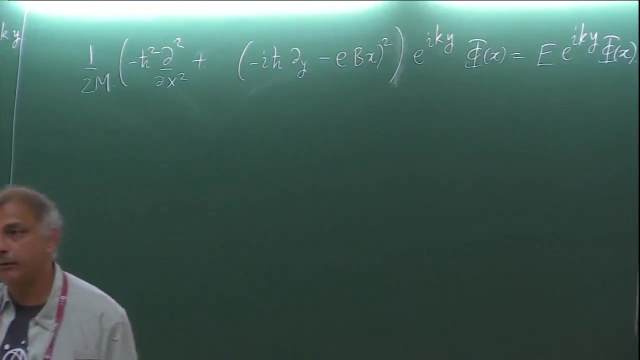 plus y of x is e. okay, this is the equation I want to solve. Of course, I've chosen it in such a way that this minus i h bar dy, acting on that, will give me an eigenvalue acting on the same thing, right. 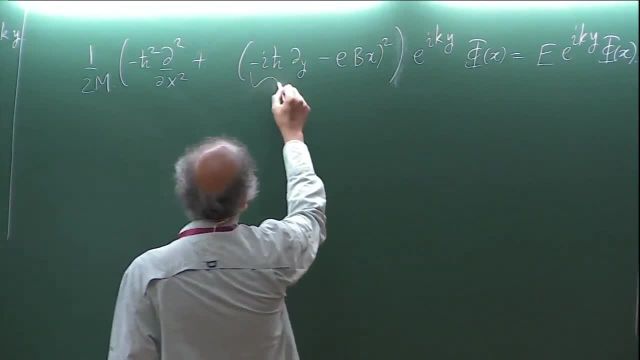 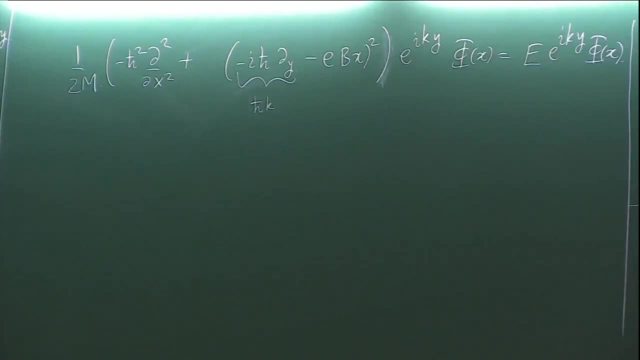 So I just plug in for this. this guy acting on that wave function is just going to give me h bar, times, a, k, And then I can cancel e to the i ky on both sides, Okay, And I end up with something that looks like this: 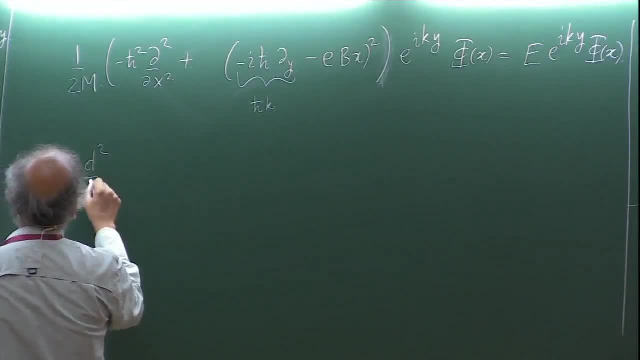 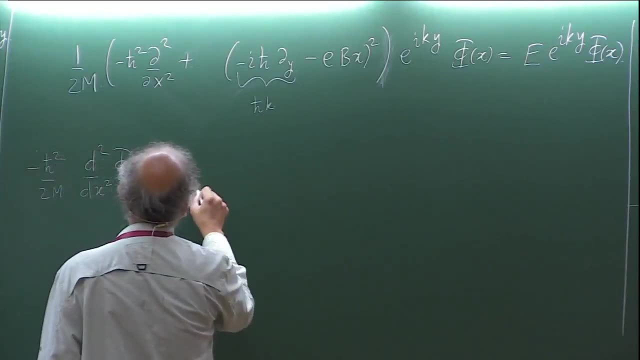 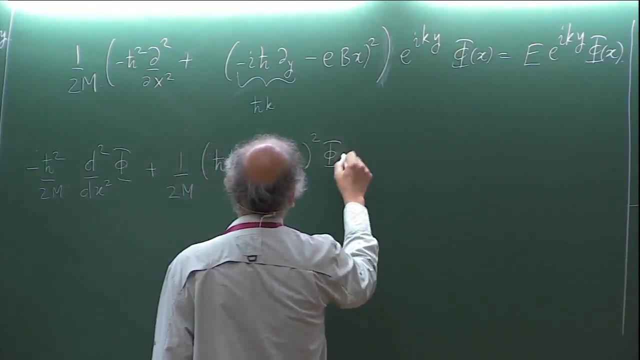 Minus h bar squared over 2m, d squared by dx, squared of phi plus. okay, and now let's see what happens here. So 1 over 2m h bar k minus e, b, x squared phi. Okay, Really what I should be doing. 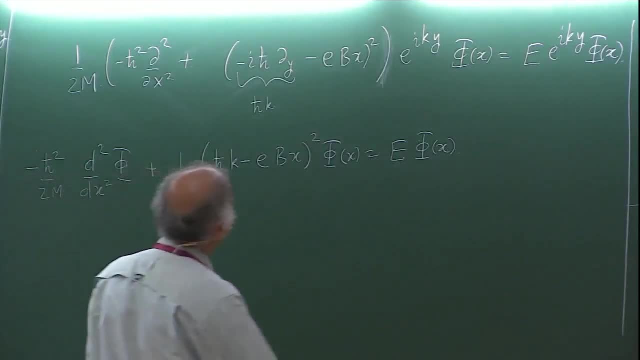 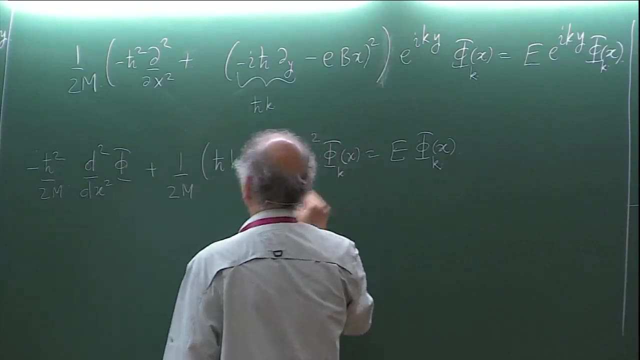 Okay. Okay, So I should, I should be labeling this phi by that quantum number, So let me do that. Okay, So there's a phi sub k here, because of course this is the equation for the phi of x, that 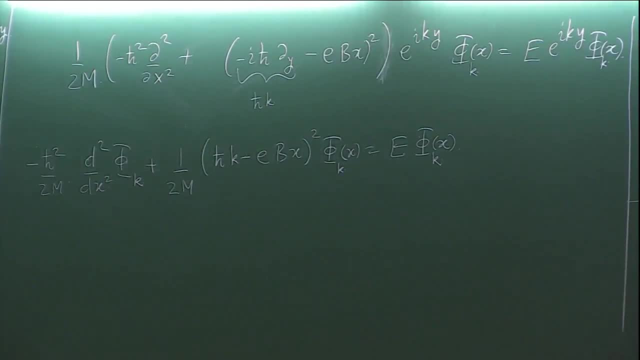 goes with a particular eigenstate of p y. Okay, Good. So if I take out this e b outside, you will see that it looks like a shifted harmonic oscillator, Right, And so it makes it very easy to solve. So to do that, you have to identify a particular length scale called the magnetic length. 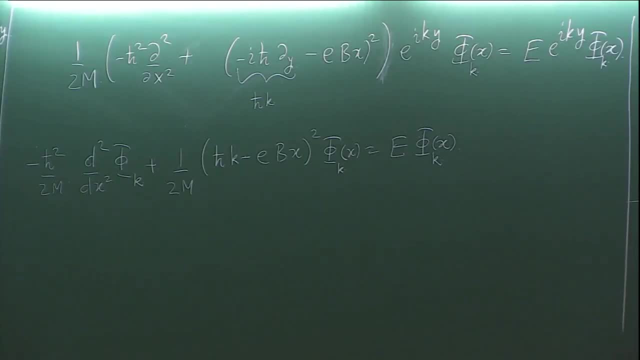 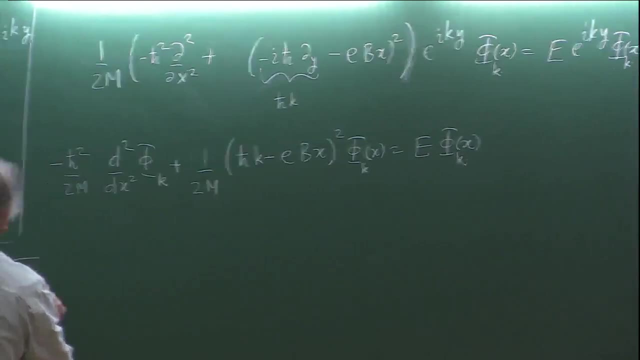 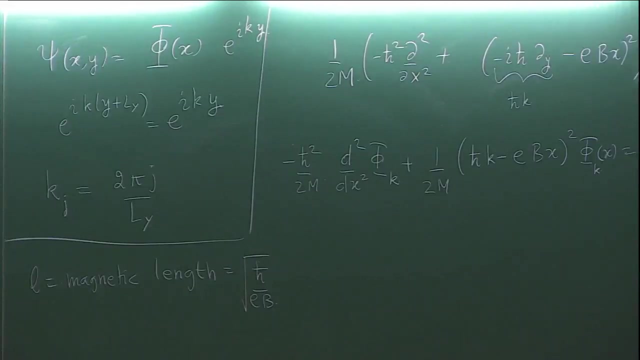 So this L is the magnetic length and it's the square root of h bar over e b. By the way, everything that I'm doing is in MKS units. If you want to go to CGS units, you have to replace the e by e over c. 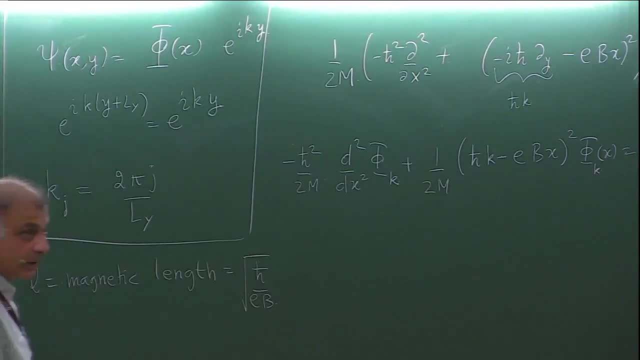 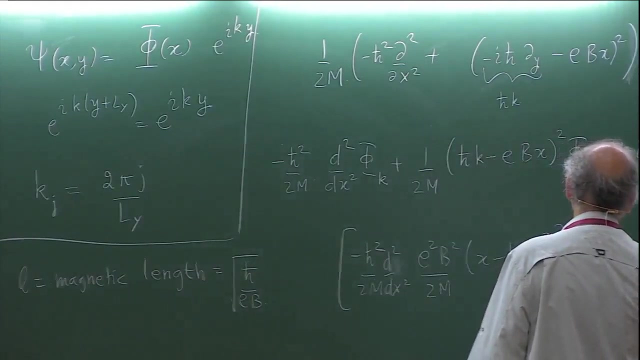 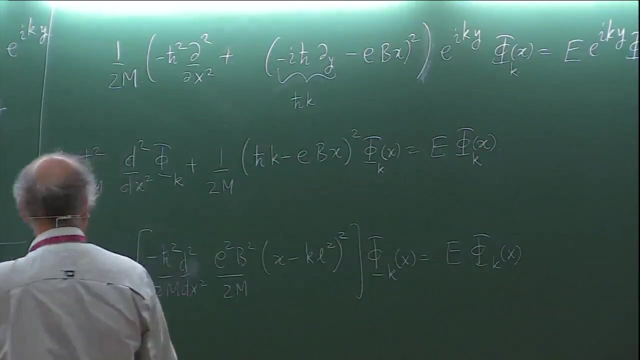 Okay, All right, Good. So you identify the magnetic length, and then this whole thing looks basically like: minus h- bar, squared over 2m, plus e, squared b squared over 2m. x minus k, L, squared- squared. Okay, That's what it looks like. 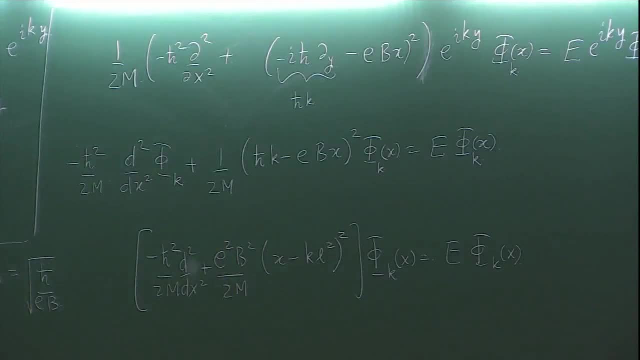 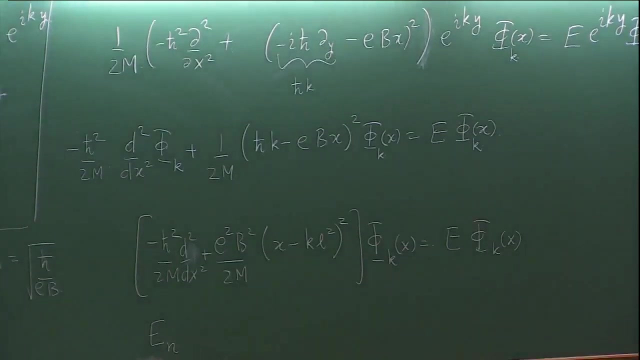 Okay, This is just some simple harmonic oscillator. You solve it. You know what the eigenstates are. You know what the eigenenergies are, Right? So the energies are labeled by a quantum number, n, that goes from zero to infinity. 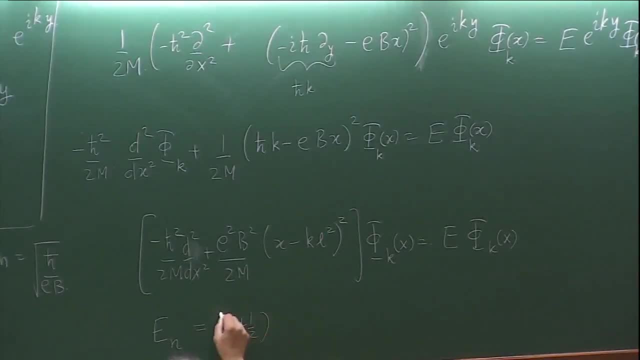 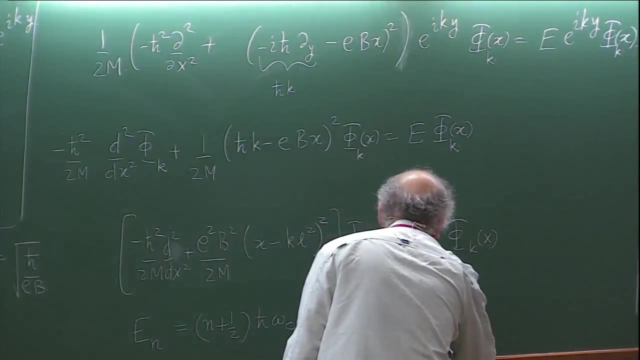 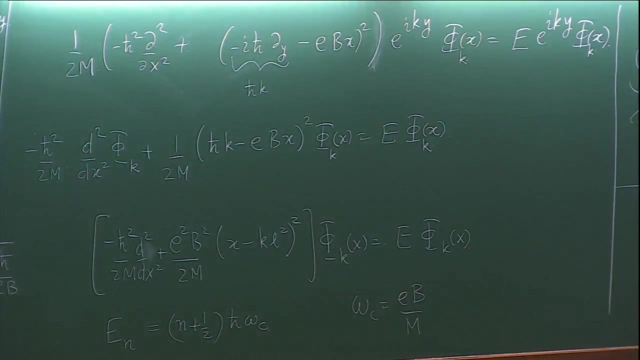 Okay, And this is just n plus one half h bar omega c. Omega c is the classical cyclotron frequency, e b over n. Okay, All right Now. one striking thing about this solution is that the energy ended up not depending upon the quantum number k at all. 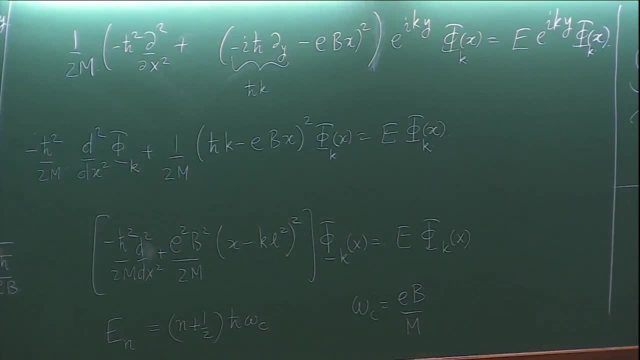 Okay, So for every value of k you actually have the same energy. And now you ask yourself, how many different values of this particular energy are there? Okay, So let's go back here. Any questions before we start counting the degeneracy. 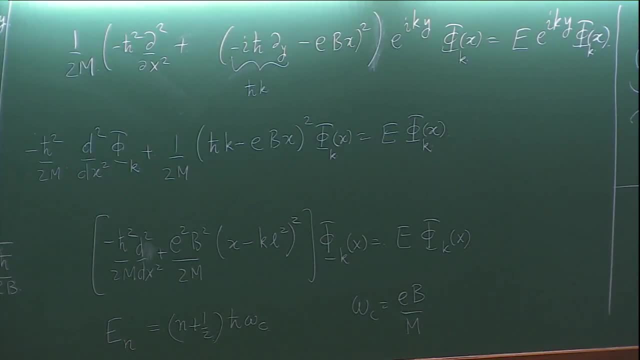 Everybody understands the solution right, Because I didn't go through the solution of the harmonic oscillator, But presumably you have seen that many times. Sorry, Go, go, go. Yeah, We did not consider the finite size in the LX direction, because then 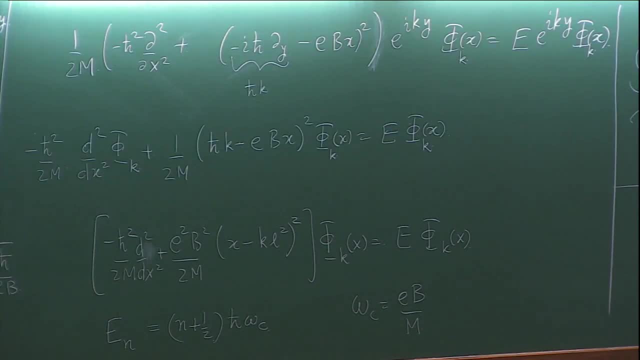 In the x direction. The solution is not. I have considered the finite size in the y direction. Yes, but that's a equation in x. Yeah, That solution is valid only for x. Yes, Yes, Yes, Yes, Yes. 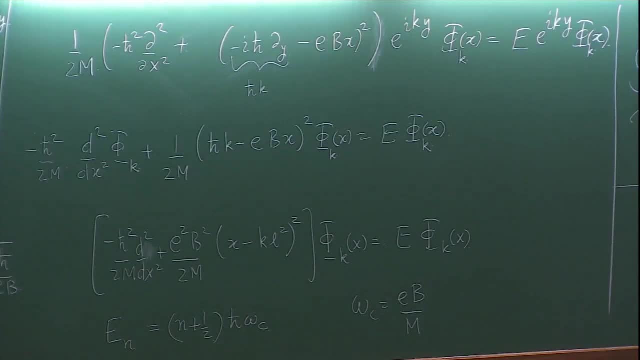 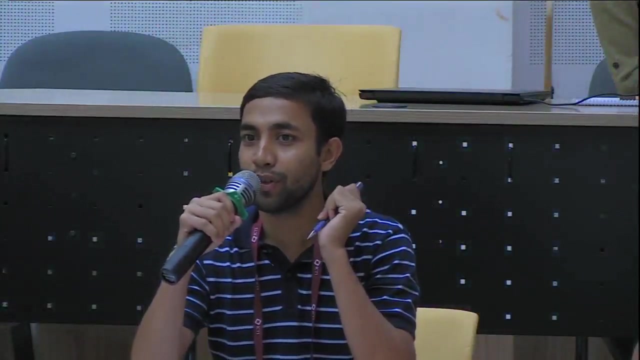 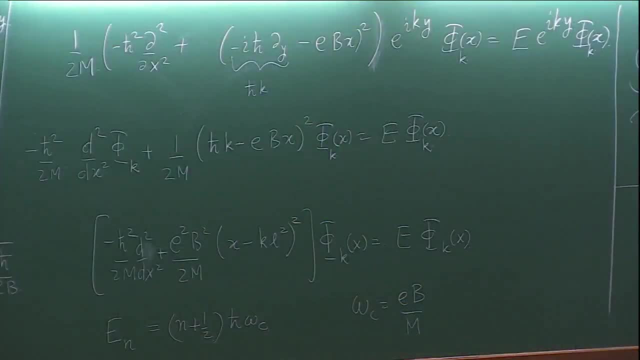 Okay, Good point. Okay, So he's saying that, basically, the solution that I have is the solution of the harmonic oscillator when it has an infinite interval minus infinity to infinity is not really valid when I have a finite interval, And that's correct. 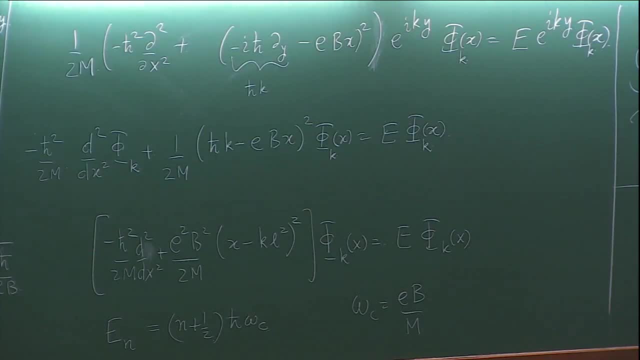 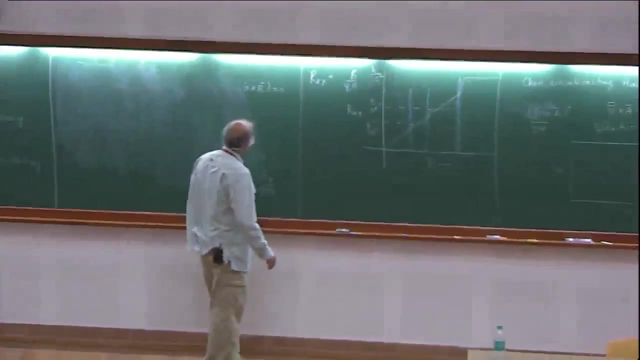 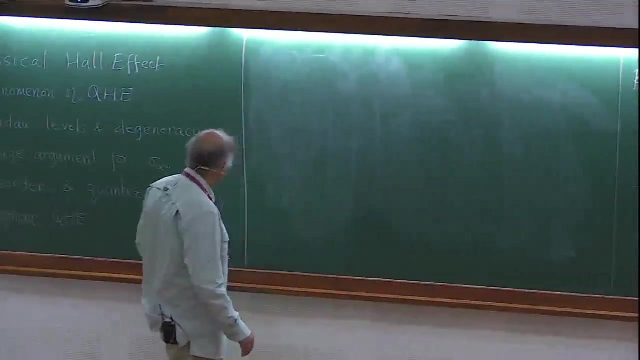 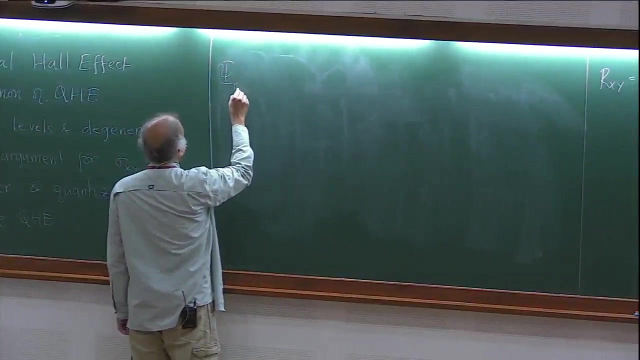 Okay, it turns out that it's okay to do this. and why is that? because you see these harmonic oscillator solutions. they decay very rapidly in X around their center. so let me write down the actual solution of this harmonic oscillator. what does it look like? so here is the, the total psi, which has, of course, two quantum numbers. 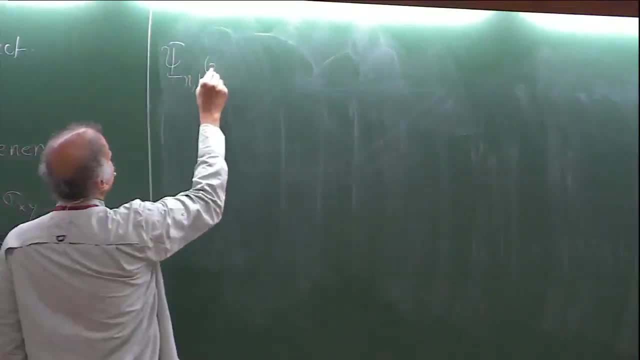 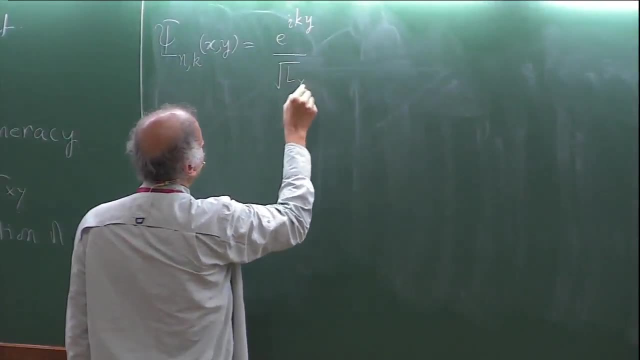 it has n and it has K, right, and it's a function of X and Y in the Y direction. you know exactly what it is: it's e to the IKY over square root of L Y. okay, that square root of L Y is to normalize it in the Y direction and in the X. 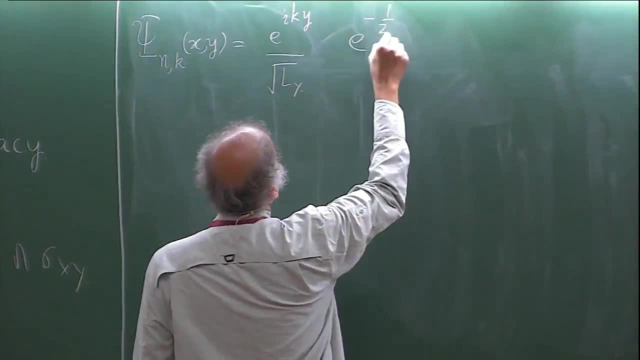 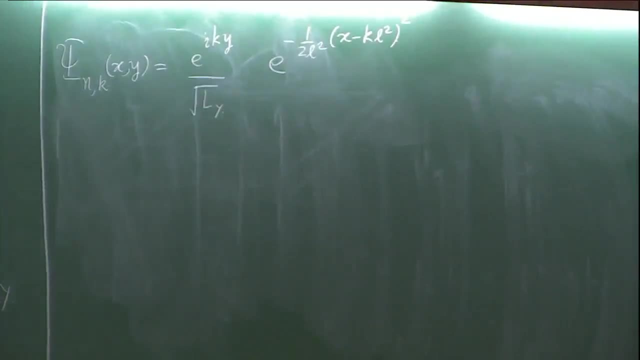 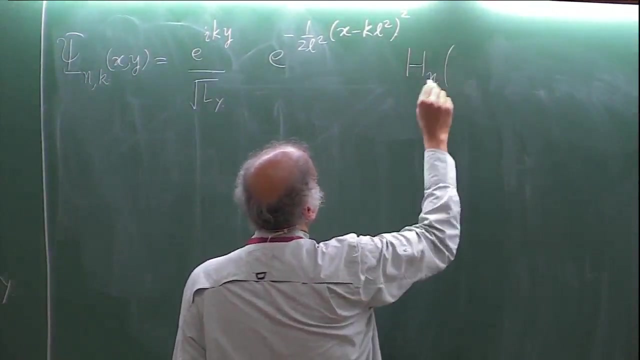 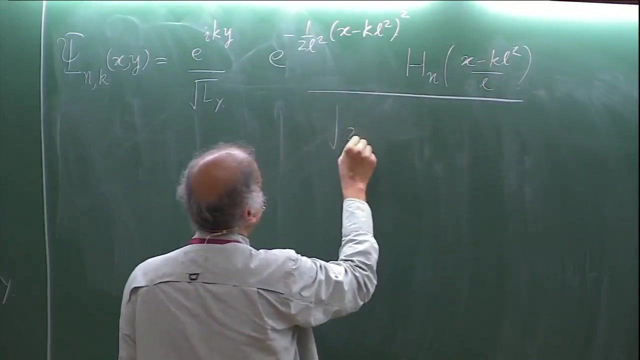 direction. what is it? well, it's something that looks like this: so it has a Gaussian kind of decay around its center. the center is KL squared, okay, and then there's some nth Hermite polynomial of X minus KL squared over L, and there's some normalization factor, some insane thing, something like this: 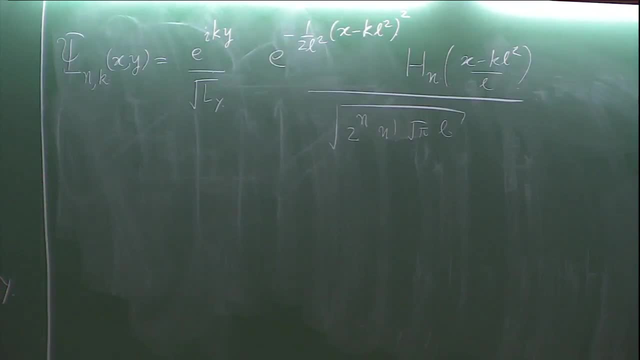 okay, so that's your eigenstate. now, the most important thing to notice about this eigenstate is that it is centered around KL squared. that's point number one, and point number two is that it decays like a Gaussian as you go away from it, and the length scale at which it decays is this magnetic length L. 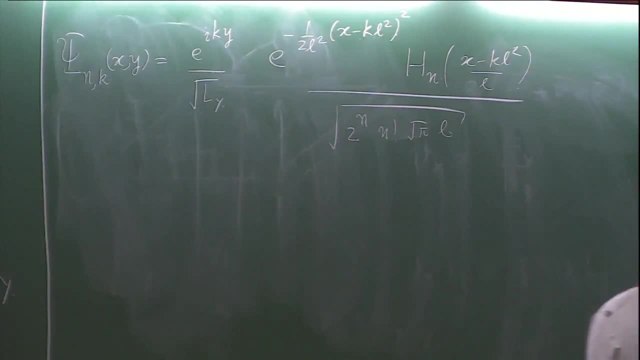 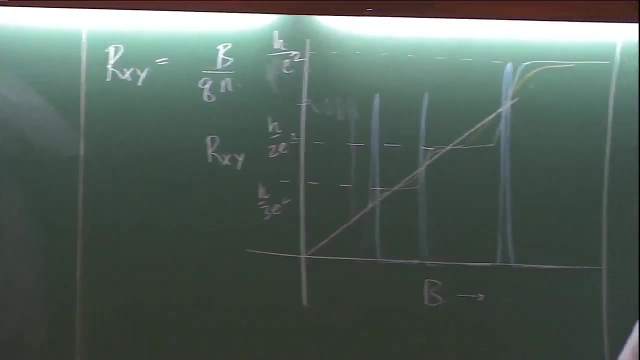 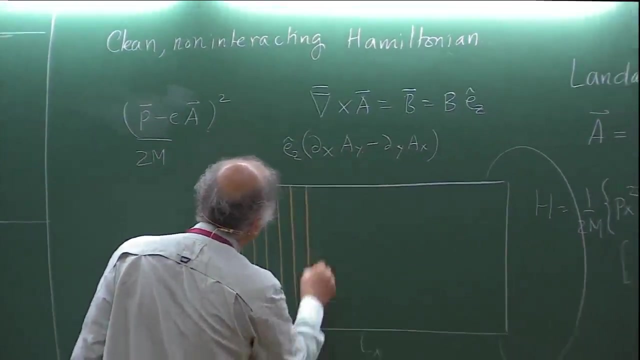 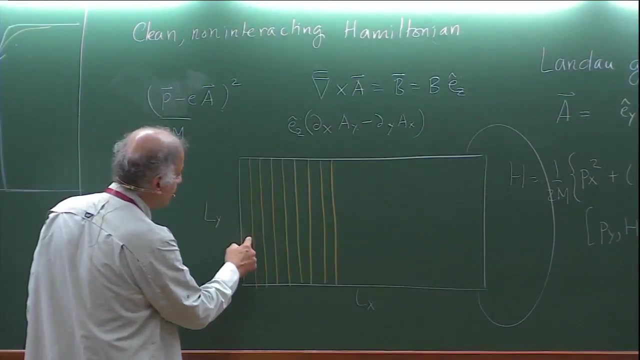 okay. so if I go back to this strip that I have drawn here, let me draw some lines here. okay, so each of these lines is supposed to indicate the center of one of these eigenstates. okay, so let us say that this will be: J equals zero. this is: 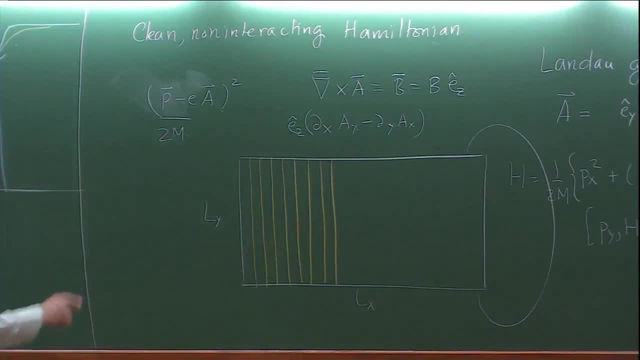 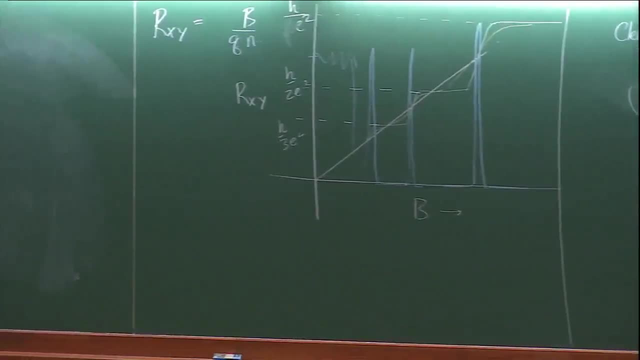 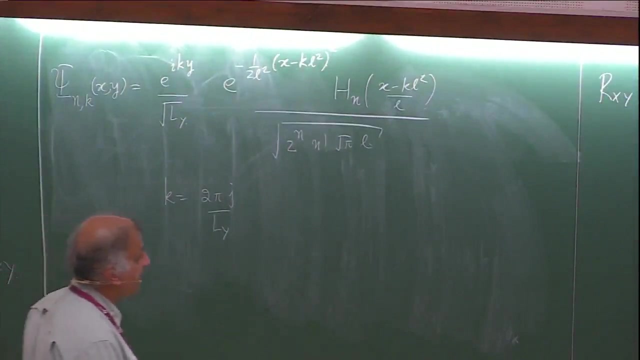 J equals one, J equals two, J equals three. and what is J? remember J is. K was equal to two. pi J over L, Y, right, that's what J is okay. so there's a discrete set of K labeled by an integer J, and for every value of K, the land our orbits around a. 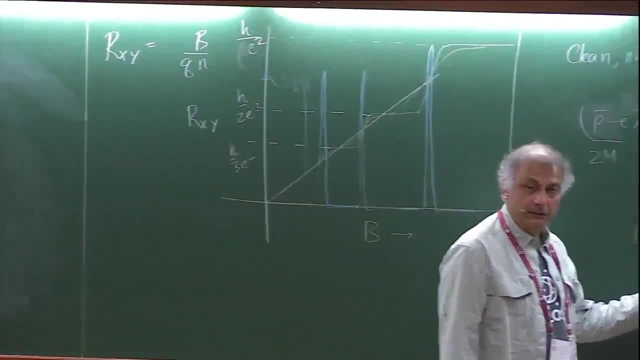 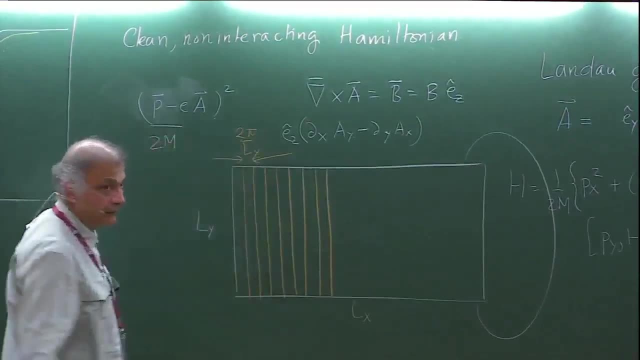 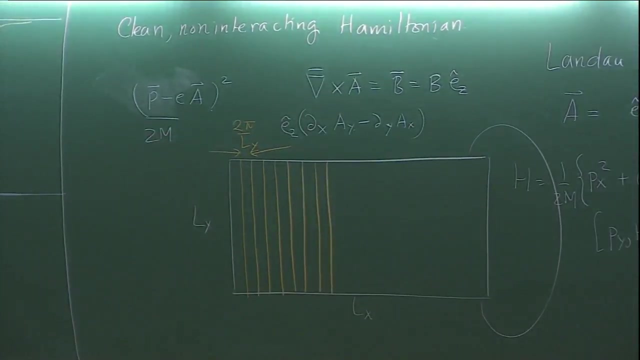 different center. okay, the spacing of these guys here goes like this: okay, so this is like two pi over L Y. okay, it's got nothing to do with the magnetic length. it has to do with how broad your sample is in the Y direction. okay, so, as I make, 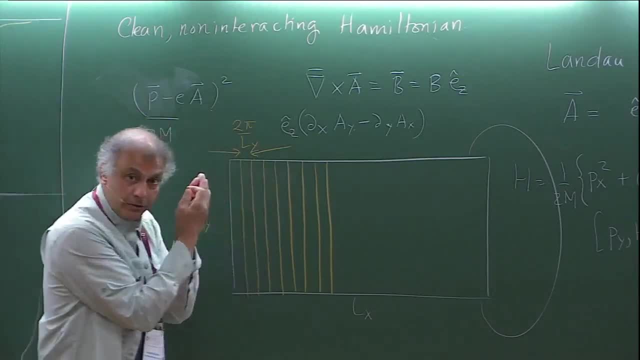 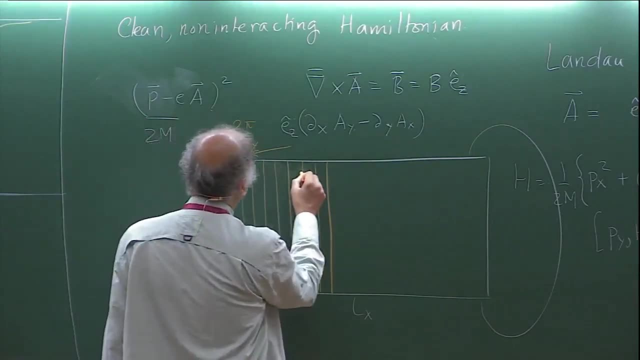 the sample bigger and bigger in the Y direction. these orbits will get closer and closer to each other, these centers. okay, now what is the magnetic length? on this length scale? it'll be something like this: so say, I take a particular orbit here. it'll be something like that. so this will be the shape of the 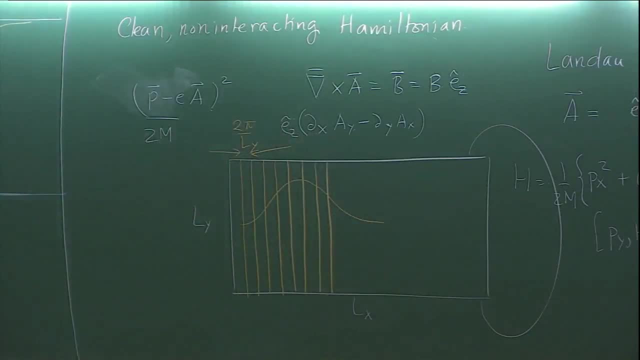 shape, which is that Gaussian, okay, around a particular center. yeah, yes, very good, thank you. so the distance is actually L squared, sorry, two pi over L? Y times L squared, thank you. okay, so the distance of the two successive K values is two pi over L? Y, but the distance of the two successive centers is delta K times L. 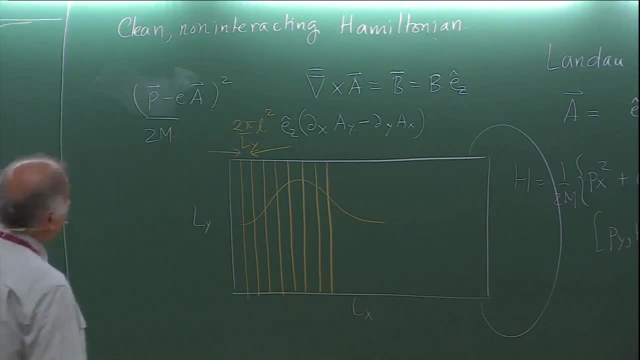 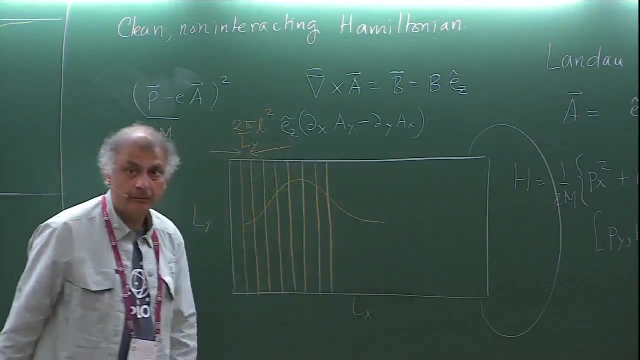 squared. okay, good. so in general, for some macroscopic value of L Y, this envelope of all these harmonic oscillator wave functions is going to be much, much bigger than the separation of successive guiding centers. okay, all right. however, the hierarchy of length scales is such that you want to have two pi over L Y times, L squared. 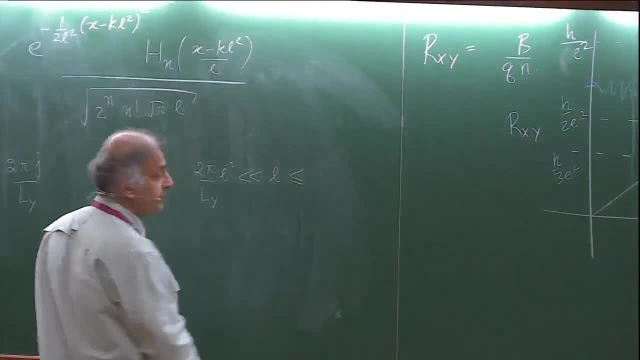 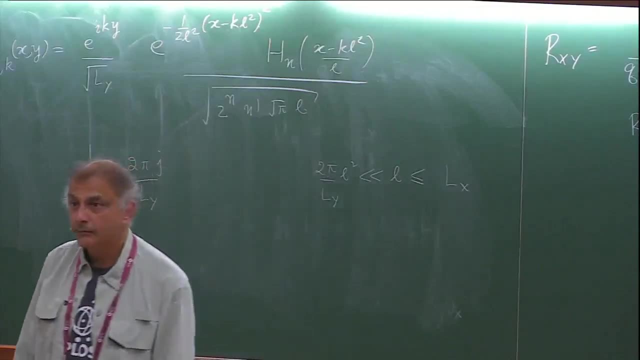 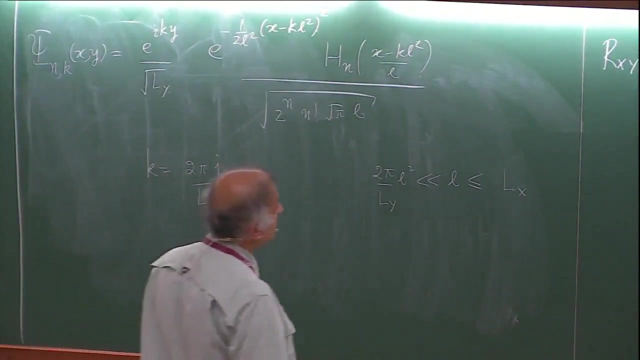 this is the smallest length scale. that's much, much less than L okay, which is much, much less than L X. this is generally true for almost any sample that you make in the lab, all right, so, basically, this wave function has already decayed to almost nothing by the time you come to the edges of the sample, and that is why. 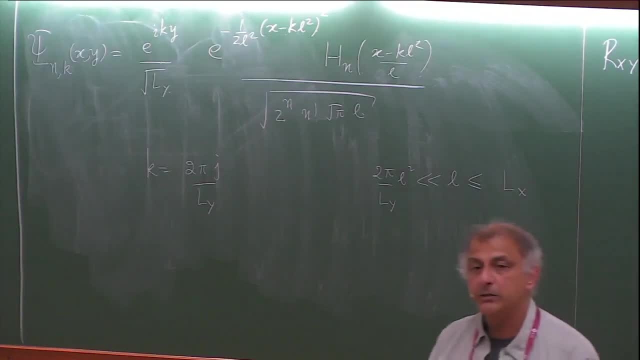 it actually doesn't matter that the sample is finite in length, as long as it's much larger than the magnetic length. yeah, all, right, now let's actually count the number of writing centers that fit into this particular ample. okay, so remember, the separation between each of these successive ones is two pi over L? Y. 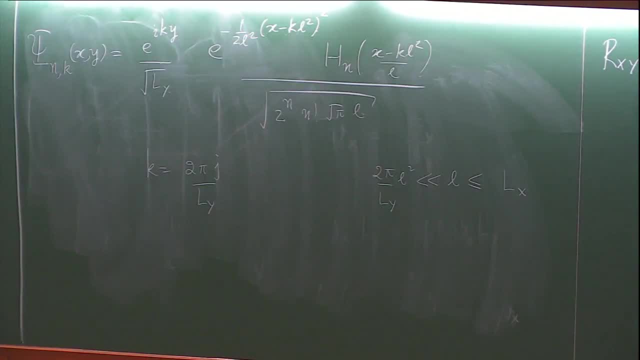 times little L squared, and you have to cover a distance of L- X. so therefore, the degeneracy of this Landau level, a number of these guiding centers, is just going to be this value, right, and what is that? there are a number of different ways of writing this. so first, 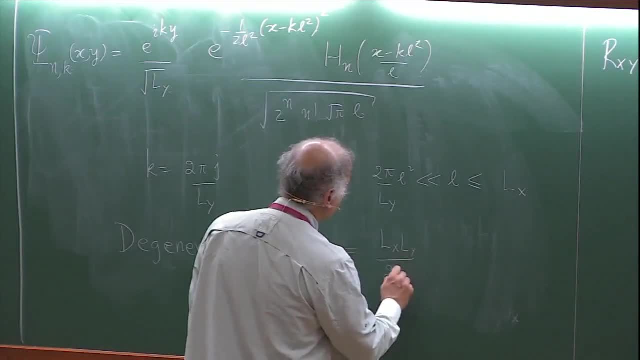 let me write it as L, X, L Y divided by 2 pi L squared. then I'll expand out the 2 pi L squared. so L squared, remember, is h bar over e B. so I will rewrite this as B times L, x times C, L y. so I'll re-write this as B times L, x times C, L y. so I've now got 2 pi L squared, so you can now reride this as B times L, X times C, L squared. this is this. 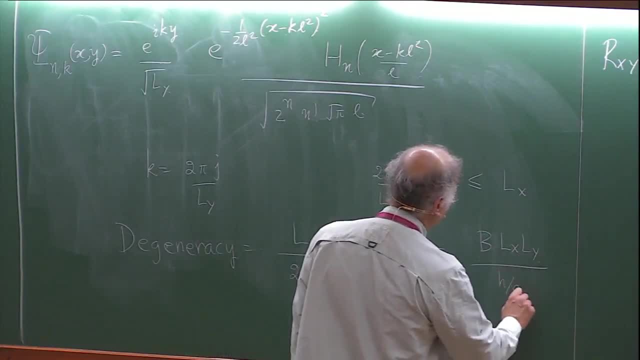 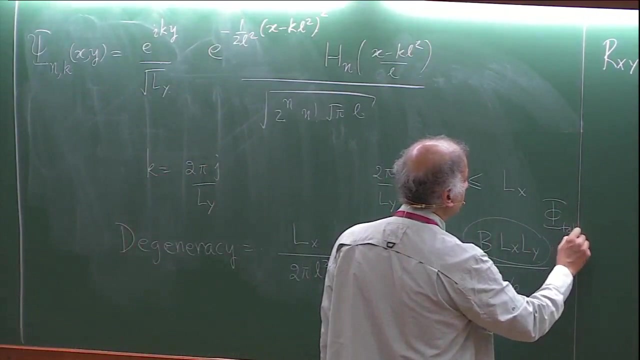 L, Y divided by H over E. Okay, let me write it like that: 2 pi H power is H. okay, This, the numerator here, is the total flux through the sample. The denominator is something known as the quantum unit of flux. 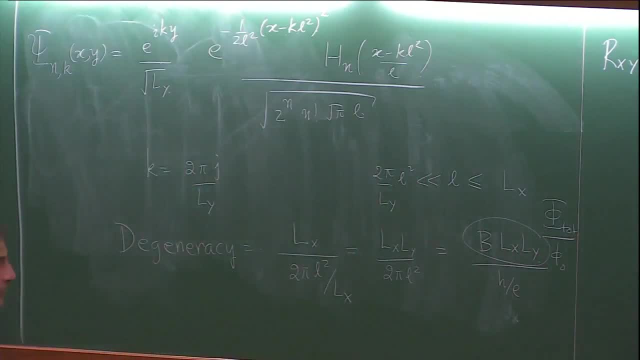 the flux quantum H over E. okay, So this basically says that the number of states that are sitting inside your sample are equal to the total number of flux quanta that are going through the sample. You have to be a little bit careful. 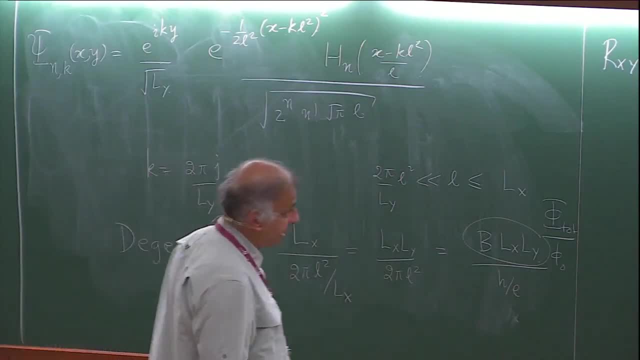 The flux is actually not quantized. okay, The flux is just produced by some magnet. Okay, the total amount of flux in your sample need not be an integer. There is no sense in which the flux is bunching up in this material. 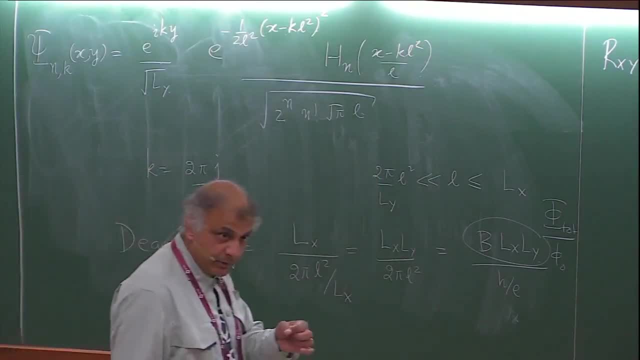 In the normal metal the flux doesn't bunch up into anything quantized. There are certain materials, like superconductors, where they do bunch up, but not here, okay. Okay, so this is just a way of counting, okay. 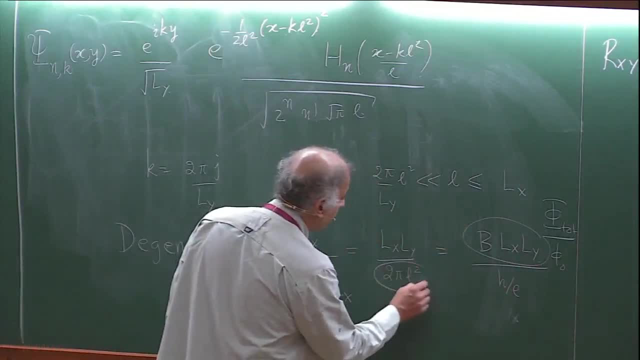 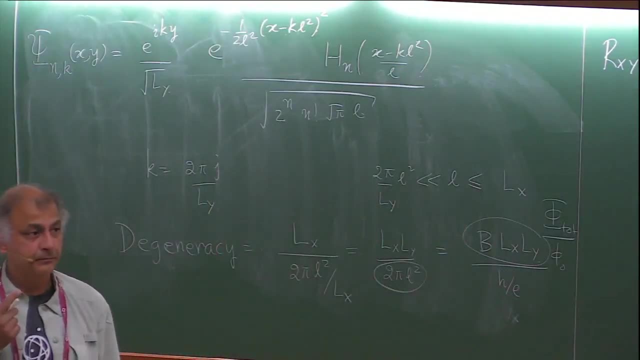 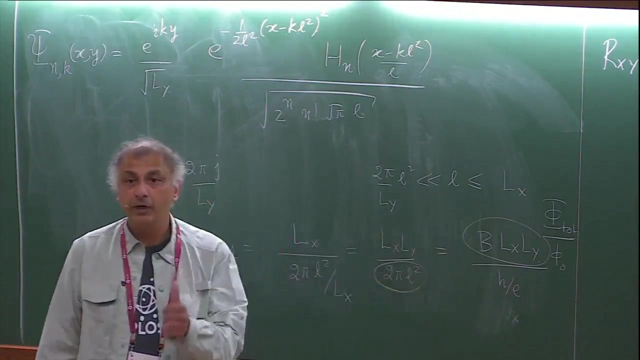 Another way to think about it is that 2 pi L squared is basically the area through which one flux quantum passes. That's another way to think about it. okay, So it says there's the total area divided by the area through which a flux quantum passes. 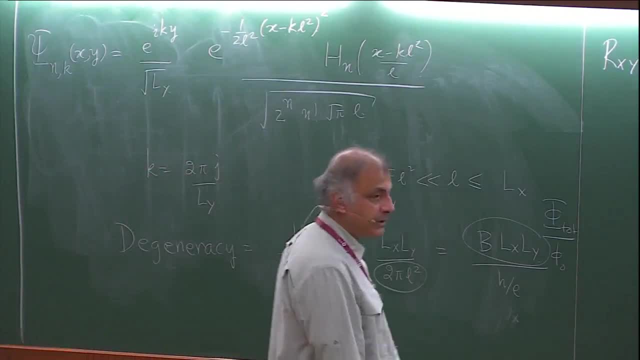 Those are the two different ways of thinking about it. They're actually the same way. Okay, so this is the degeneracy. This is the degeneracy of a land-down level. Okay, Good Questions, All right, So now let's go to the gauge argument. 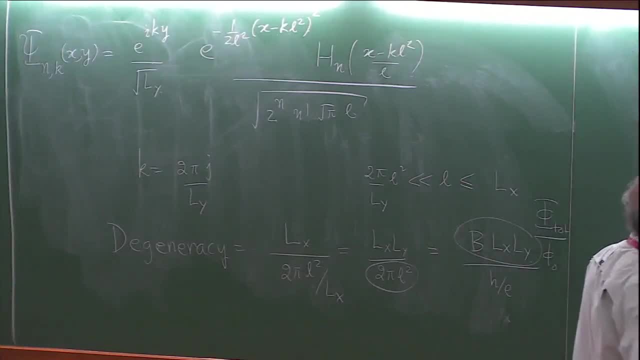 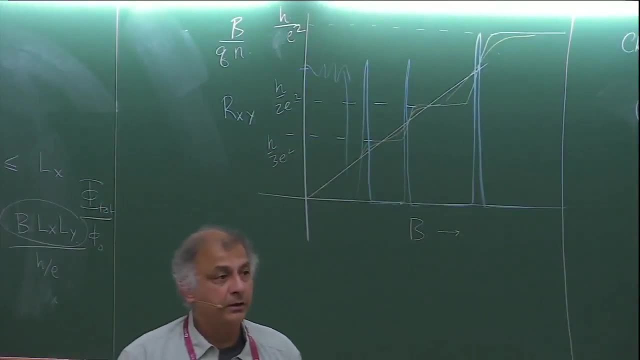 So the real question. of course, somebody asked me right here that the straight line is really supposed to be the correct answer. for a very clean sample or a sample with no disorder, that should be the answer: at all temperatures. Okay, that is true. 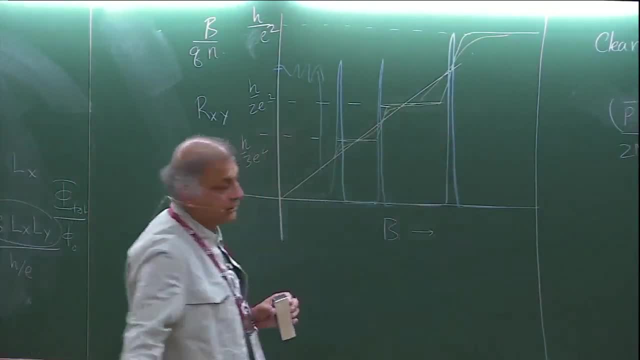 However, what is seen is these steps. So the question is: what is it that accounts for the quantization of either the Hall resistance or the Hall conductivity? Okay, what is it that accounts for that And that has to do with disorder? 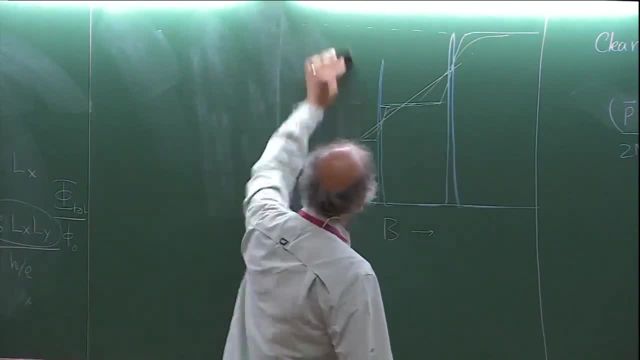 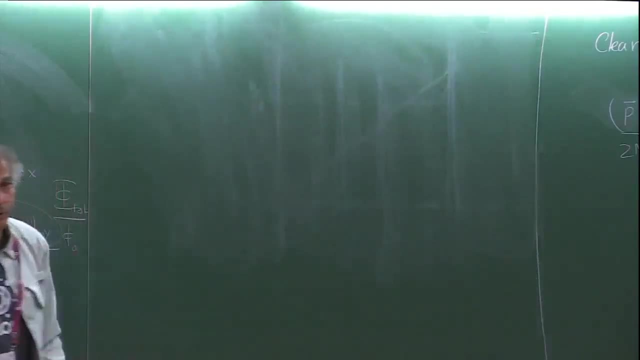 Okay. so to work up to disorder, let me first give you this gauge argument in a clean sample, Then I'll give you the gauge argument in a dirty sample, And finally I'll give you one simple view of what's actually going on. 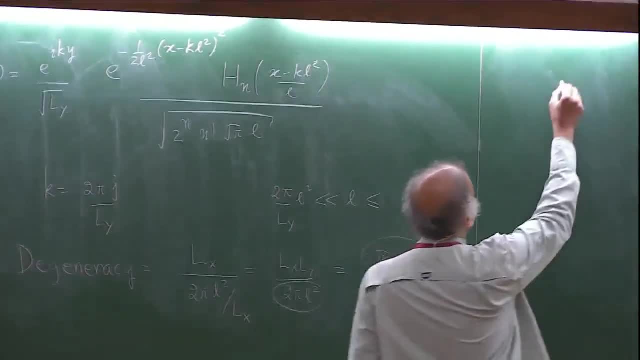 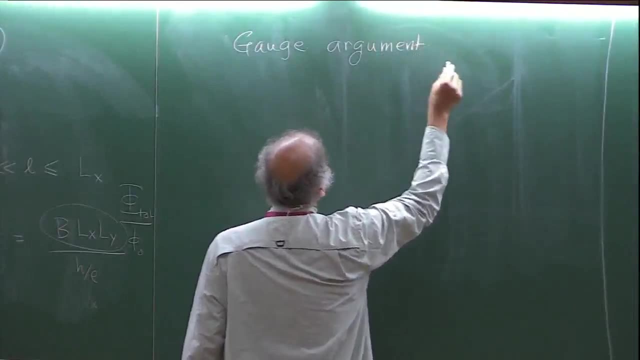 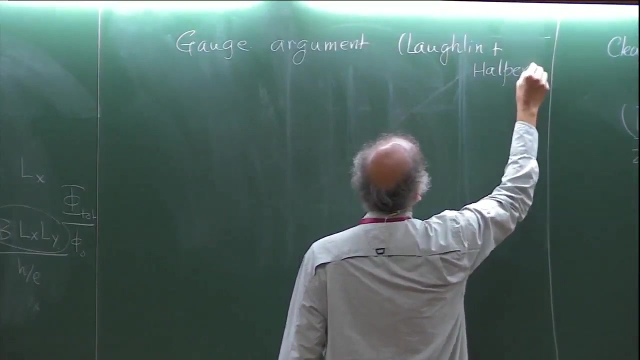 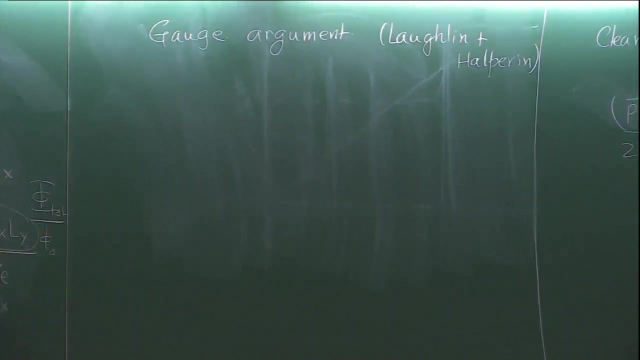 in the presence of disorder. Okay, This, by the way, is due to Laughlin and Halpern, All right, so here's how it goes. So I'm going to take that clean sheet and I'm going to roll it up in cylinder. 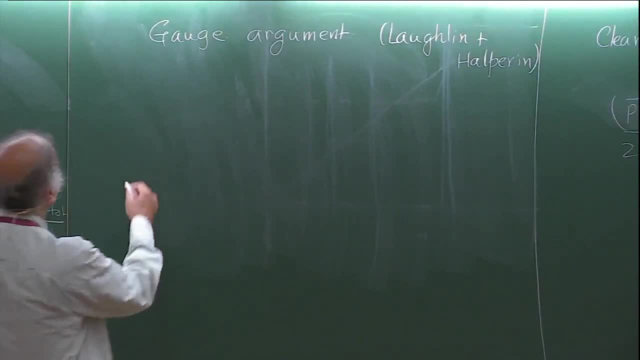 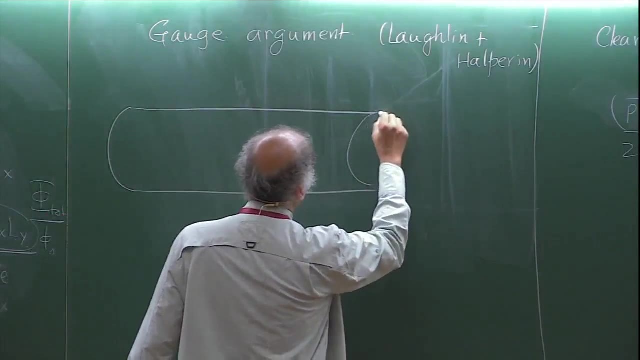 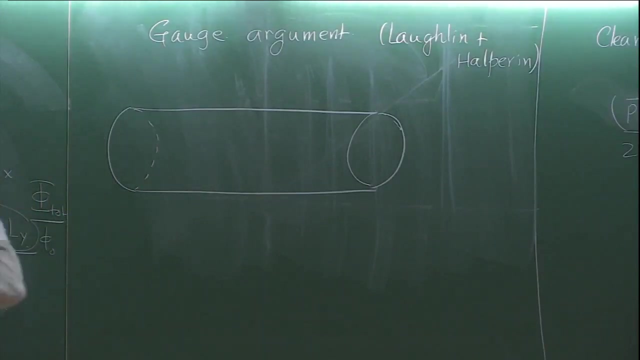 The way I promised. Okay, Now let me write it as a cylinder. So here it is, All right Now on the cylinder. the circumference of the cylinder is going to be Ly, Right, Okay, And then there are going to be. 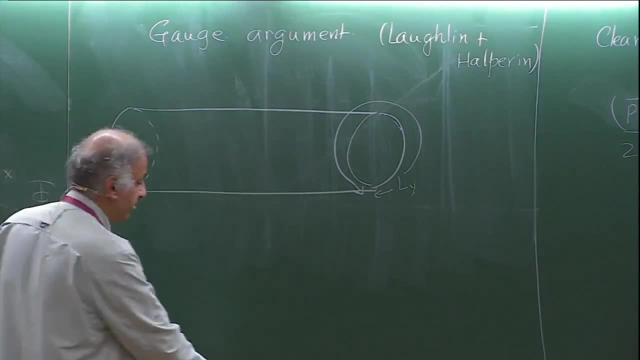 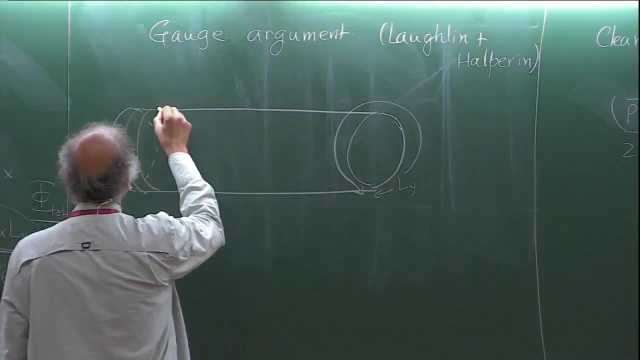 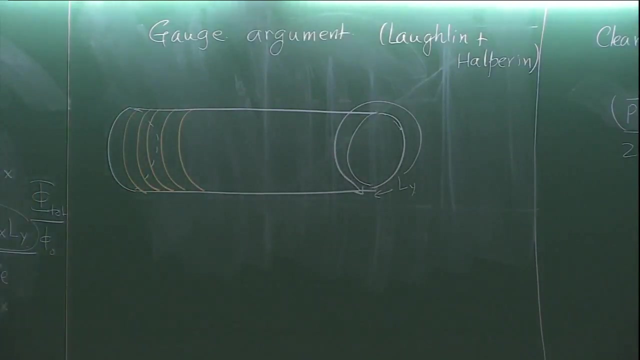 these Landau guiding centers that are spread out. They're going to be spread evenly along the length of the cylinder, So let me draw a few of them So it looks something like this: Okay, Good, So far, it's exactly the same. 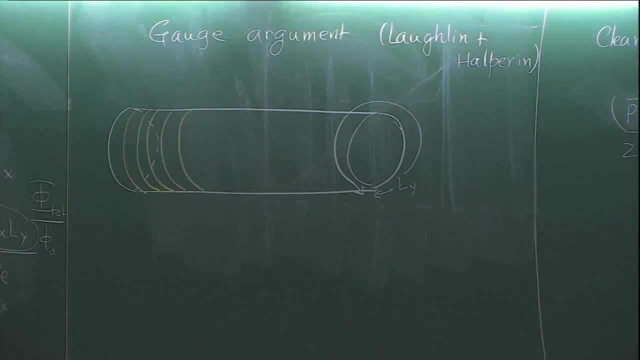 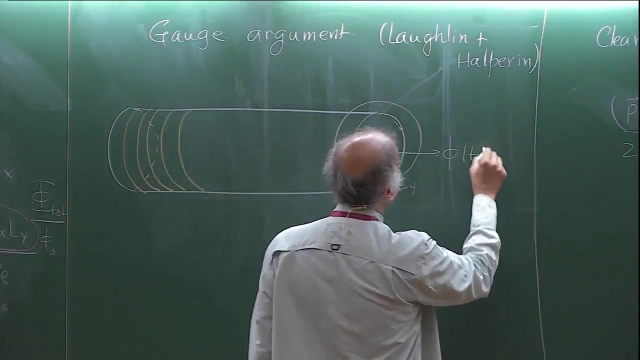 as what we had over there. Now I'm going to do something a little bit different. I'm going to put a flux through the hole of the cylinder, through the hollow axis of the cylinder, Okay, And this flux is going to be changing with time. 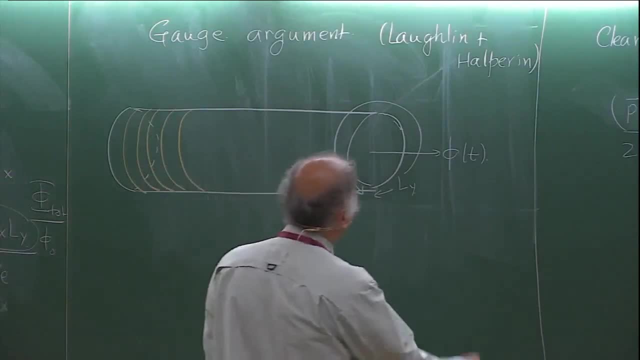 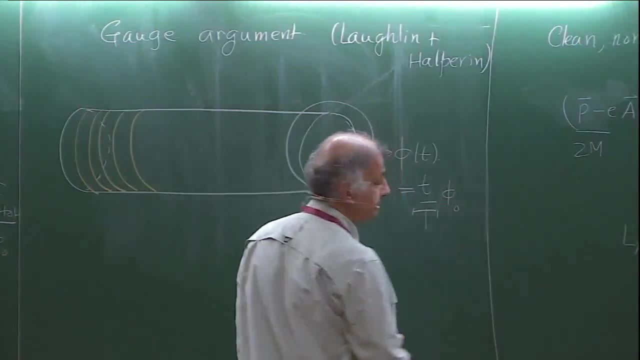 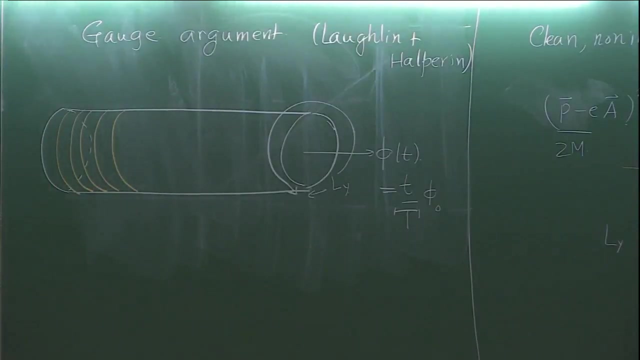 This flux is going to be arranged in such a way that at the end of some time, which I will call capital T, it will equal one flux quantum, And you will see the importance of this being one flux quantum in a little bit. Okay, So I'm going to arrange. 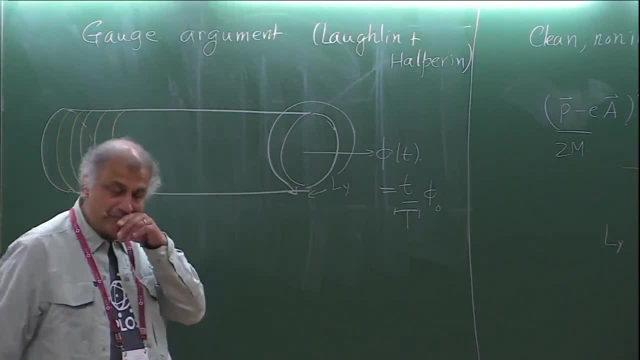 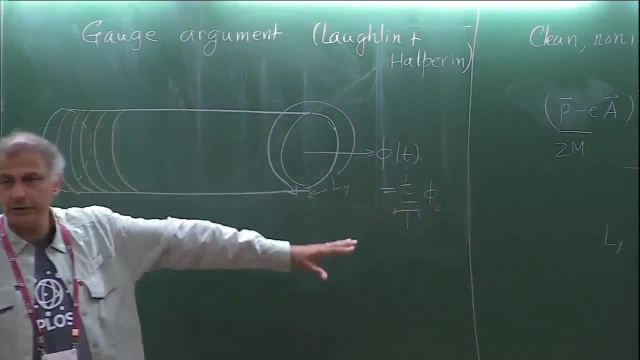 for it to be like this. So what's the whole idea? So the idea is that I'm going to solve for this system. I'm going to do a very slight generalization of what we already did. It's going to be very similar to what we did. 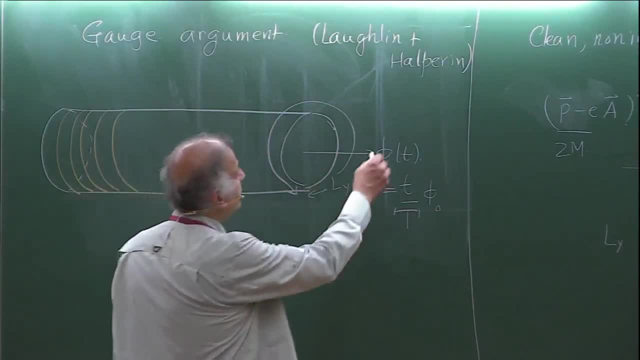 except for one little bit, And then we're going to treat this phi as an adiabatic parameter. Okay, So remember, this flux is being changed very, very, very slowly. Okay, So, as this flux changes slowly, the adiabatic theorem says that: 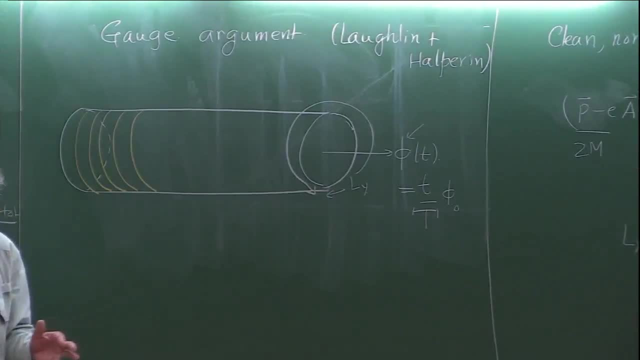 if particles were occupied in certain states, then as you change that parameter, those states that are occupied continue to be occupied. Okay, And we will see that. what's going to happen is that, as you change this phi from zero to one flux quantum, each of these individual 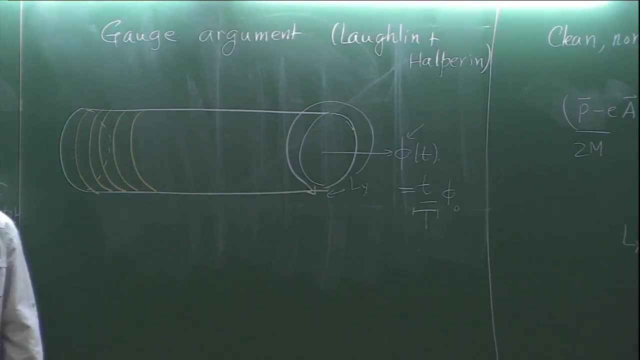 guiding centers will move to the next one. Yeah, So in that case the magnetic field is perpendicular to the plane of the, Correct. But in this case, when we consider the flux through the hollow, is it perpendicular to the? That's correct. 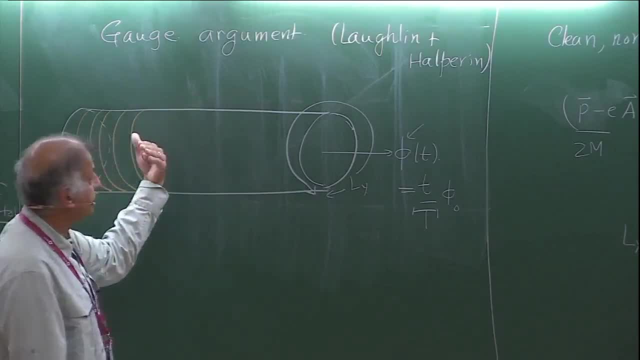 So the idea is that there is a perpendicular magnetic field on this sheet, So there's something that's coming radially outward from the axis of the cylinder. That is a constant magnetic field. I'm not changing that, Okay, In addition to that constant magnetic field, 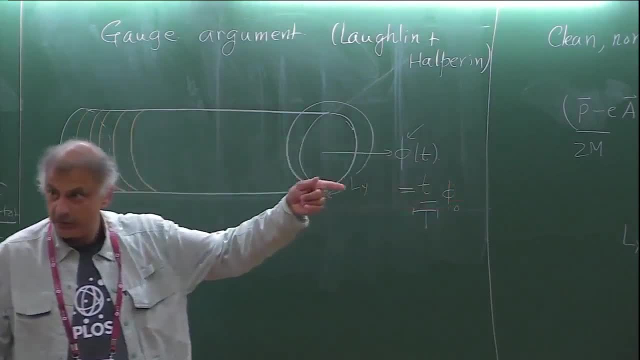 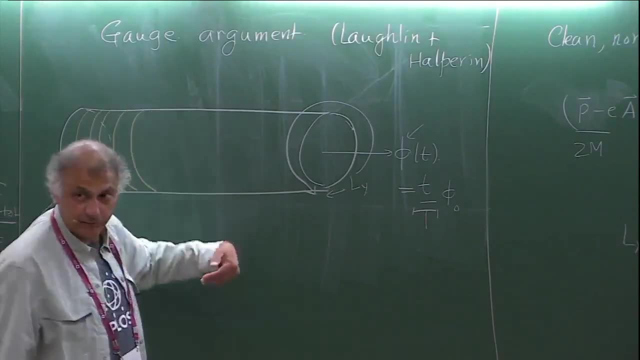 I'm imposing another flux that goes through this, the hollow of the cylinder Right. It's not producing any magnetic field on the surface of the cylinder, Okay Okay, It's a solenoidal flux. So imagine I put a very thin solenoid. 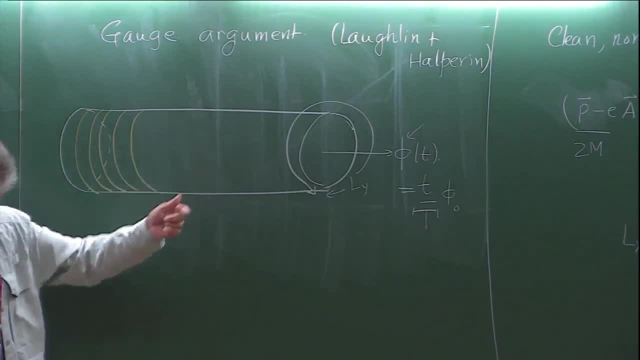 inside the cylinder Right And I change the current in that solenoid very, very slowly. That's what I'm doing. Okay, It's not producing a magnetic field. In fact, it's supposedly not doing anything. Of course it's doing something. 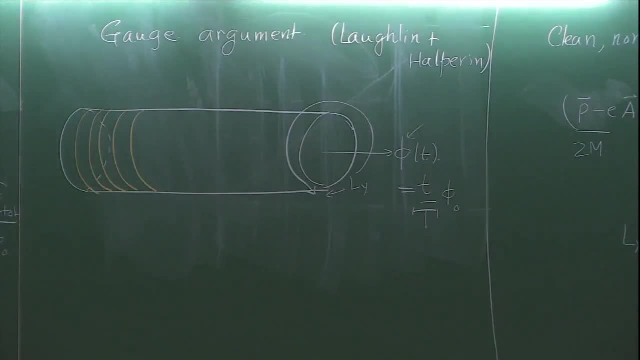 Otherwise I wouldn't put it here. Okay, So that's a constant magnetic field through the surface. Okay, You're asking: how would they ever do this experiment? No, I'm asking that if I want to change the flux of the hollow, 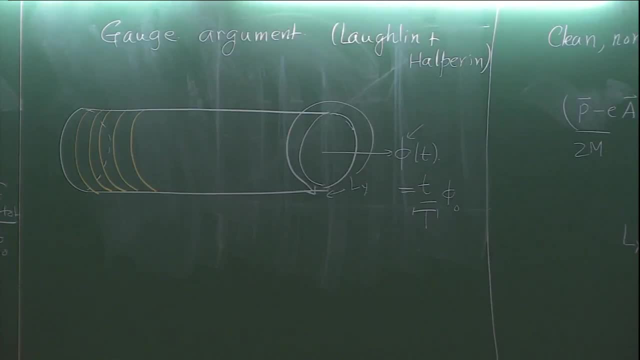 so it needs that the current in these rings of the solenoid should change. That is not the solenoid, by the way. That is the actual quantum Hall sample, Right. The solenoid itself is some very, very thin thing here. 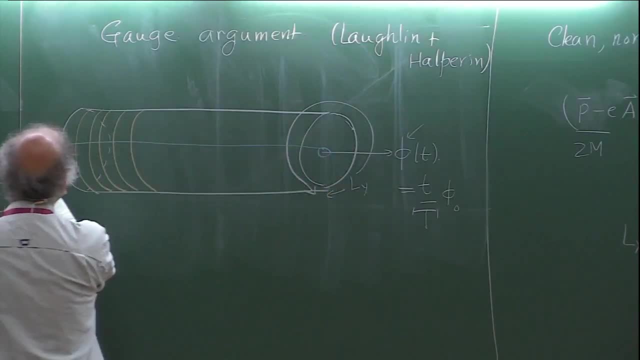 Okay, There's some very thin solenoid that's going through here. Okay, I'm putting a current through. that Understood, All right? Good, You should ask me all these questions, Otherwise you will completely misunderstand what I'm saying. 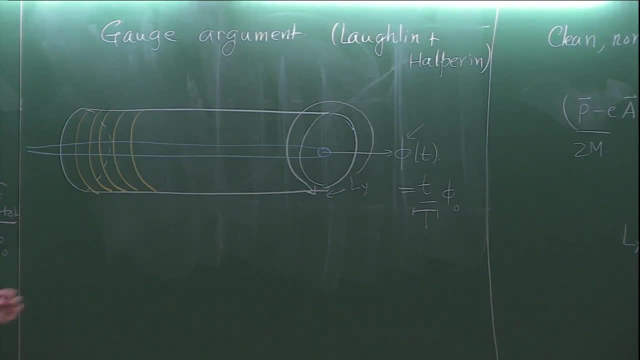 Other questions. So everybody gets what I'm doing right. I'm putting a very tiny, very thin solenoid through here and I'm changing the flux through that solenoid, Okay, Good, So I'm going to solve this problem. 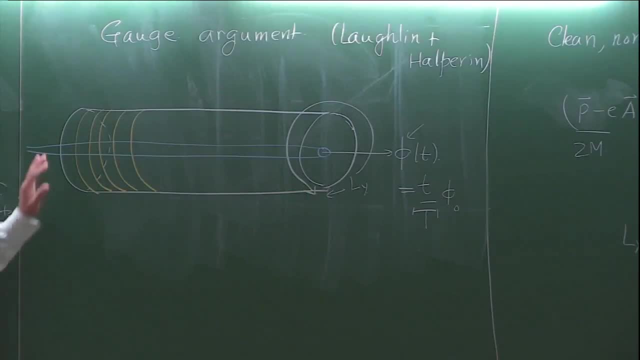 like I said. So here's the broad picture of what is going to happen. So I'm going to solve this problem. for fixed values of phi, I'm going to treat phi as an adiabatic parameter, And you will see that at the end of the day. 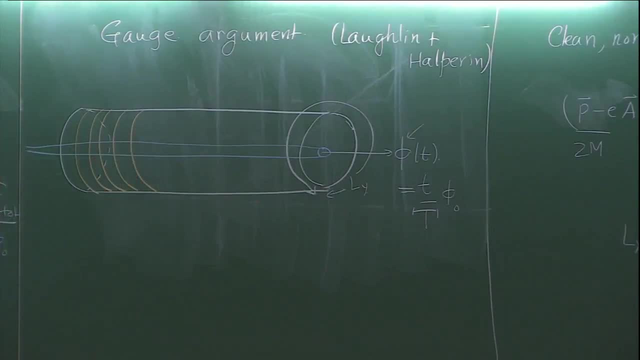 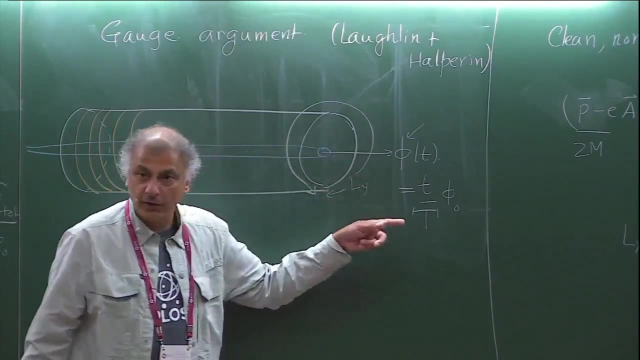 when phi changes from zero to one flux quantum, each of these guiding centers moves on to the next one. Okay, Then I'm going to use Faraday's law to solve this problem. So in the same varying flux, it produces a circulating electric field. 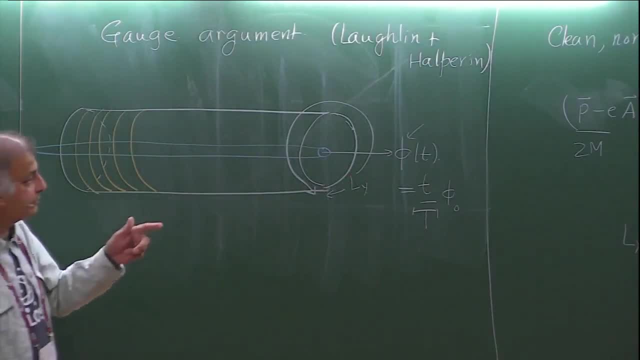 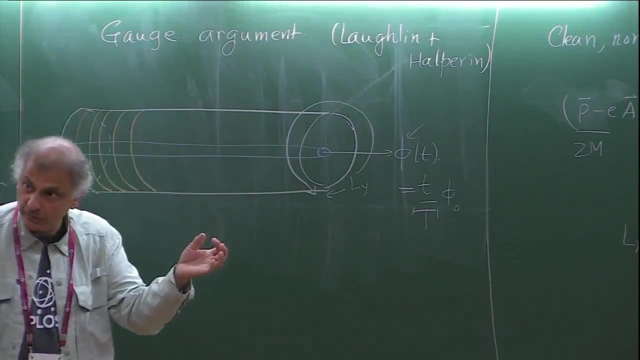 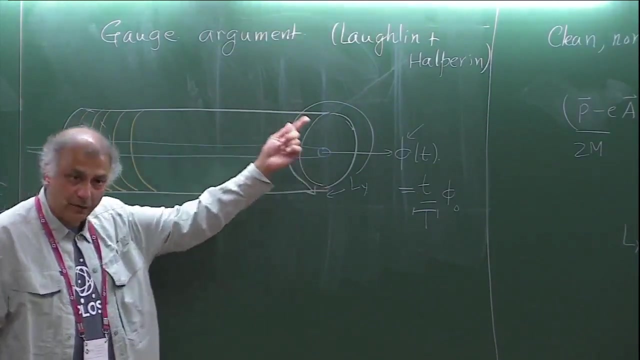 in the y direction Right. But that circulating electric field in the y direction has the response that electrons move through the separation between two successive guiding centers. That will tell you the current. So there will be a relation then between the electric field in the y direction. 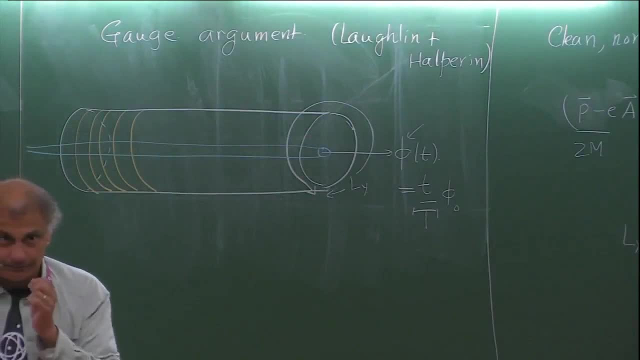 and the current density in the x direction, And that exactly is sigma xy. Okay, So this is just the warm up, because this is the clean system. After that, I'm going to go to the dirty system and show you how this generalizes there. 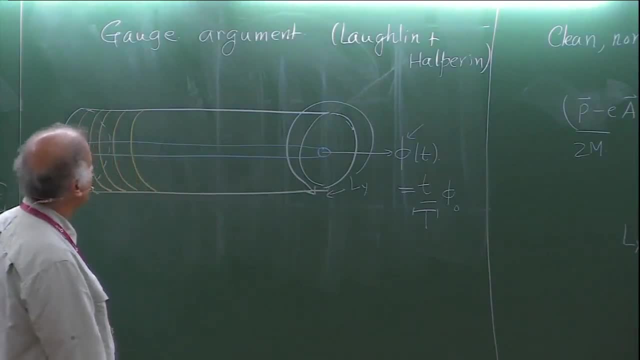 Okay, Good, Alright. So first step is to solve this problem in the presence of some arbitrary phi. Okay, Actually, it's very simple. All you need to do is: whenever there's a phi like this, how do I take account of that? 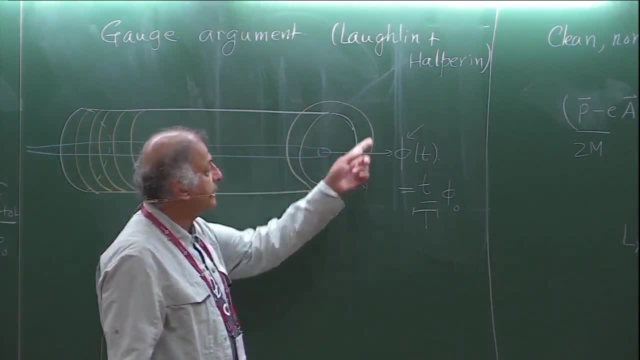 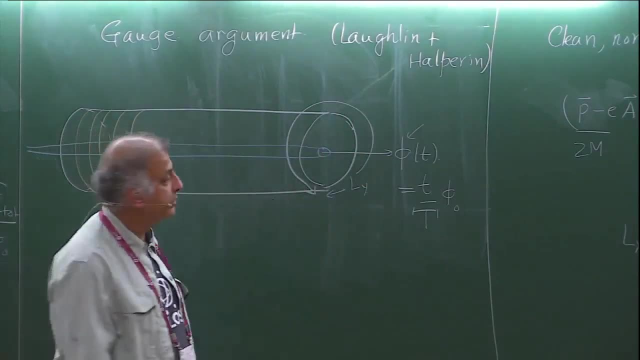 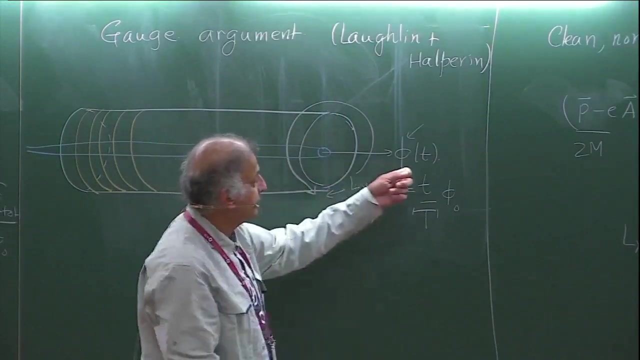 I can make a gauge field that exists in the y direction, Okay, Which integrates to phi, Right, Because I know that the line integral of the gauge field around that circumference, the extra gauge field due to this phi, should be equal to phi itself. 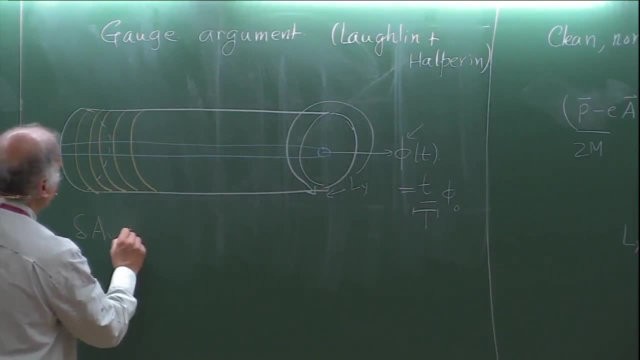 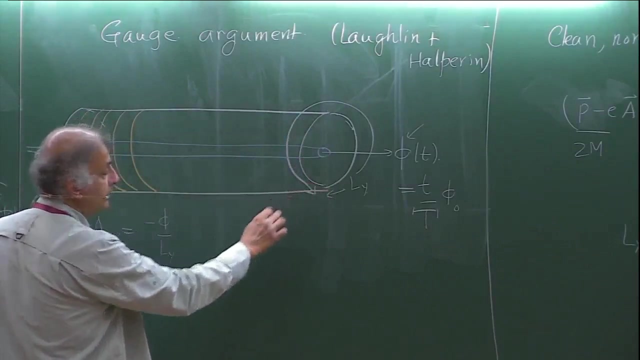 So therefore I say that the delta ay, due to this phi should be exactly phi divided by ry. You guys agree with that? Okay, There's a minus sign because I have chosen the l to go in that direction, but really I should do the line integral. 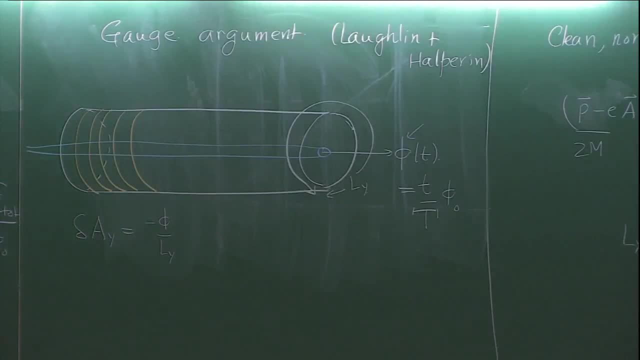 in the other direction. Okay, But up to a sign. that's what it is. Alright, We already know what the ay was. It's bx. So all that happens now is bx minus this. Okay. So therefore the distribution goes through entirely as before. 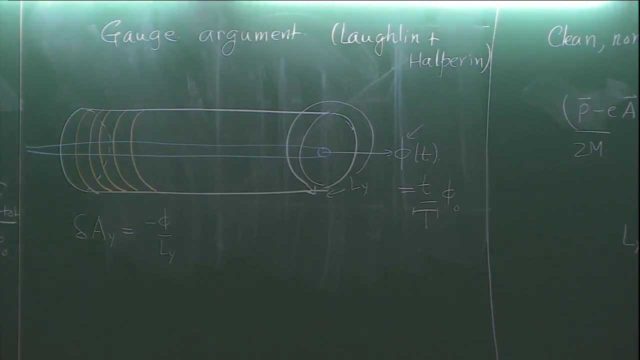 Once again, py is a conserved quantity, Right, It's e to the i ky times something, And therefore the Hamiltonian that comes out is going to look something like this. So let's not get confused between the capital phi, which is the wave function. 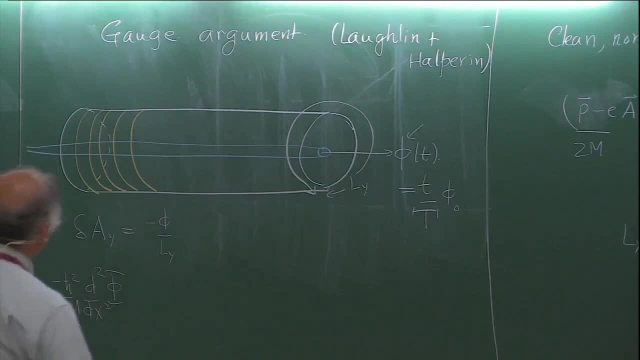 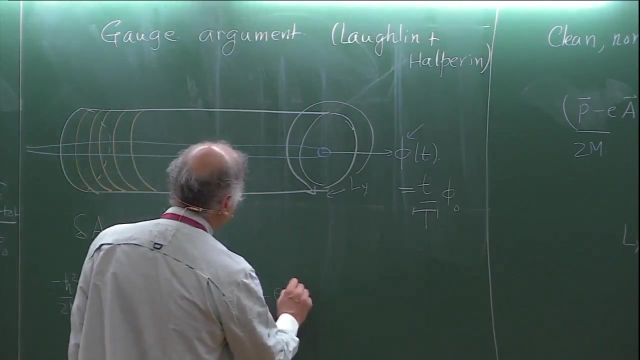 and the little phi which is the flux. Okay, So this is some phi sub k of x plus. so let's see what it looks like now. So the minus i h bar d by d ky was an h bar k minus e bx. everything here is as before. 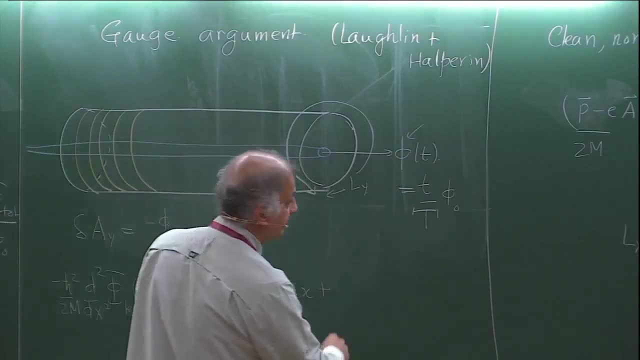 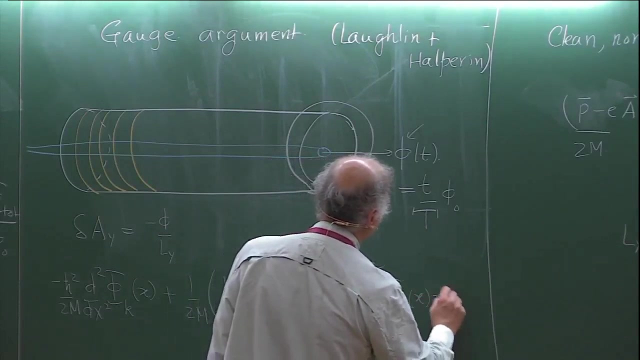 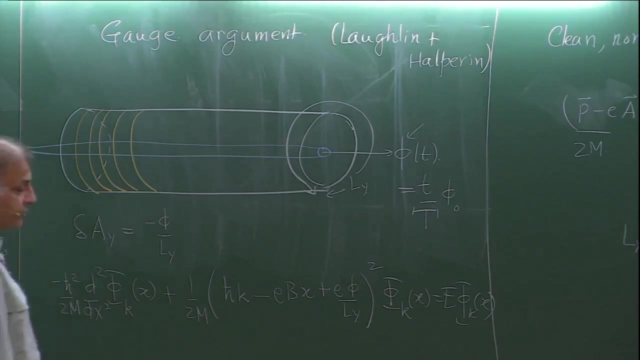 And then there's a plus. what is it? e phi, Right, That's really all it is. That's the only change that happens there, Correct, Okay. So what is the net effect of this change? The net effect of this change is to take k and shift it. 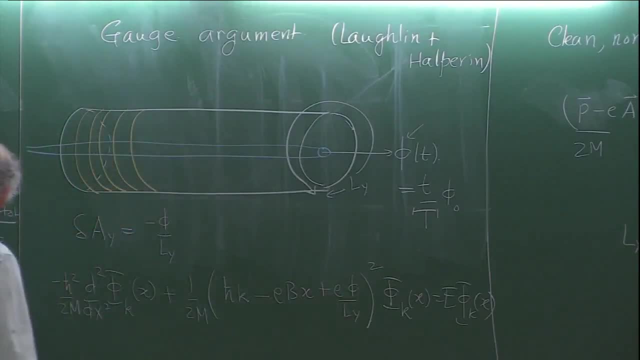 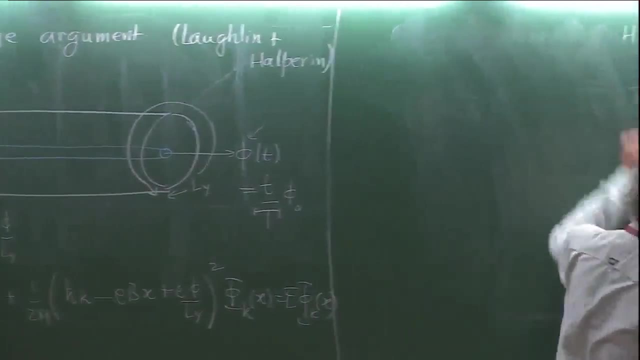 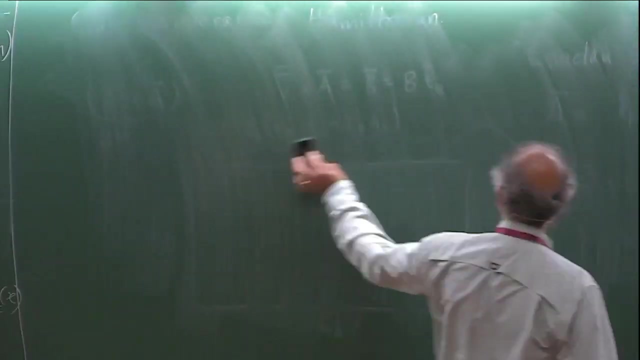 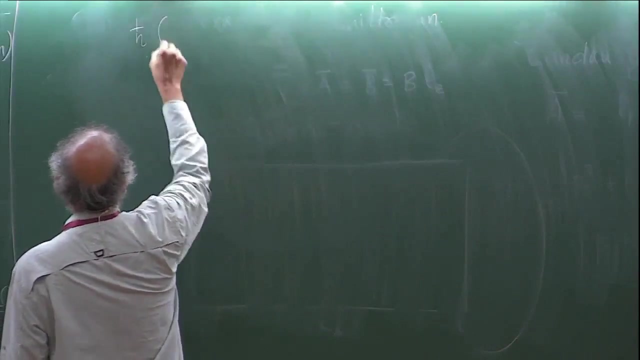 as something. Okay, What is that something? Let's see. By the way, Shubhra, how much time do I have left? Okay, Very little, Okay, Alright, Okay, so I will write this as h bar. 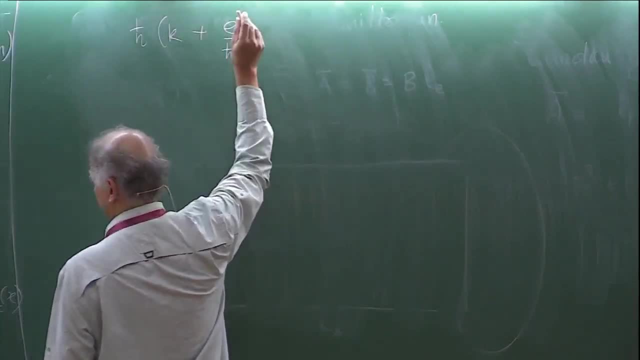 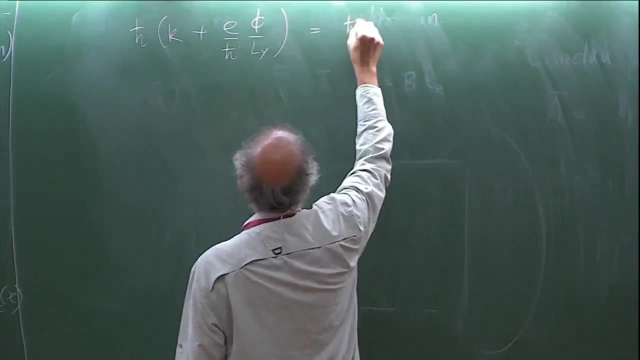 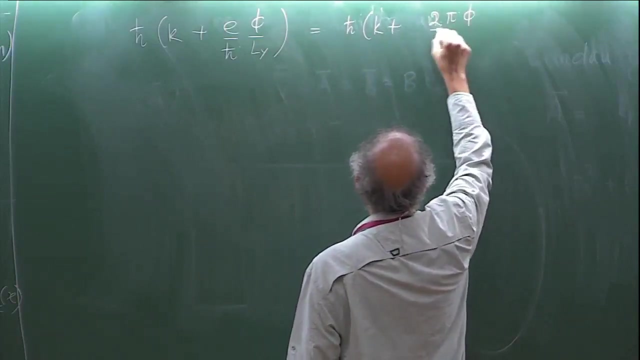 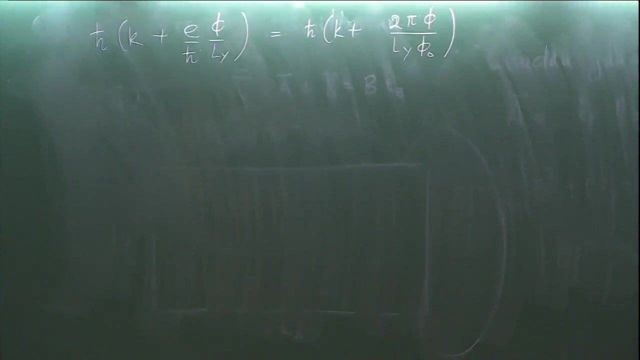 times k plus e over h bar phi ly. Okay, And this will be h bar k plus. Remember that phi naught is h over e. Okay, So that's what it looks like. So what does that mean? That means that when I 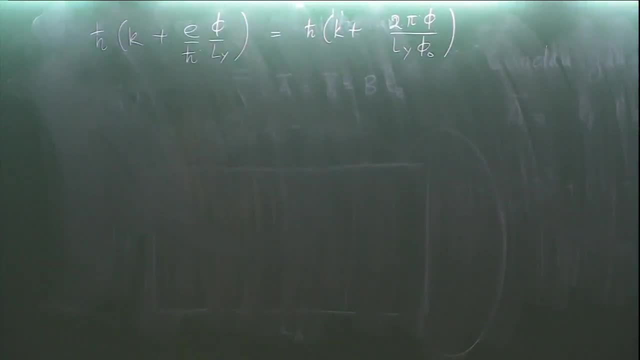 change the flux from zero to phi naught k shifts by an amount which is two pi over ly. But two pi over ly is exactly the separation of the two k values, two successive k values. Okay, This is the crucial point. So 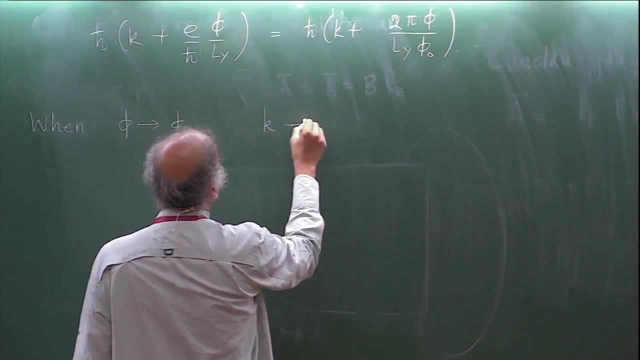 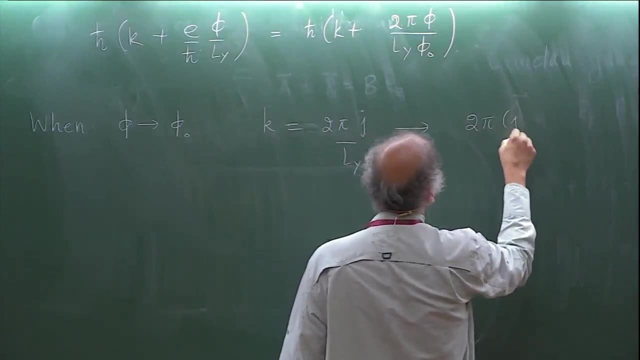 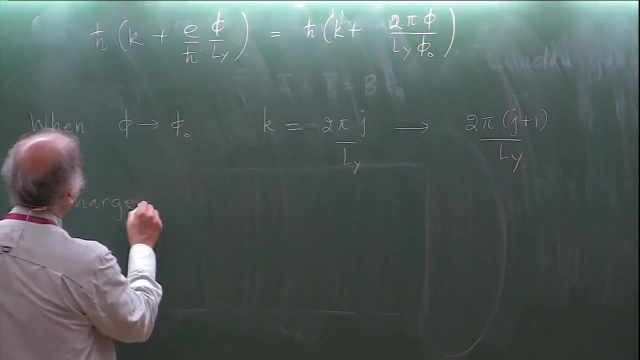 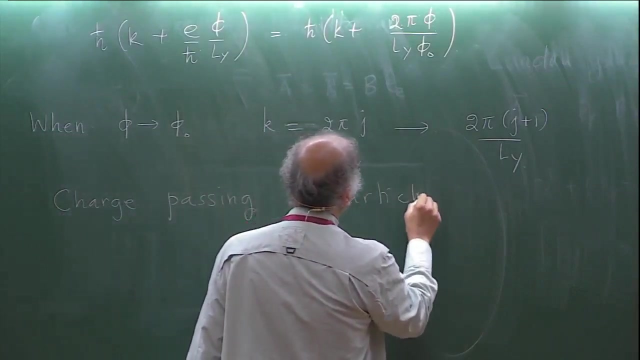 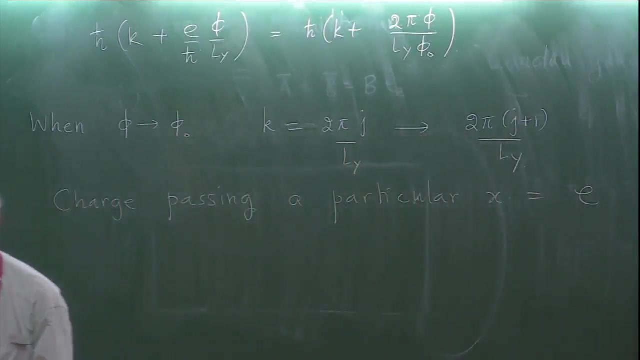 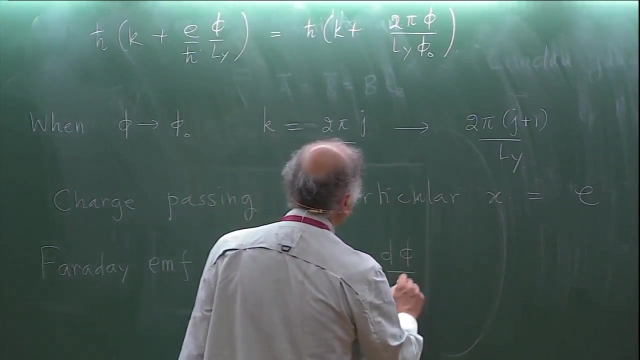 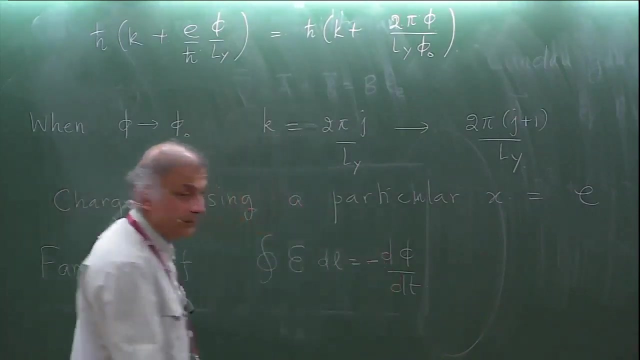 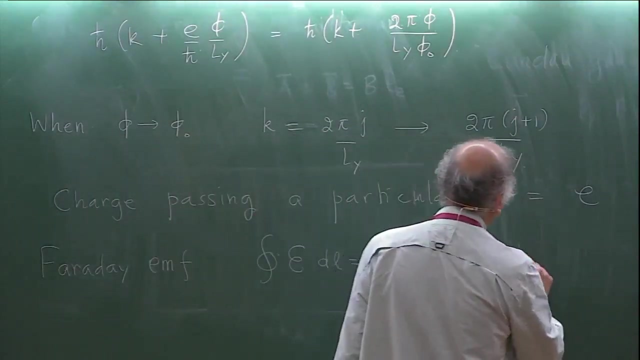 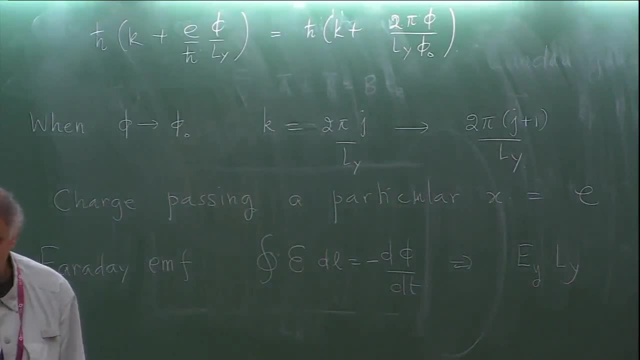 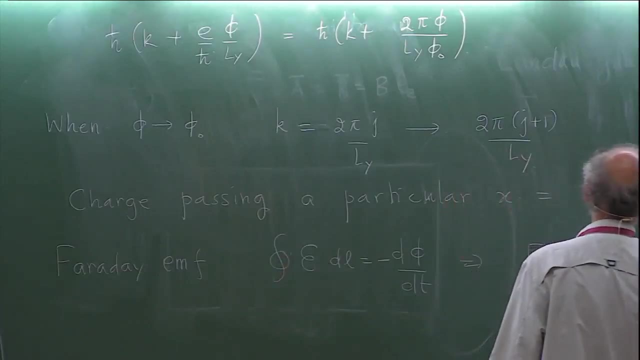 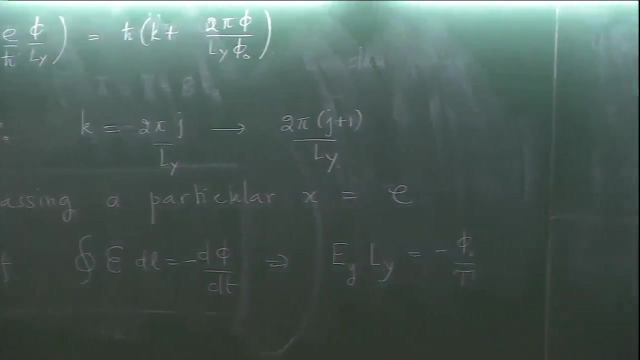 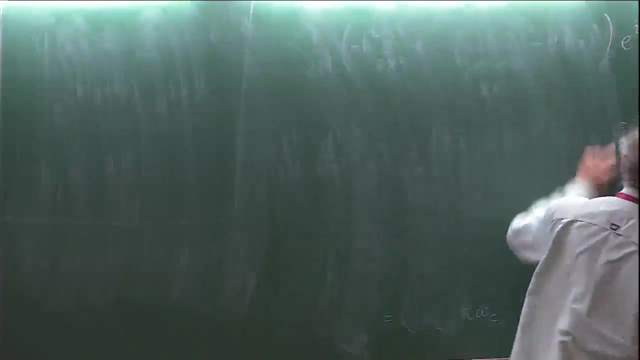 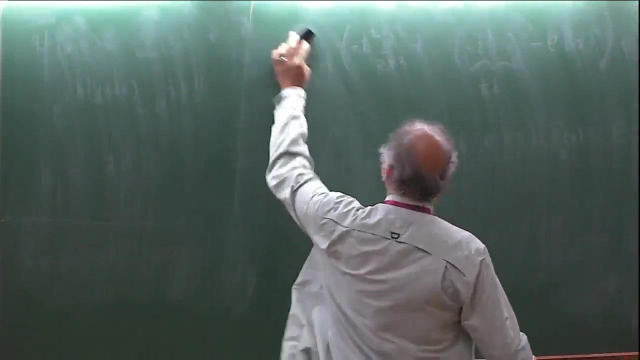 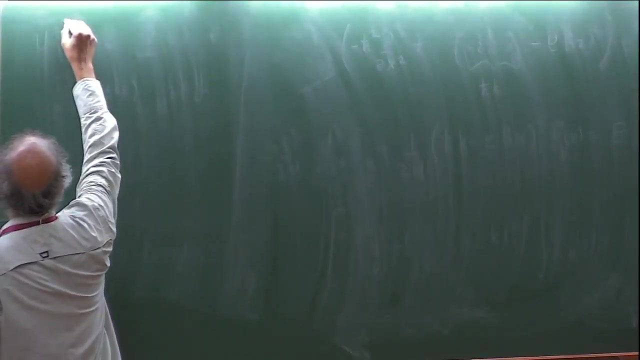 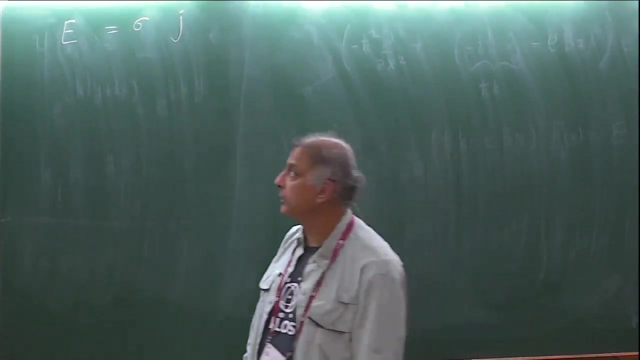 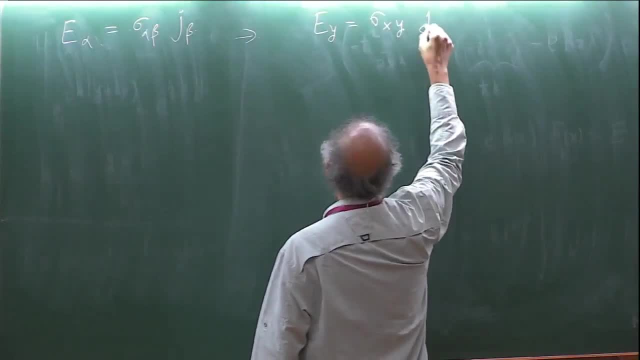 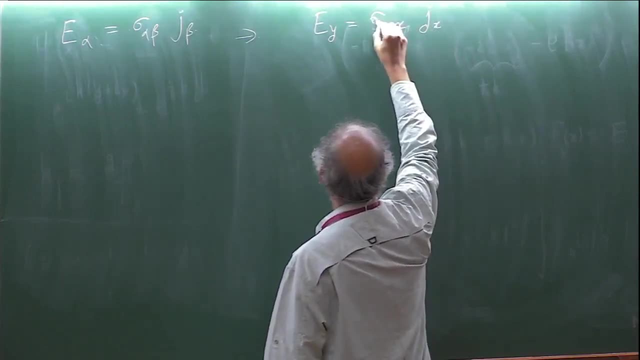 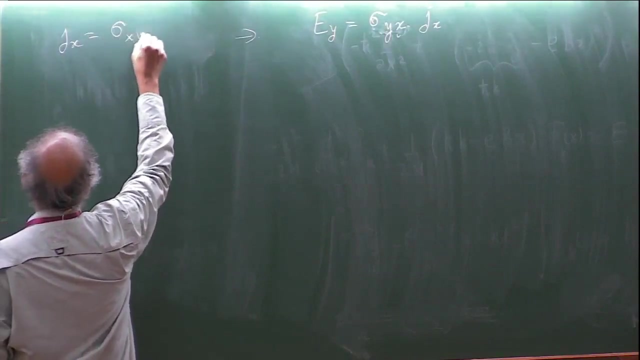 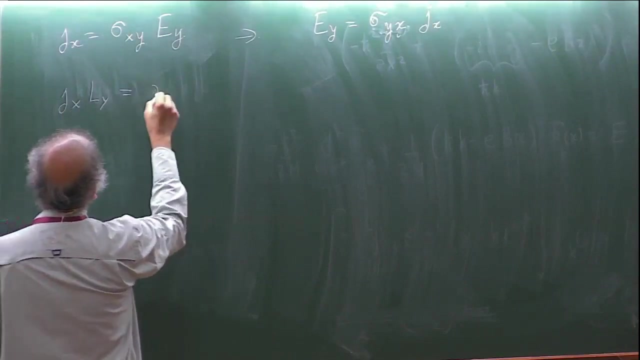 So let's see, Let me multiply this by y, So jxly is equal to sigma xy ey ly. 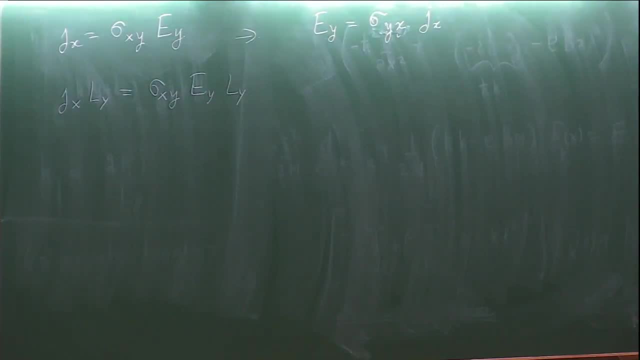 Why did I multiply this by ly? Because I want to get the total current in the x direction. So jx is the current density in the x direction. Again, for a two-dimensional sample, the total current is okay. I'm out of time. 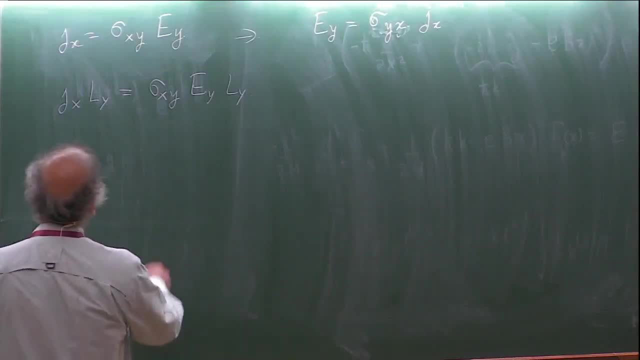 Okay, I'll speed up. Okay, I'll speed up considerably. All right, so this is the total current in the x direction, right? So this is ix. is sigma xy, ey ly. Very good, Ey ly, I already know what it is right. 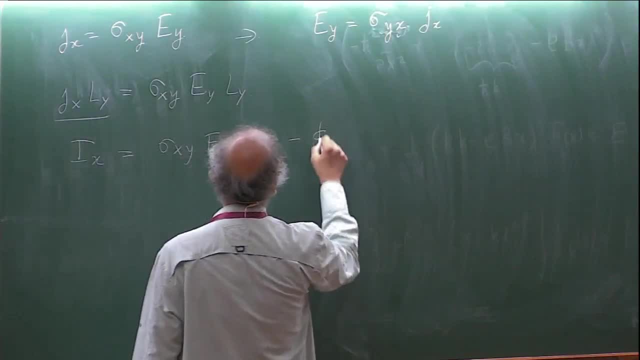 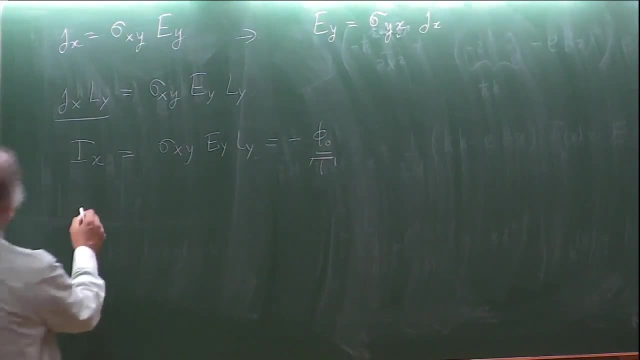 Phi naught over t. All right, I'm going to integrate this over the time between 0 and t. So integral 0 to t dt Ix. How much is that? That is the total charge that passes any particular point. 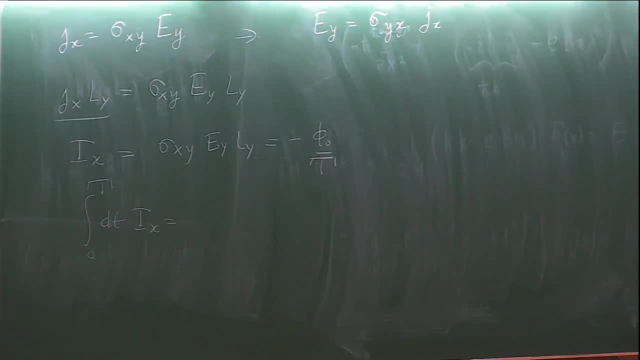 But the total charge we agreed was equal to one electronic charge if one Landau level was full. So this is just equal to e and that should be equal to sigma xy times. ey ly Sorry, this is Okay Okay. 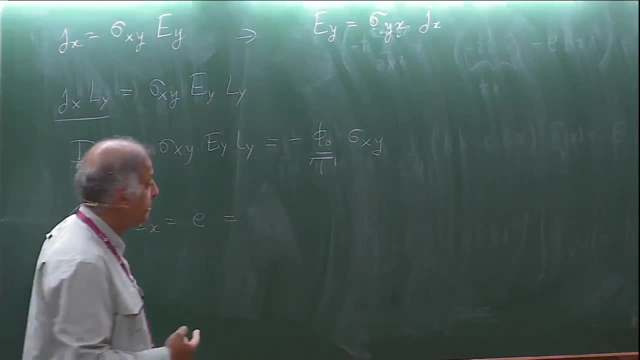 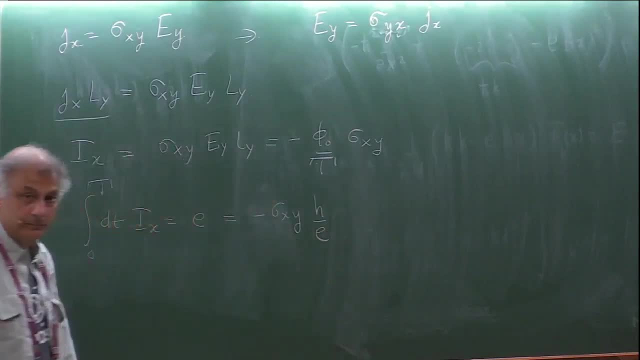 and then I'm going to write down: phi naught, That's h over t. Okay, So this tells you that, sigma xy, That's what it is. Now, if you had n Landau levels full, the total charge that has been transferred. 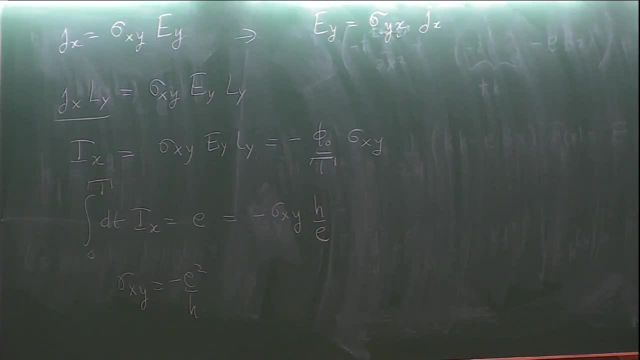 would have been n times an integer times e, Okay, And therefore the sigma xy would have been e squared, divided by n times h. Okay, Good, All right. So this tells you that this must be the Hall conductance for a clean system. 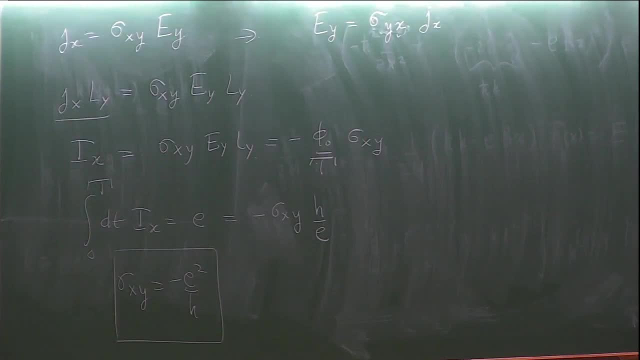 So, as I told you, this was just a warm-up. So what happens for a dirty system? All right, So here comes the argument. So there were lots of little orbitals here, right, These guiding centers were here. Let's imagine. 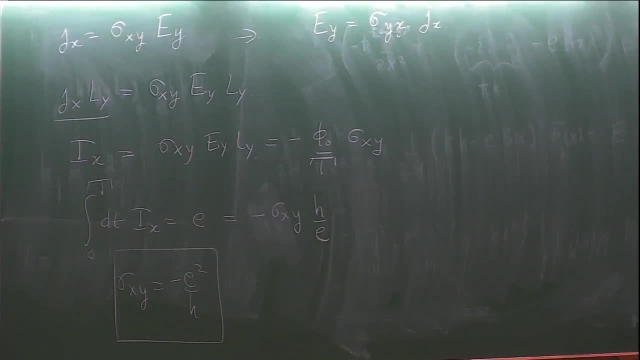 Question: yeah, So if we consider that n Landau levels are filled, so where does it change that? I missed that point. Sorry, I couldn't hear you. So if you consider, this is where that we have considered, one Landau level is filled here. 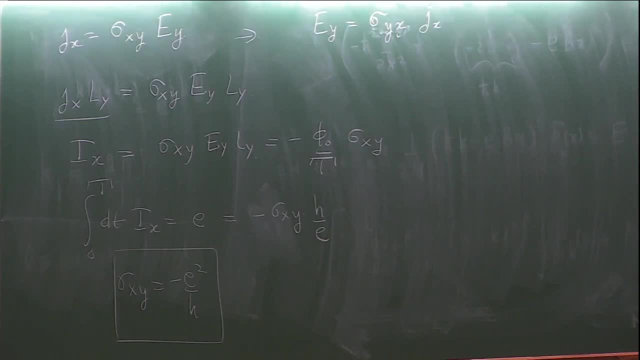 Yes, So if we consider, n Landau levels are filled. so where does it change actually here Here? So the total charge that passes a particular x is equal to this. This is the number of occupied Landau levels. Okay, Right. 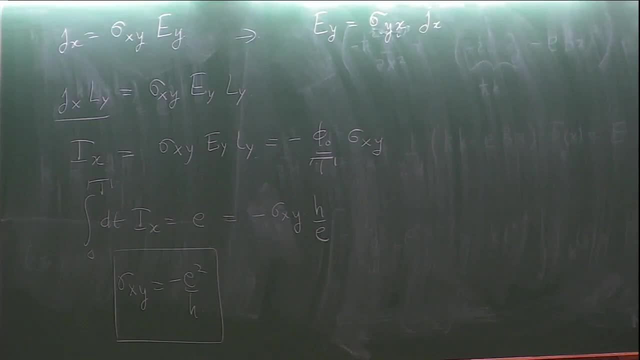 Because each Landau level will have its own set of guiding centers like this: Right, Okay, Okay, okay, okay, Right. So that's where it will change and this is where it will change here. Yeah, Okay, Yeah. 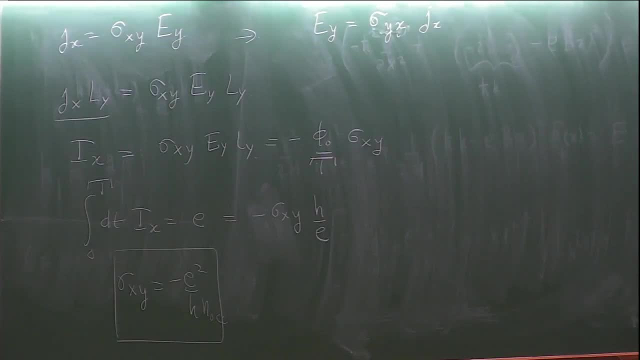 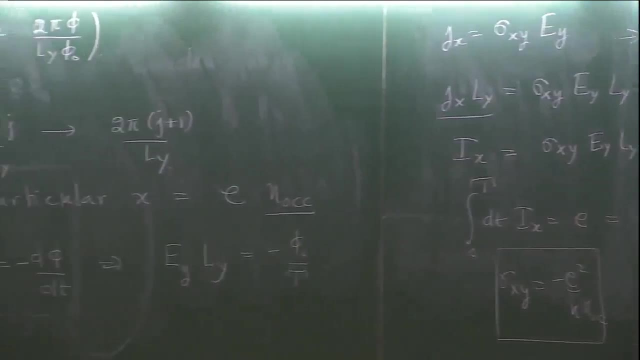 What happens at the boundary: Right, right, right, right, right. So I'm imagining that there is some contact that can feed electrons from the left and there's some other contact that can take away electrons from the right. So I'm assuming that that is happening. 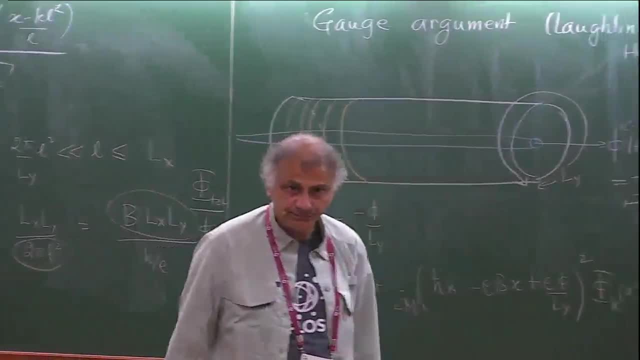 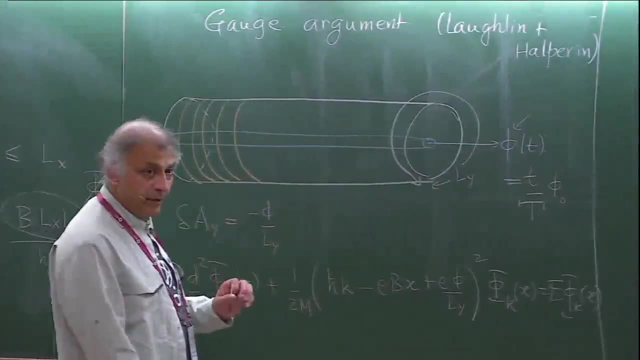 Okay, I'm sitting somewhere in the middle of the sample where all this is not important. Okay, All right, now we come to the disorder. So the argument goes as follows: So remember, there were some guiding centers here right Before you put in the disorder. 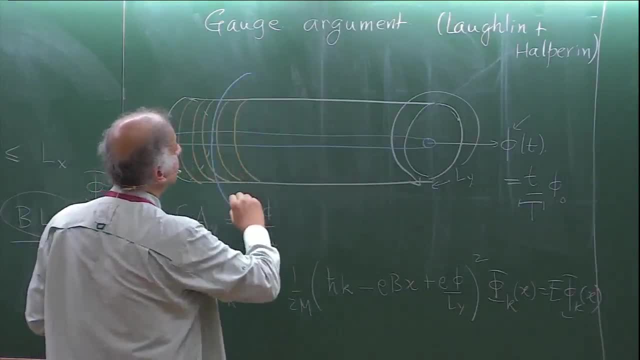 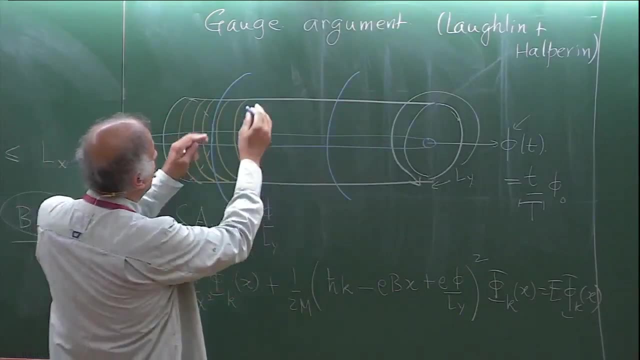 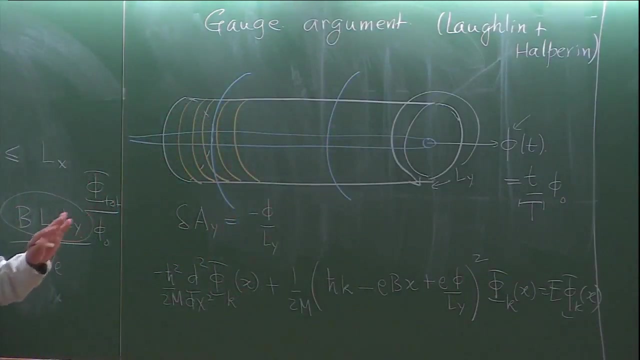 Let's imagine putting in the disorder only between here and here and leaving the rest of the system clean. Okay, So to first approximation. all the guiding centers that are sitting outside the disorder are not affected. It's not strictly true, but it's reasonably true. 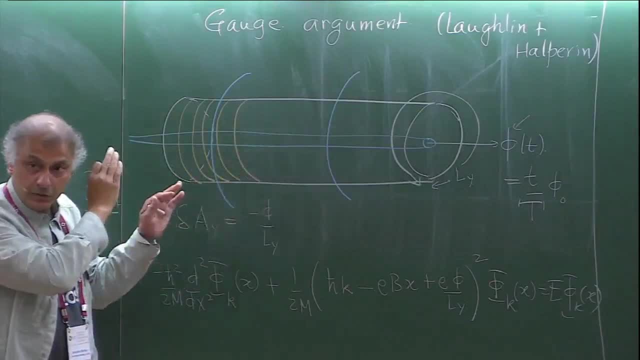 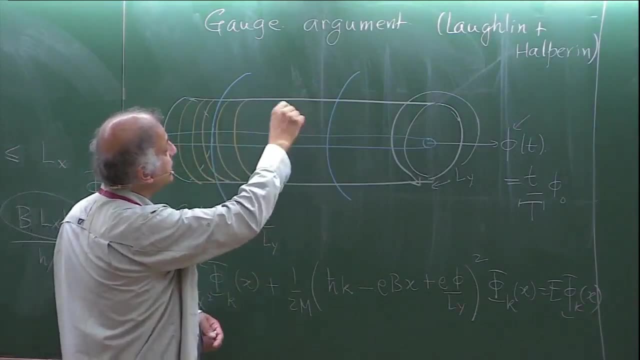 Because, remember, the wave functions decay with a Gaussian as you go away from this guiding center center, right, Okay, so all these guiding centers that are here will get mixed up by the disorder, They will get scrambled and there will be some superpositions. 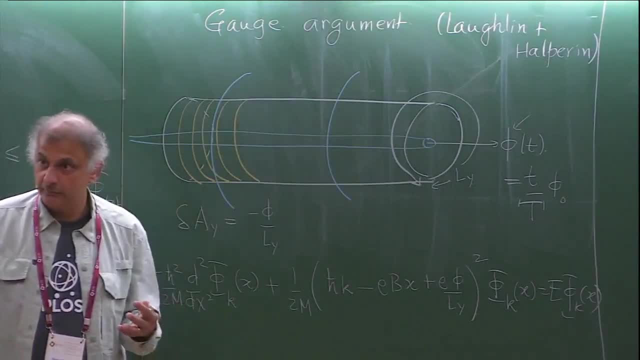 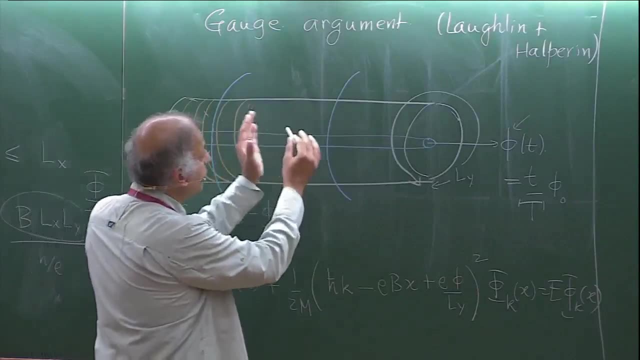 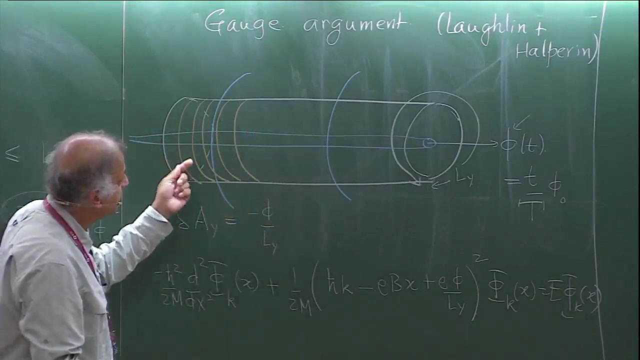 some new superpositions, which will be the true eigenstates. Okay, But the key point is that, remember, those superpositions are made out of these old guiding center orbitals, So therefore, as I change the flux, each of them goes to its next partner, right? 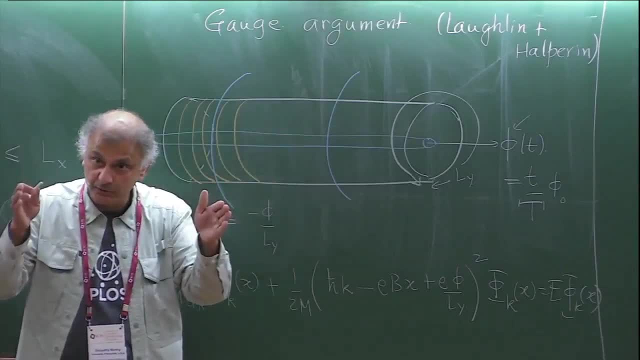 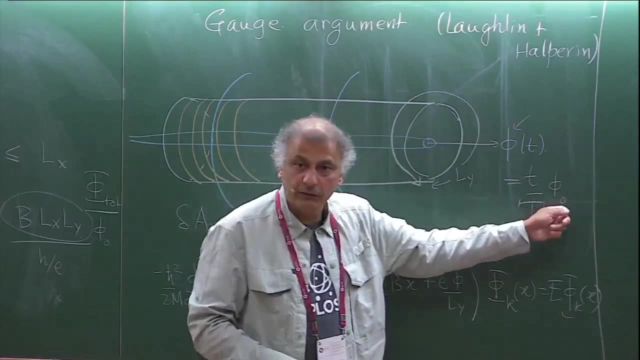 So the same thing should happen inside here. If I look in the superposition that's formed by the disorder, each guiding center should move to the next one. By the time I'm done, putting one full flux quantum, the situation looks exactly the same as before. 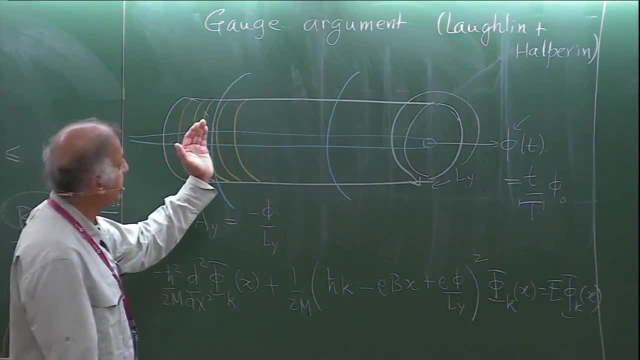 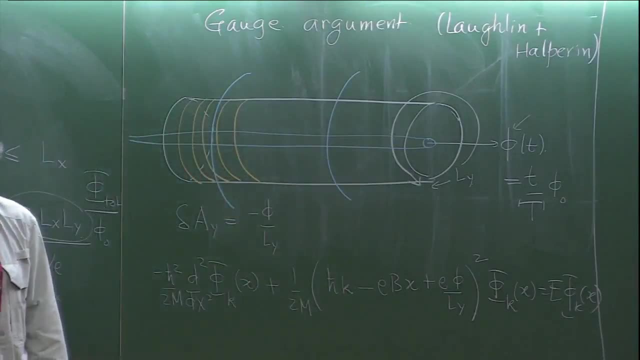 Okay, Because one guiding center has entered from this end of the disorder and one guy has left from that other end. Okay, So unless charge is accumulating inside here, the electron must have been transferred from one end to the other end. You guys get the argument. 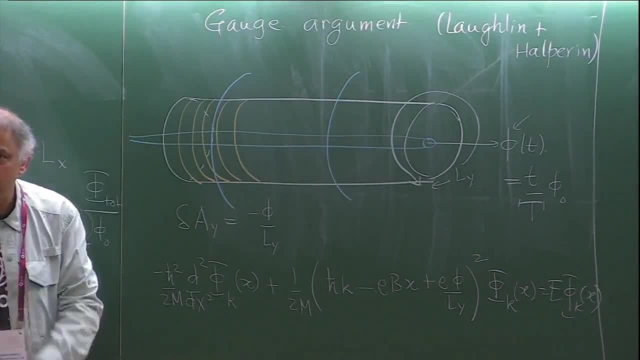 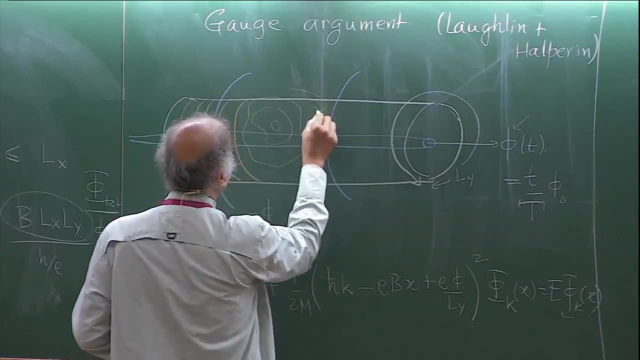 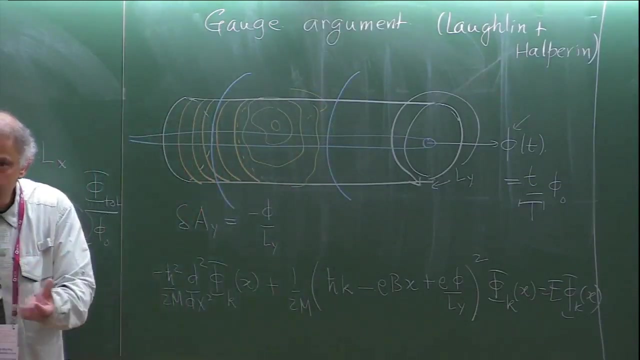 No, Let me repeat it. Okay, So in here there's some very scrambled looking. OK, it goes to the other side and so on. Okay, All these guys were degenerate. So whenever you have a set of degenerate states, 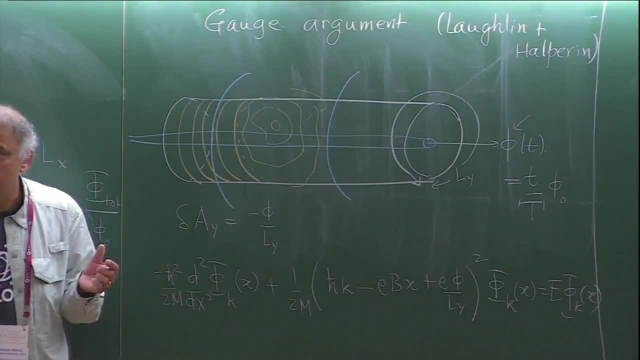 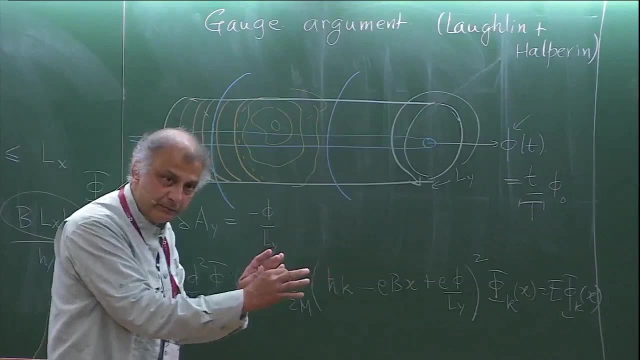 and you put any perturbation, everything gets completely scrambled up Because you have to diagonalize the perturbation right In the space of degenerate states. Okay, So they get scrambled up and there's a new set of eigenstates. 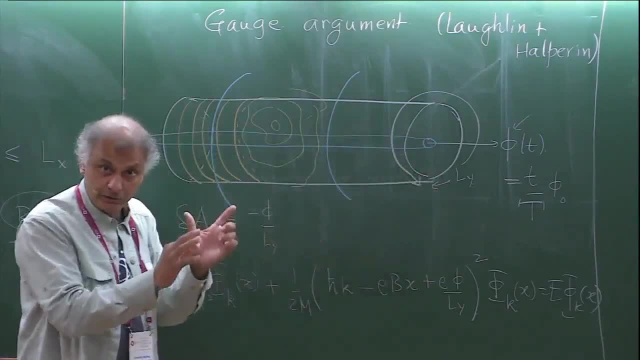 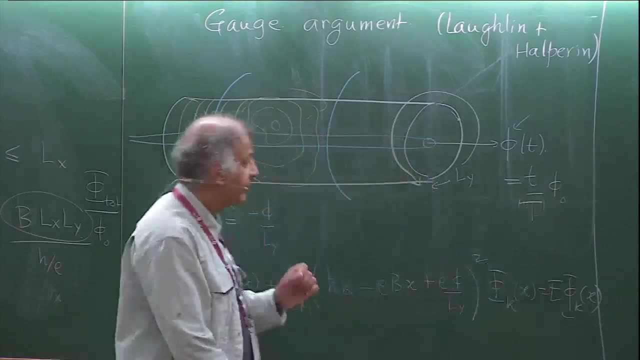 As I change the phi, this superpositions will all change, Right? But the key point is that when I take the superposition- and I take phi from 0 to phi 0, each of these guys has gone to the next one. 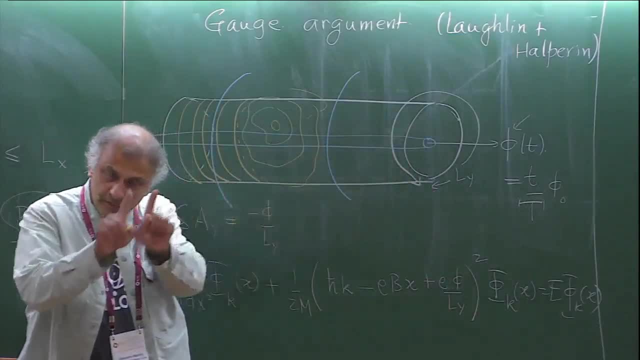 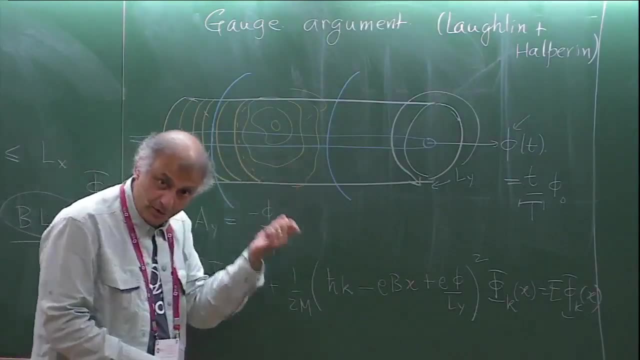 Right, So inside the superposition. so look at each individual guiding center in the superposition. Each of them has gone to the next one. Okay, So all the states that were occupied before are still occupied, But what has happened is that one guiding center